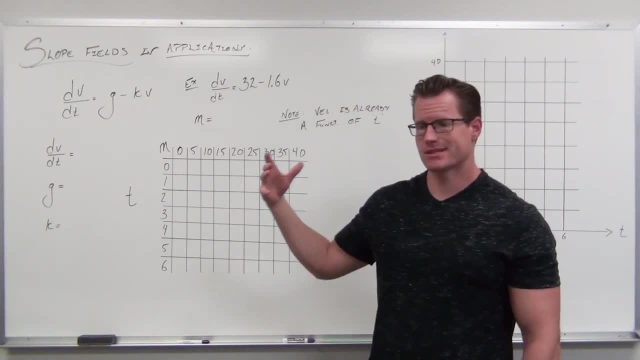 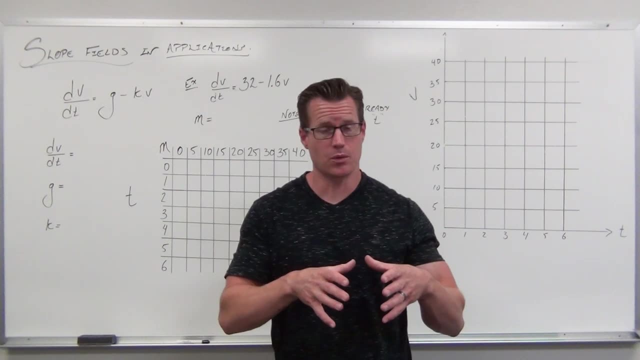 using differential equations. So again, let's start off with some sort of an application, Let's talk about slope fields and we'll get this picture of what's really going on with our situation. So a lot of times, in some of the simplified word problems you're used, 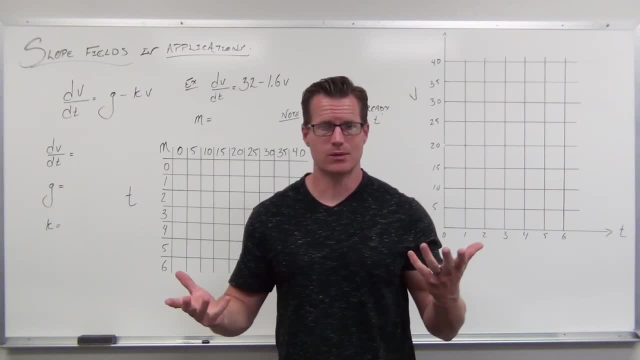 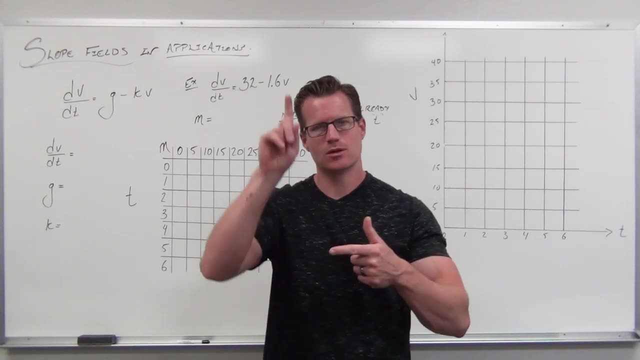 to. we neglect things like wind resistance, which isn't really realistic. If you jump out of, like, let's say, a helicopter, We're going to jump out of a helicopter, It's so cool, Don't jump up because it's spinning. But let's say you jump out of a helicopter. 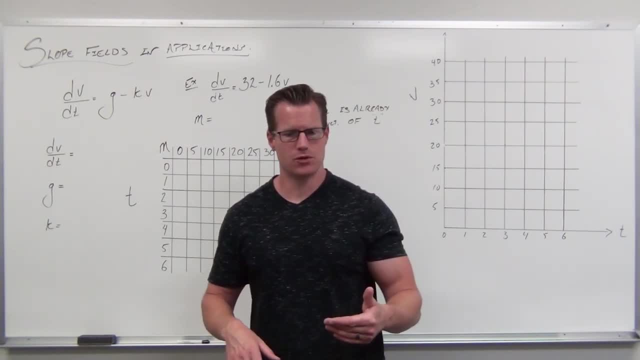 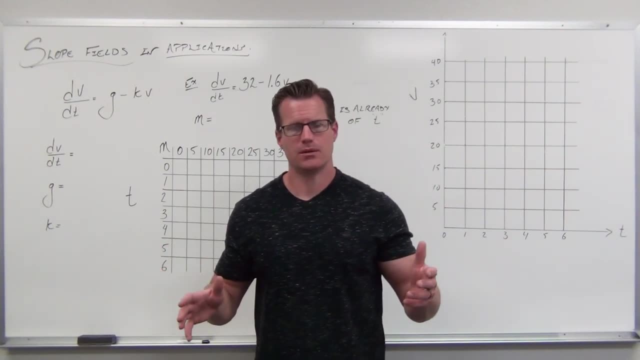 Well, you're going to fall. Now it makes sense that if you jump downward you're going to fall faster, And if you just kind of fall out you're going to fall, You're going to fall slower. But when you think about how wind resistance works, if 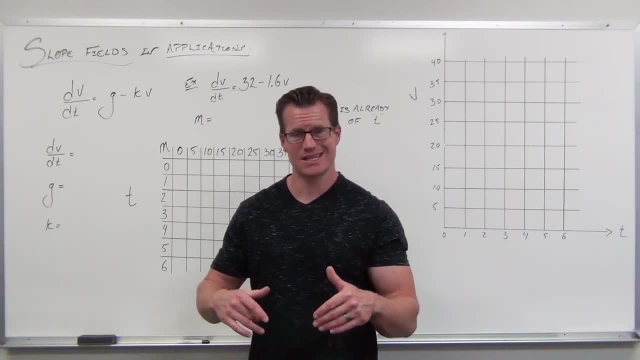 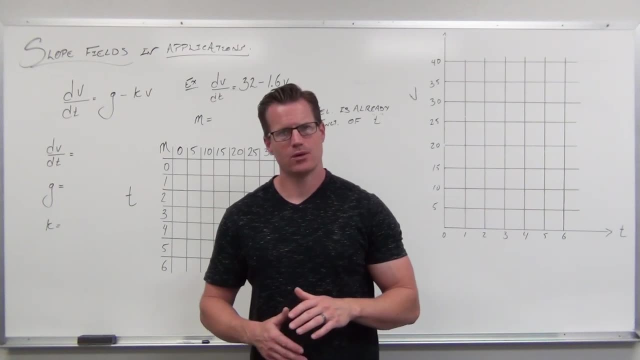 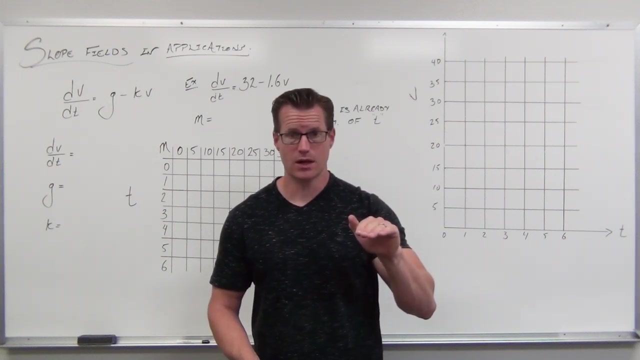 we just had gravity and no wind resistance, yeah, we'd pick up velocity until we smashed into the ground or pulled a parachute. But if we have wind resistance, as our gravity is pulling us down at a constant acceleration, our velocity is increasing, Yeah, but our 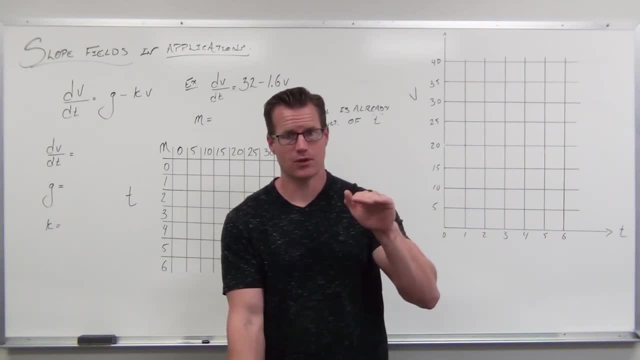 acceleration is not. We're falling down. Well, we're picking up velocity And as we pick up that velocity, we're going to fall And we're going to fall. And as we pick up that velocity, we're going to fall. And as we pick up that velocity, we're going to fall. And. 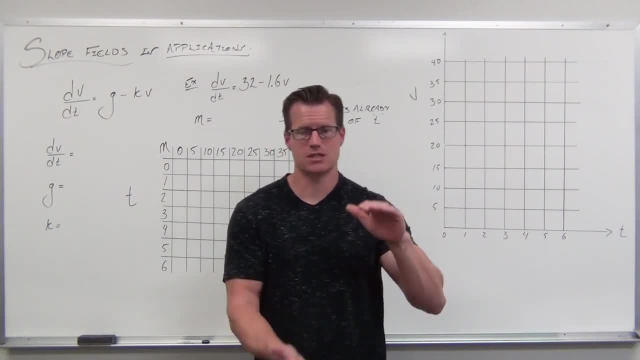 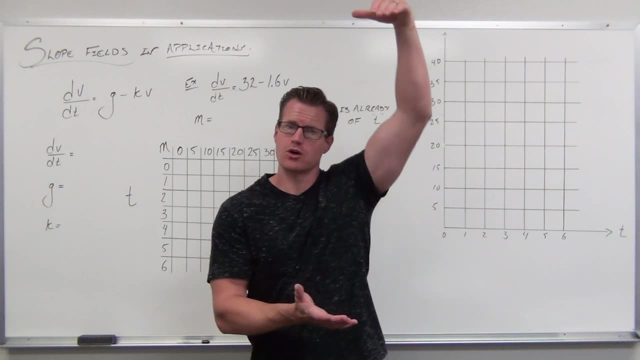 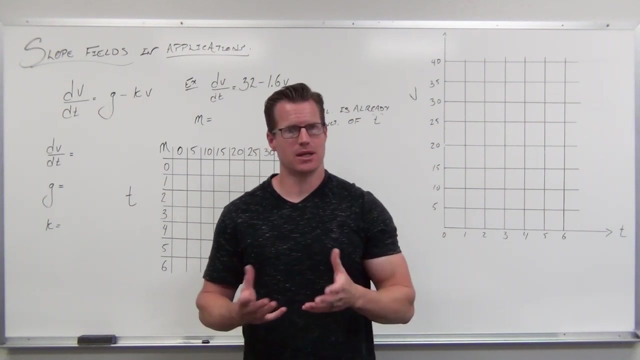 as we pick up that velocity we encounter more air resistance, wind resistance. We encounter this force upward of the wind, holding us up or pushing us up. So gravity is going this way, but the air resistance is actually a counterforce pushing us up And it depends. 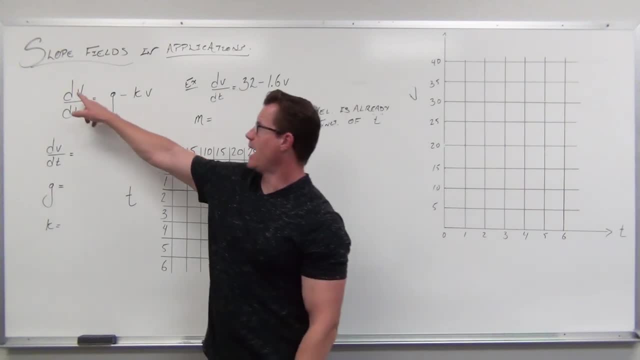 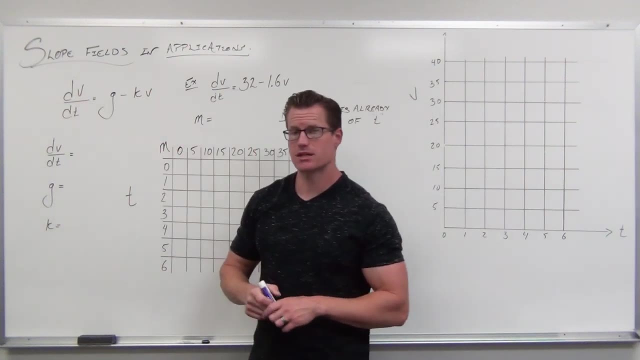 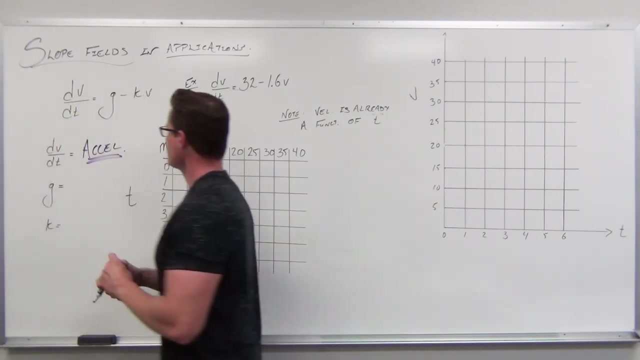 on your velocity. So, as it turns out, if we have how our velocity is changing, that's acceleration. Remember that the way that velocity is changing, the rate of change of our velocity with respect to time, that's acceleration. Well, in previous examples, like simplified versions, we would just do this And we go. 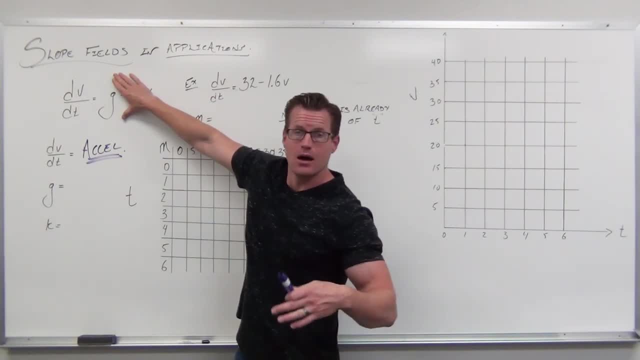 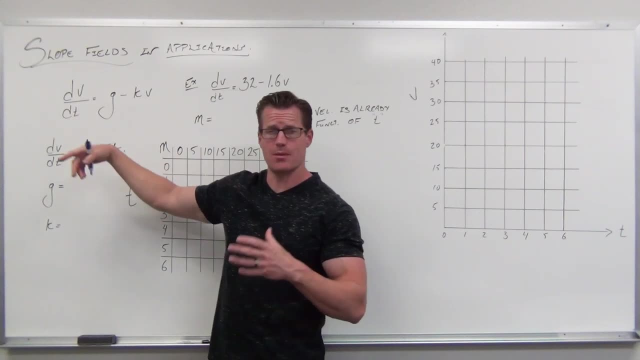 yeah, we're accelerating from gravity, Wind resistance, Nah, But we do have air resistance. So if we look at the way that velocity is changing with respect to time, our acceleration it is the acceleration to gravity minus, so that's downward, So acceleration to gravity. 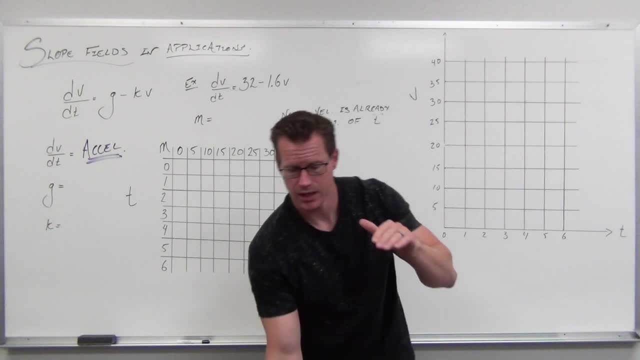 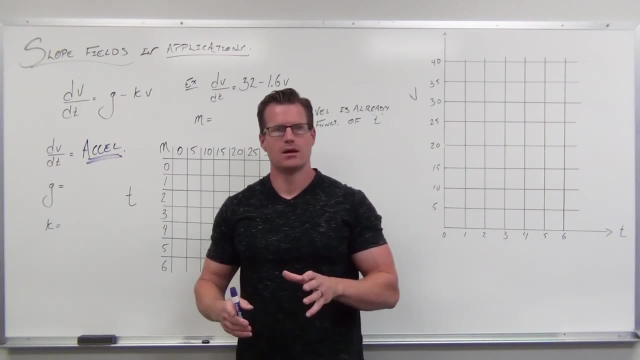 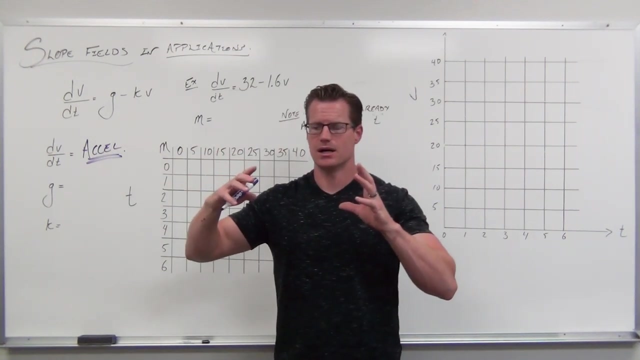 let's consider that gravity is is pulling us down. Air resistance is opposite of that. So our air resistance is some proportional constant like k, but it's proportional to our velocity. So the constant proportionality here is k. That's some sort of a number that's based on whatever the object is that's falling. 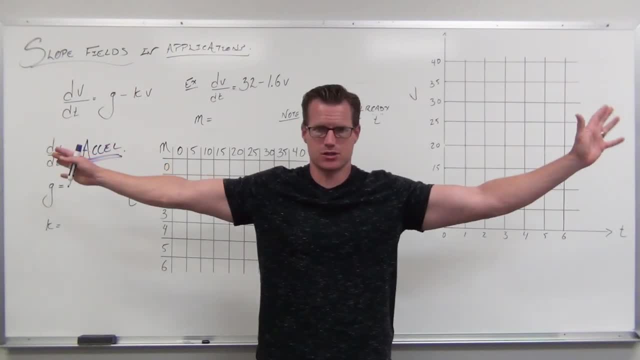 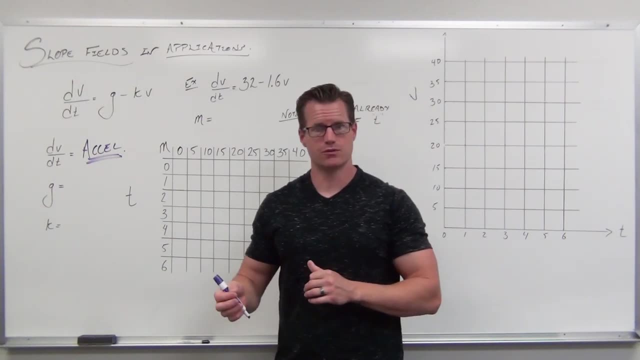 So we have a larger body or something would encounter more air resistance than like an arrow or a bullet or something, And but it is proportional to velocity. So if we look at our velocity, that's proportional to velocity. So the faster you are going, the more air. 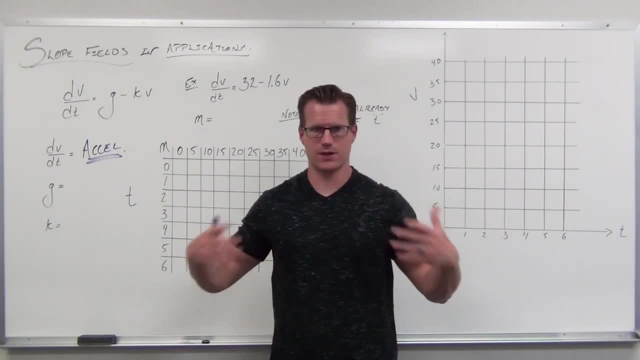 resistance you encounter. We know that right now because if we're standing still you're not feeling any resistance. but if you were running 20 miles an hour, that'd be really fast. You would feel a lot of wind against you. or if you stick your hand out of a moving 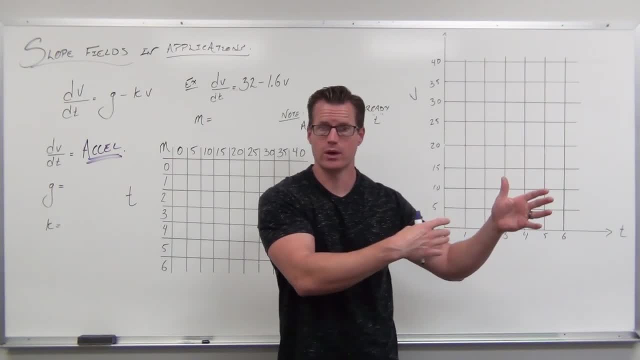 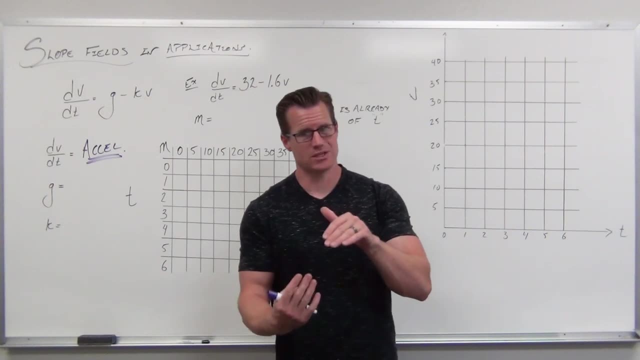 car, then you're going to feel that that wind against your hand, So the, and the faster you go, the more wind that you feel. Well, then that's pushing us upwards, That's a force that's acting upwards. So, in real life, our acceleration, the rate of change of velocity with respect to time, 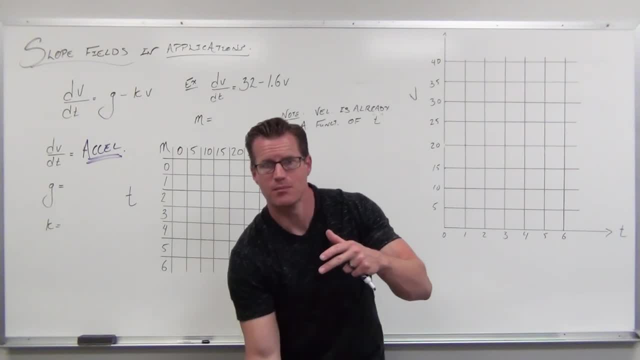 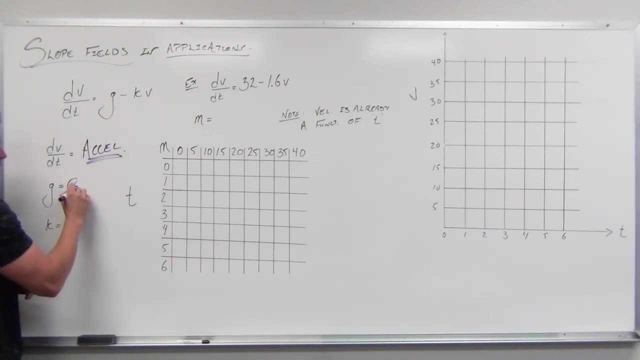 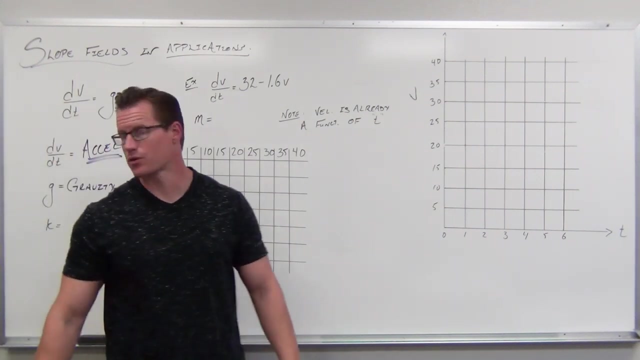 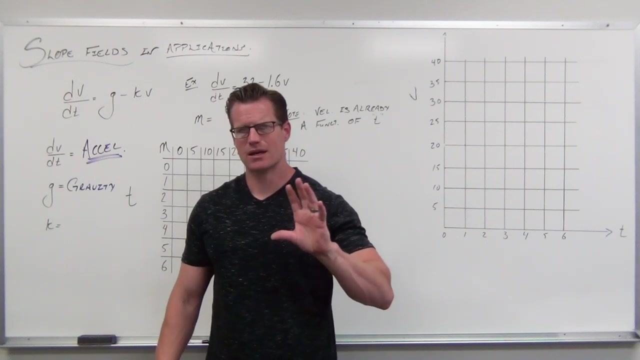 is, yes, gravitational constant, but minus the air resistance. I hope that makes sense to you. So G is that gravity, and it's the constant acceleration for a gravity. K is the, this, this idea of you: have a proportionality of air resistance. 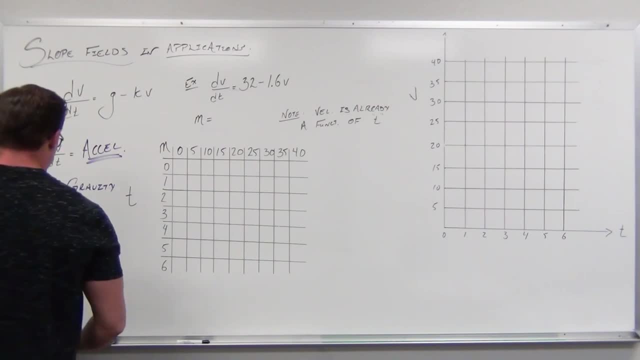 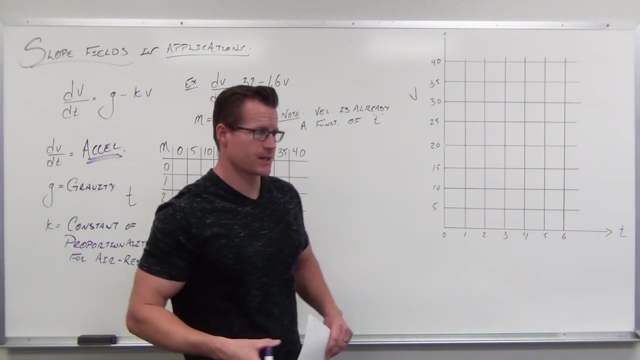 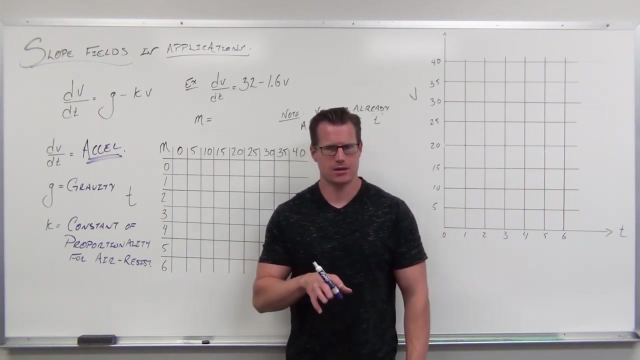 So how? that would be object specific. so whatever you are throwing out or dumping out or jumping out that that K is going to change. you know what object you are considering air resistance for. so here's the idea, and this is what I really want to get get out of this. if you just consider the gravitational acceleration. so 32 feet per second squared. and so every second that you're going, you're increasing the velocity of 32 feet per second. well, if you don't consider air resistance, yeah, we pick up velocity until we smash into the ground, but if we have air resistance, something pushing up against us at some point- 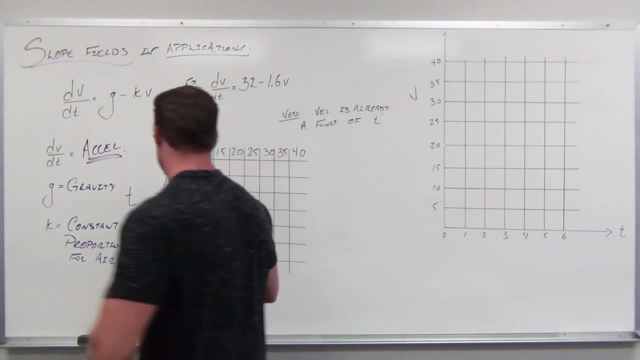 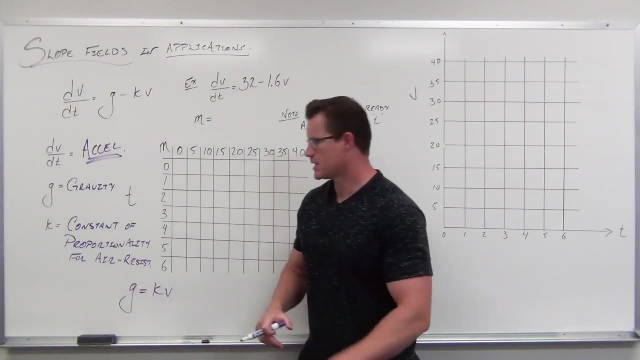 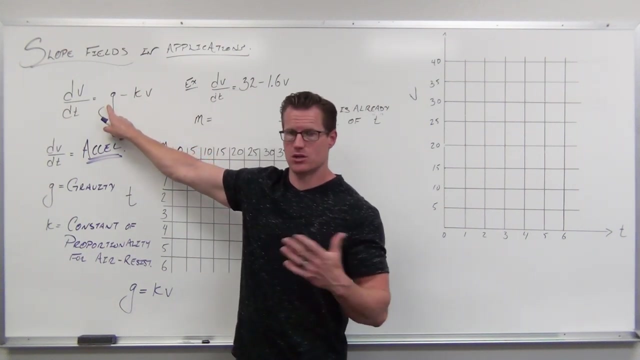 check this out at some point. G will equal K times V. somewhere along this line this is going to equal this. look, that's a constant that's not changing. we're on earth. it's always the same gravity. yeah, it does change as we get away from the 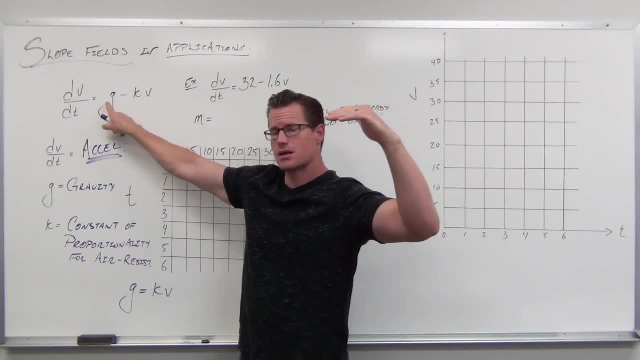 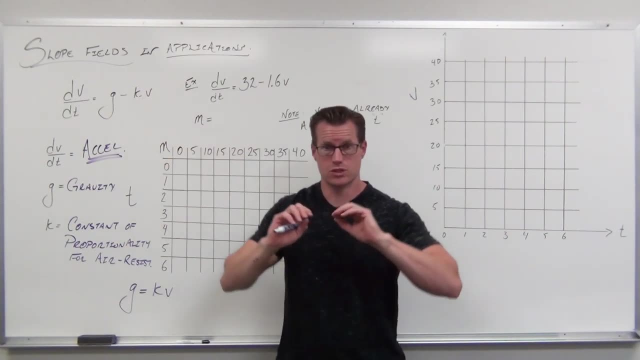 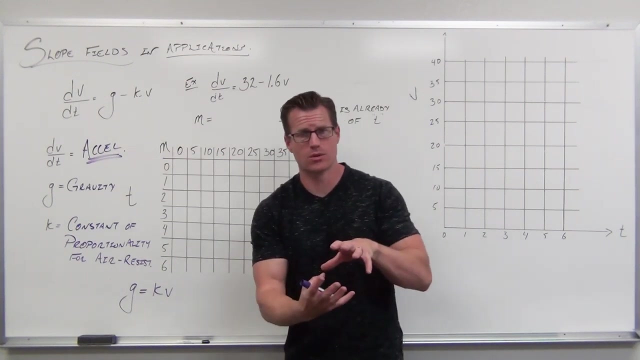 earth, but not, not by much. so that's constant. if that's a constant, and we hold that constant and this increases as velocity goes up. so so you dump something out of the helicopter, it's gonna pick up speed. as it picks up speed, it gets more and more and more air resistance against it. so the way our 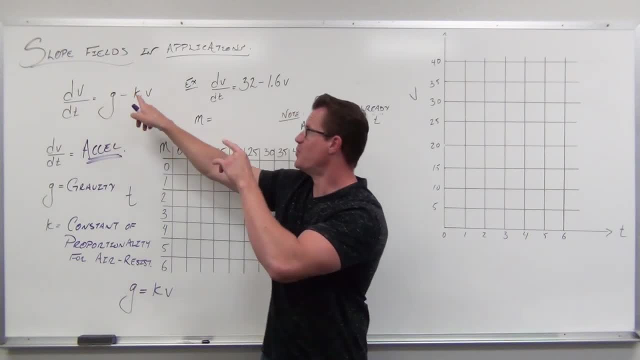 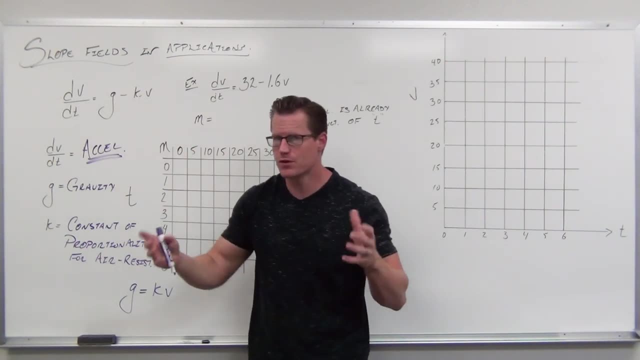 velocity is changing, our acceleration is constant, but this is growing as time goes on. that's growing. at some point, these two things will be equal. well, if you subtract two equal things, what do you get? well, you get zero. so, at some point, our acceleration, the way that- 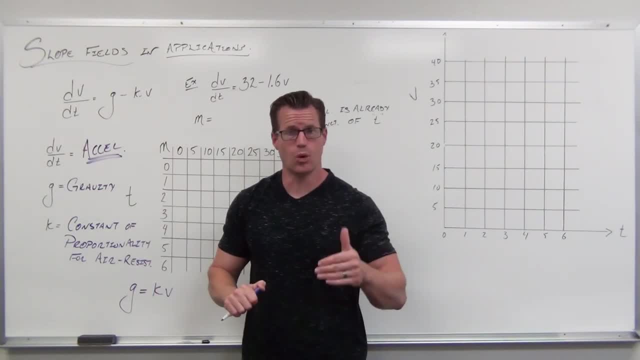 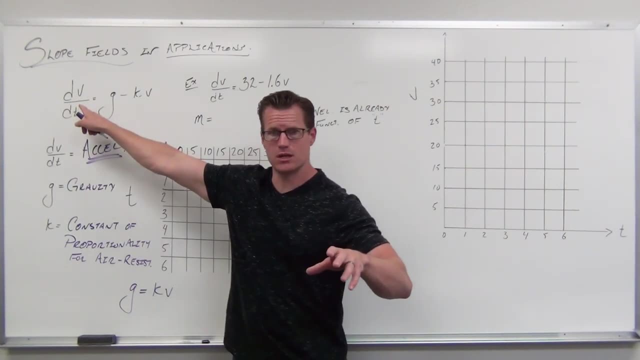 our velocities changing will be zero. it means our velocity won't be changing anymore. let me explain that one more time. so you throw something out, your velocity is going to change. that's acceleration, how your velocity is changing. so the rate of change of velocity with respect time your acceleration is. 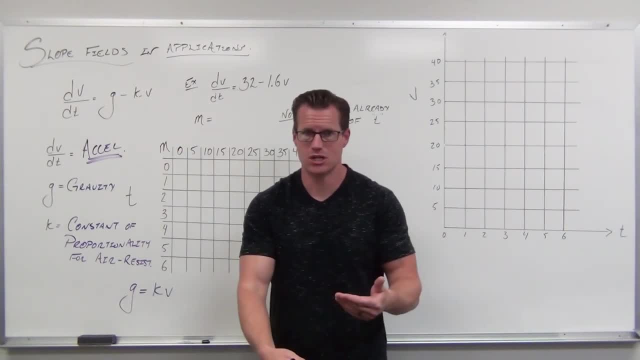 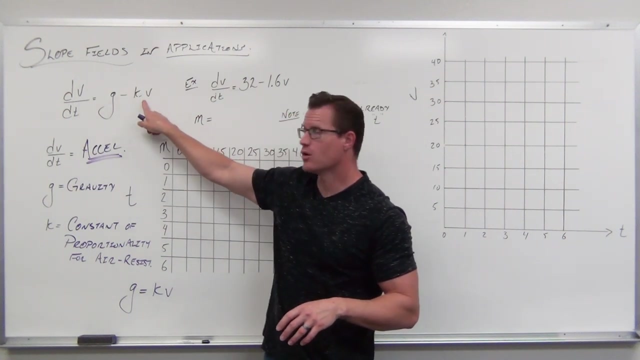 G minus air resistance. So right at the beginning you just have G, but your velocity starts going up, You're going to gain air resistance. So that's pushing against your acceleration, It's pushing against the body. It's going to slow your acceleration If that's constant and that's growing your 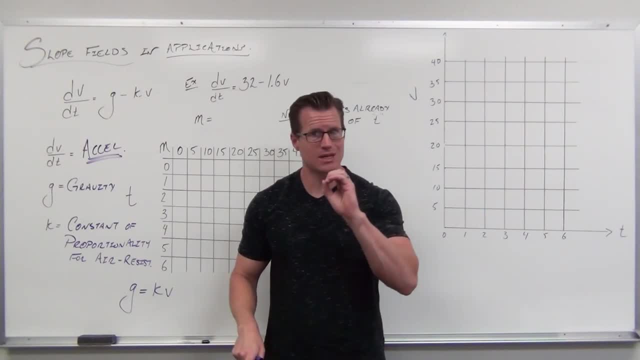 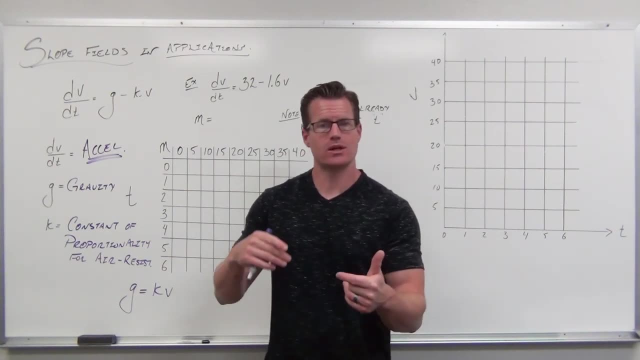 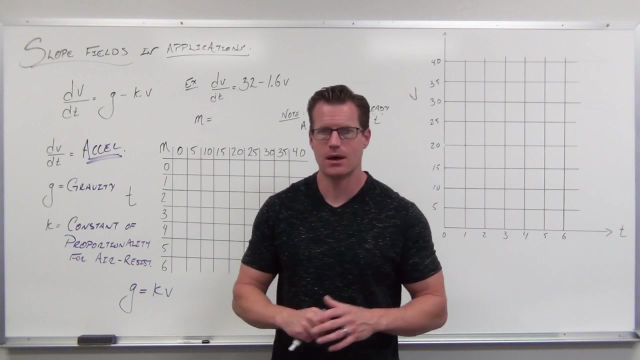 acceleration diminishes to the point where at some point you're getting zero acceleration. That doesn't mean your velocity is zero, That means that your velocity is not changing. So at some point you're going to hit a terminal velocity, or some people call that a limiting velocity for speed-related type. 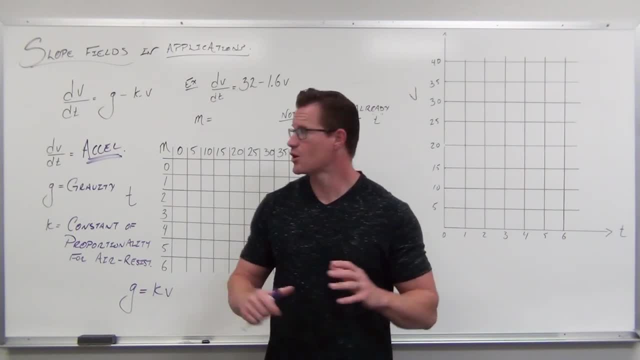 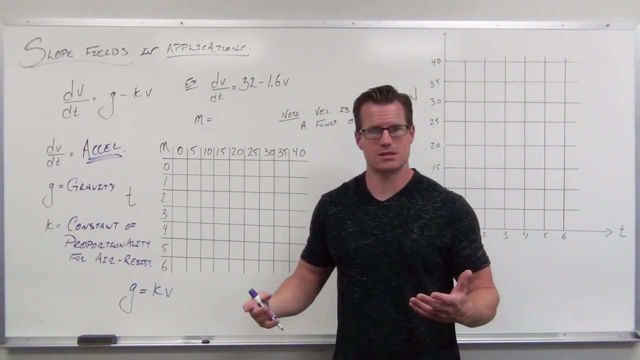 problems. We're going to hit that and we're going to see that in our slope field. So, without any specific techniques on how to solve these things, we can come up with a slope field to describe the situation. So one last time: Yeah, we're. 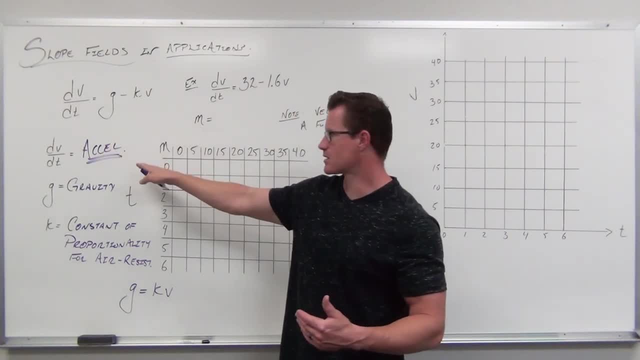 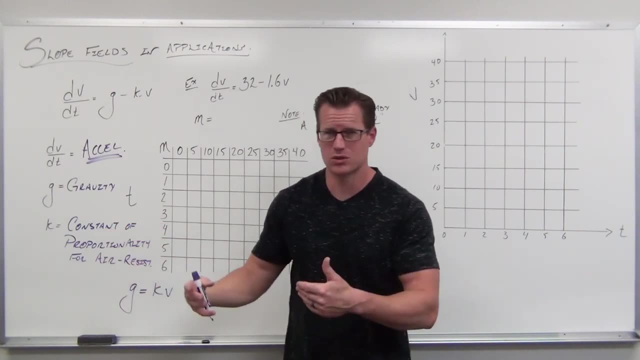 jumping out. Yes, the way velocity changes at specific times is called acceleration. Gravity is a constant, but the velocity changes at specific times. Gravity is a constant, but the velocity changes at specific times. Gravity is a constant, but the proportionality of your air resistance is proportional to well, your air. 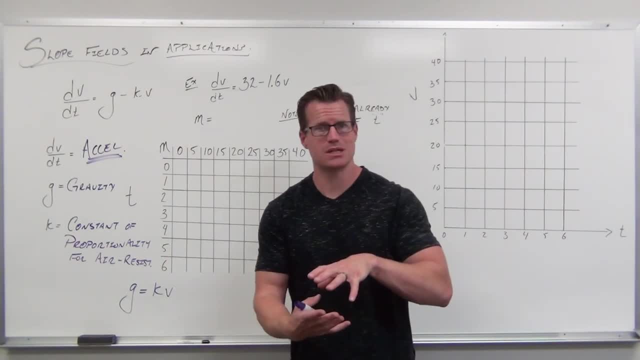 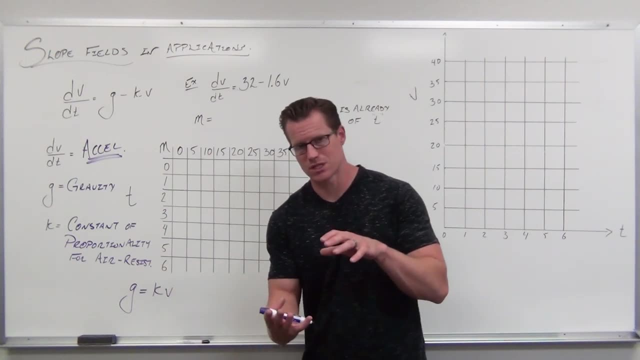 resistance is proportional to velocity. The faster you go, the more wind pushes against you. At some point you're going to reach this where the way that air resistance is forcing up is equal to how gravity is pulling down. That's going to be your limiting velocity. So when that happens, it's going to be: 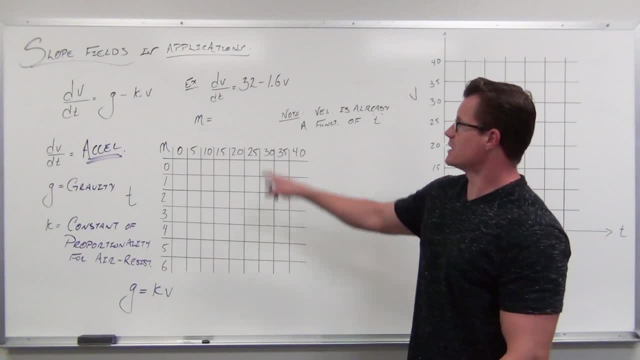 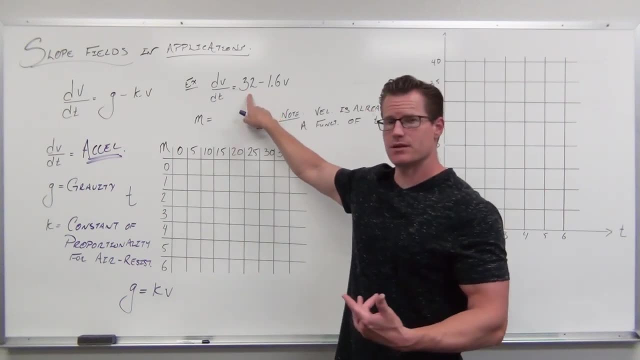 your limiting velocity and we're going to check that out. So let's say, let's explore one. So let's say that this is our situation: We're going to jump out of a helicopter and that, right there, that's gravity. That's 32 feet per second squared. 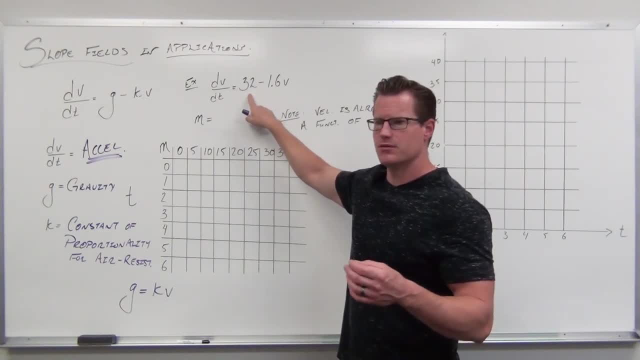 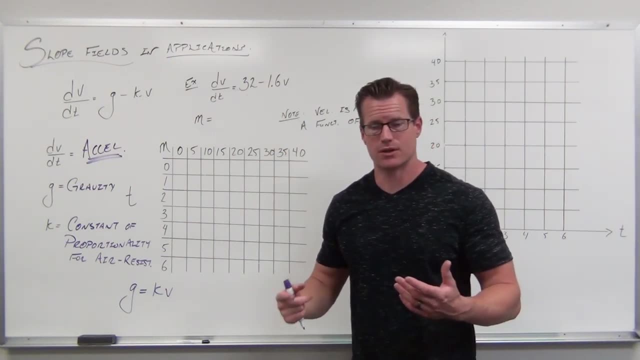 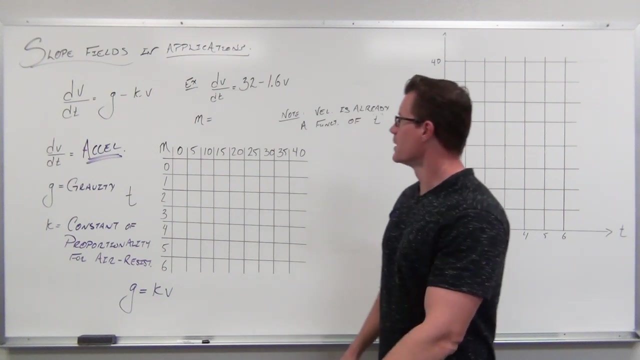 We have found somehow that the constant of variation, or how we're proportional, is this constant of 1.6 times. whatever velocity you're traveling, That's going to be how our wind resistance is affecting us. Let's say this is us jumping out. So if we have a first-order, 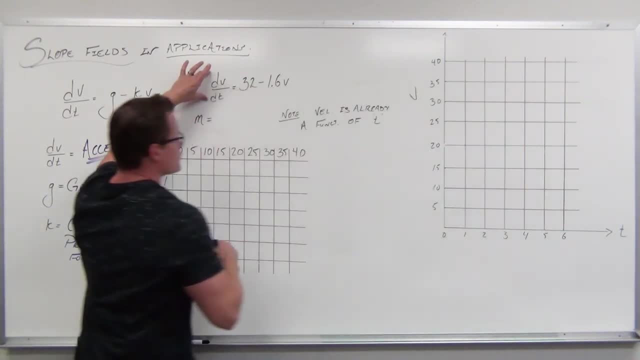 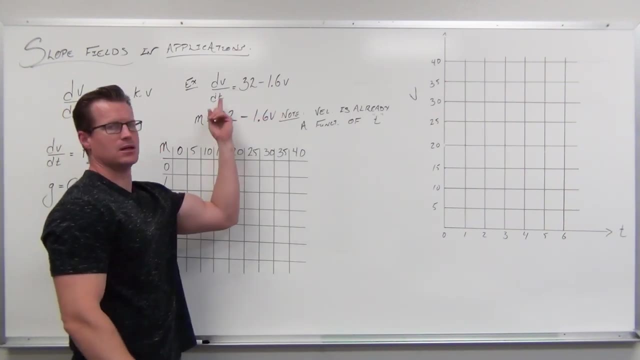 differential equation. we know that this means slope, So first derivatives mean slope. That means our slope is 32 minus 1.6 v. Well, where's the t? Remember that velocity is already a function of time, So velocity is changing. 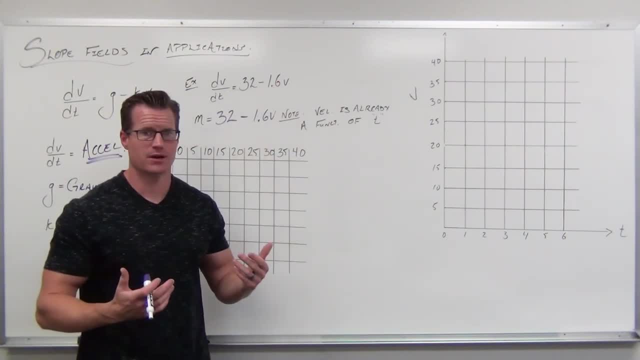 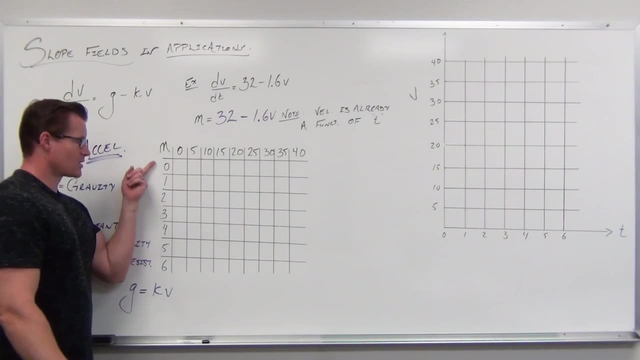 with respect to time, The t is wrapped up in that. That's our dependent variable, but t's in there somehow, So all we really need is velocity. What that means is: this is going to be weird, but as our time goes on, these numbers are not going. 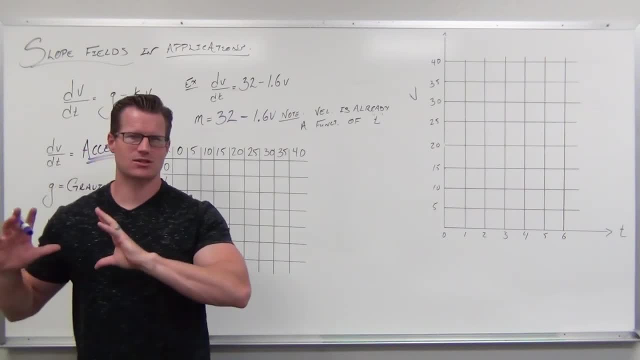 to change. There's no place in the world that we're going to be able to find the velocity, So the velocity is already a function of time. If we plug in the t, v already has all the t's in it, So all we've got to do is plug in zero. 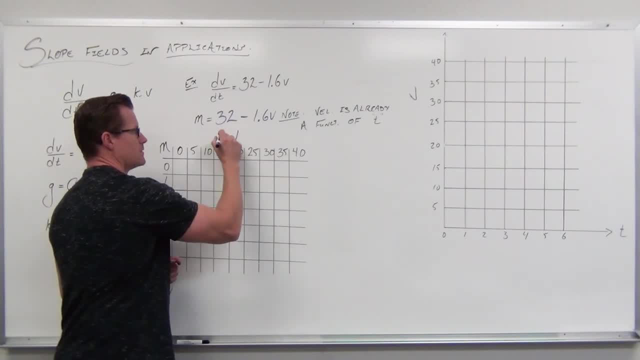 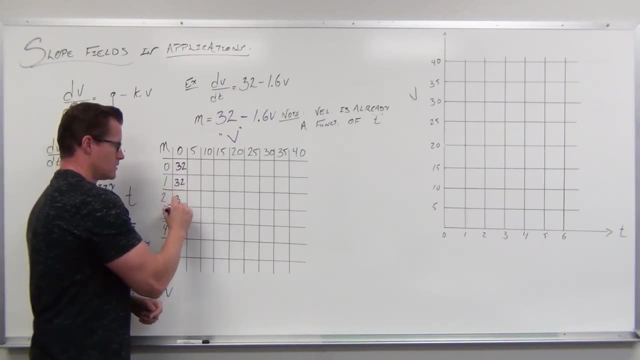 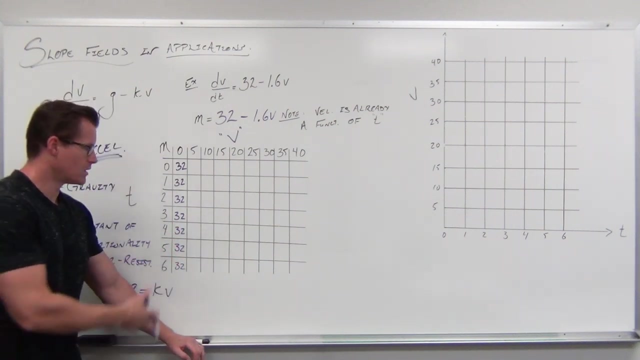 If we plug in zero for our v- and here's all of our t's- Plug in zero, you're going to get 32. And that's not going to change Our t. doesn't affect that. Our velocity is already 32.. 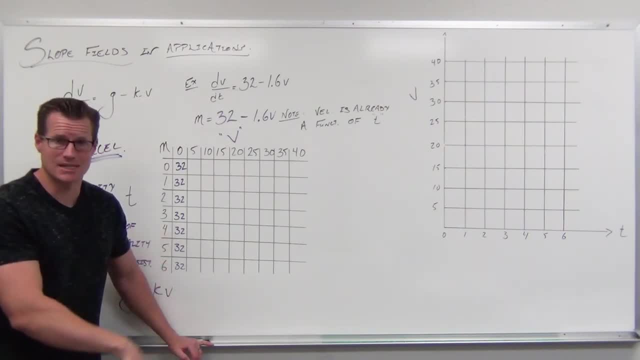 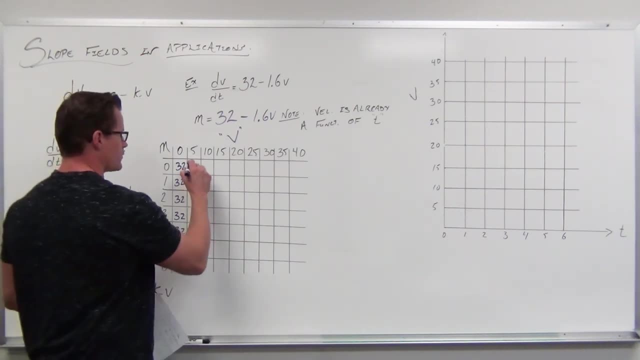 already has those. it's already a function of t. it already has those t's in it. It's not going to affect that. Plug in 5.. What do we get If we plug in 5, we get 24.. So 32 minus 1.6 times 5.. 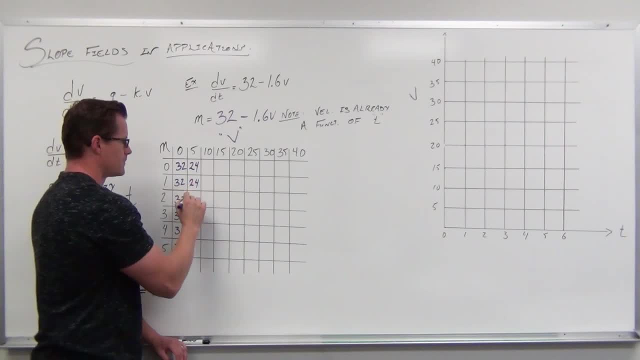 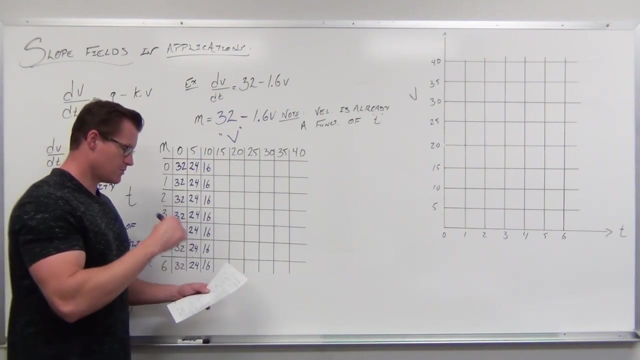 5. If we plug in 10,, well, that's 32 minus 16. So we're going to get 16 all the way down. If we plug in 15, 32 minus 1.6 times 15 gives us 8.. 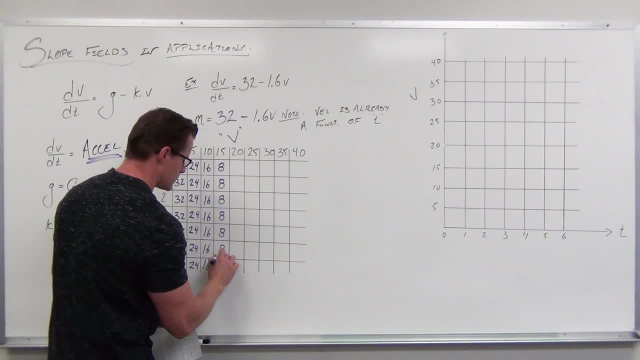 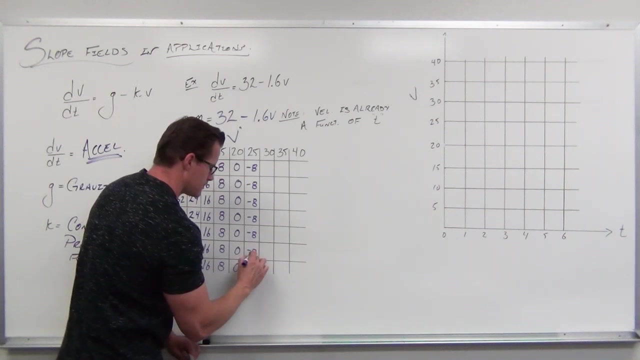 And if we plug in 20, we're going to get 0.. This is what you're looking for And if you continue this, this is negative 8 and negative 16.. You know, if you were watching for the slope field video, the one right before this, we 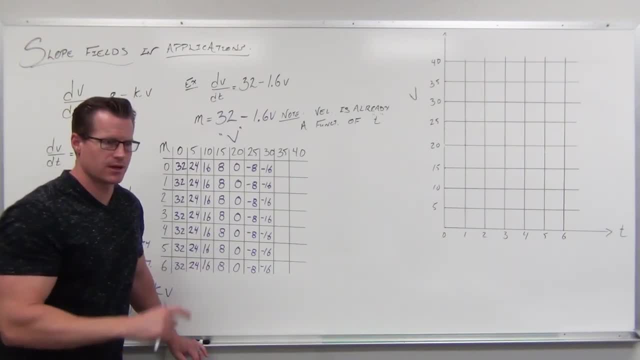 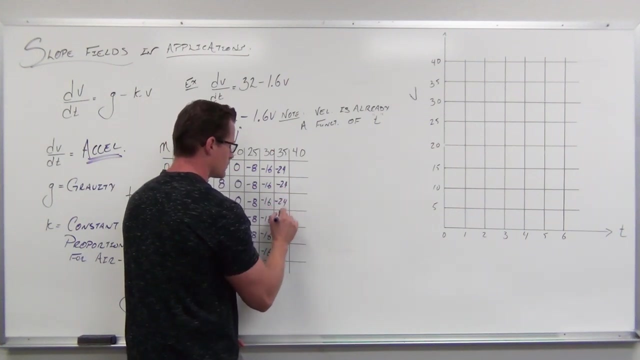 had diagonals that weren't changing. That happens a lot when you have like x's plus or minus y's- This when your time is not even available Very long, here you're going to get these verticals that aren't changing happens. 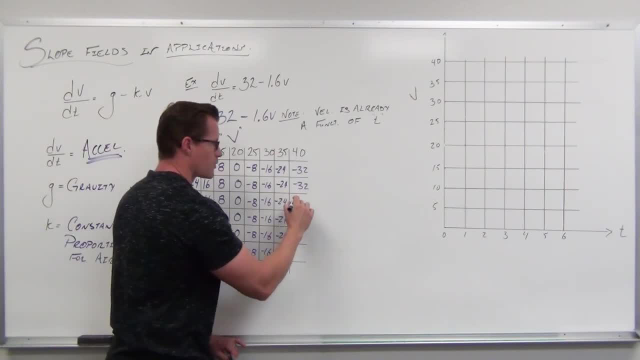 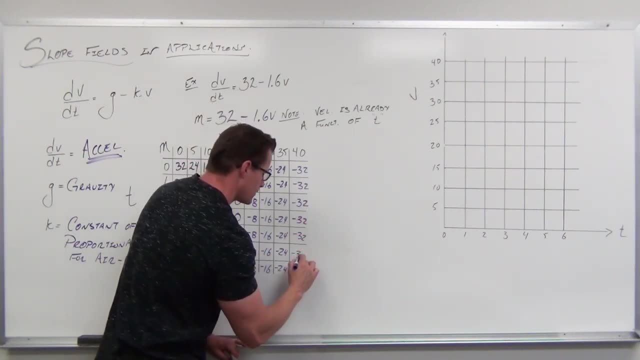 And I know that you can plug in 40 and do 30 minus 1.6 times 40 and get these same exact numbers I'm getting All right. So let's make all this make sense before we do our slope field and look at what's going. 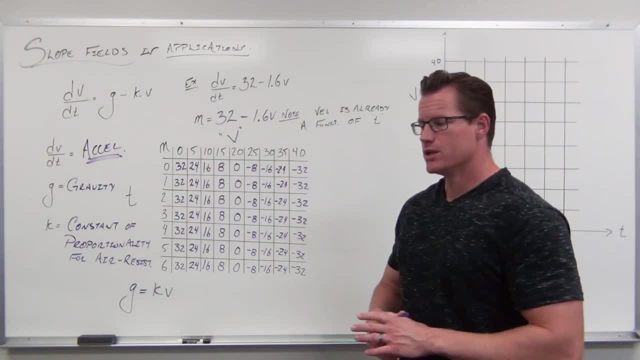 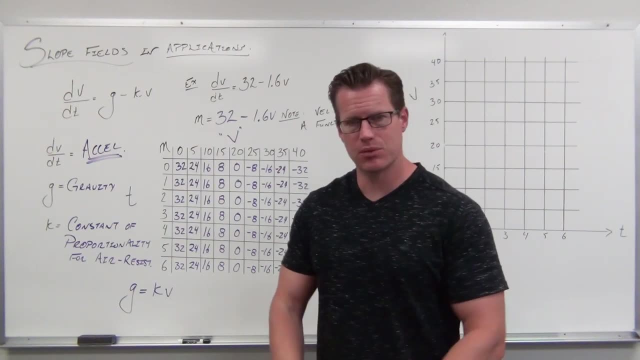 to happen on our graph. So we know that in real life we get air resistance. That means that when you jump out you're going to reach some sort of limiting velocity. At some point your air resistance is going to meet up with acceleration to gravity if 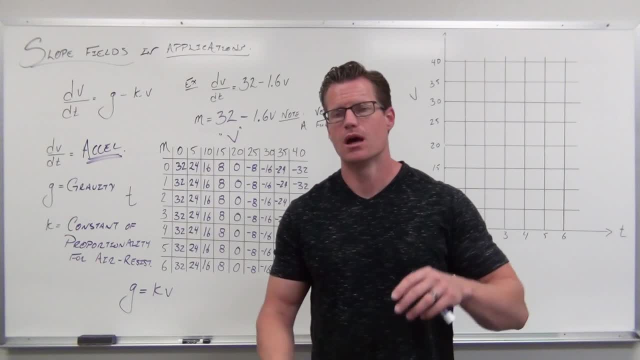 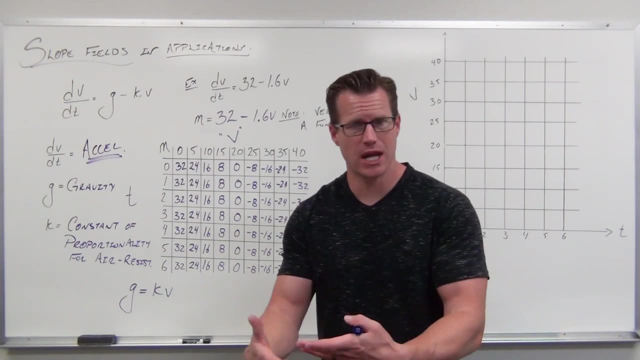 you're jumping high enough and don't hit the ground first or pull a parachute or something, They're going to be equal. That means that you're not going to be changing your velocity after that. Zero change, A zero acceleration means that you have a constant velocity at that point. 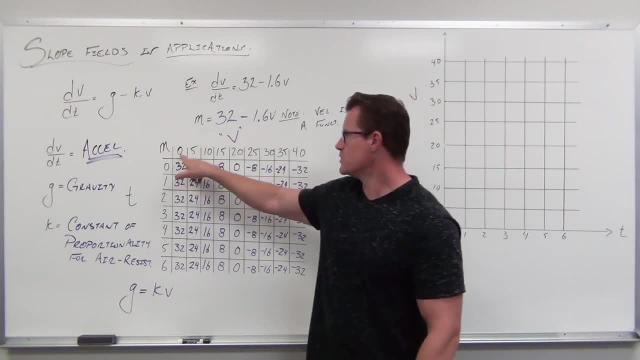 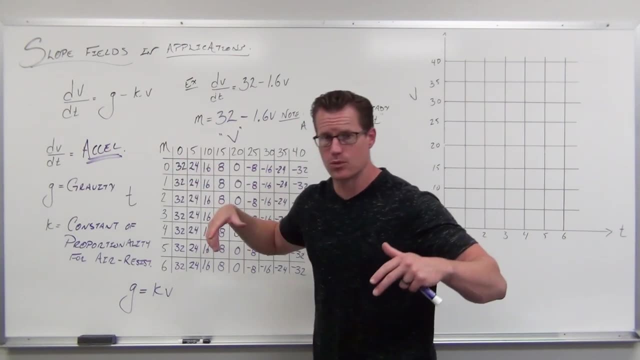 So this is what that does. This says: if you jump out, you just fall, So your initial velocity is zero. You're not jumping downwards, You're in a helicopter, right, So you're probably not going to jump up because there's a blade. 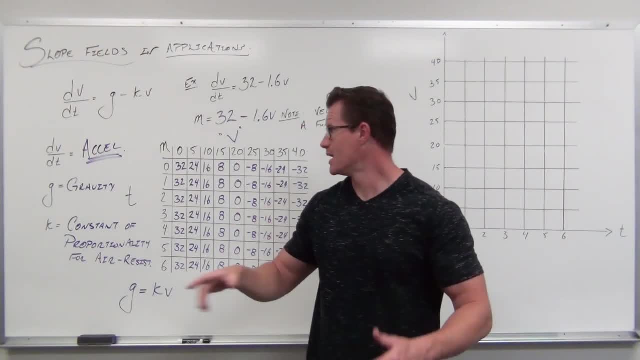 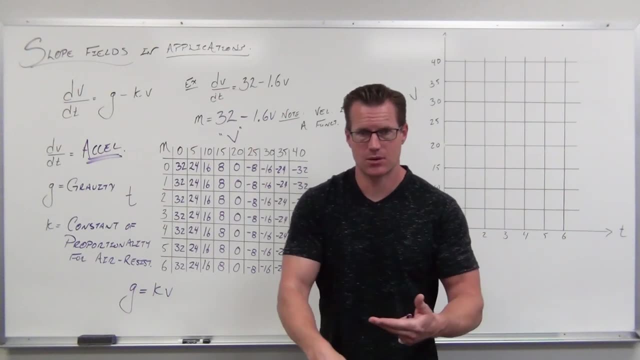 That would be a negative initial velocity. So if you jumped out and went negative five, You're going to probably hit the propeller. You don't want to do that, So this would be jumping downward. So if we jump out at zero, so just fall. 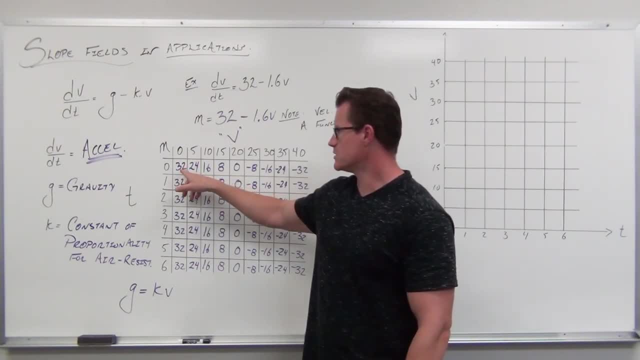 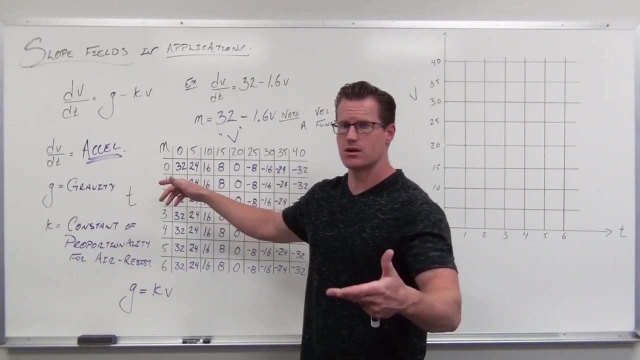 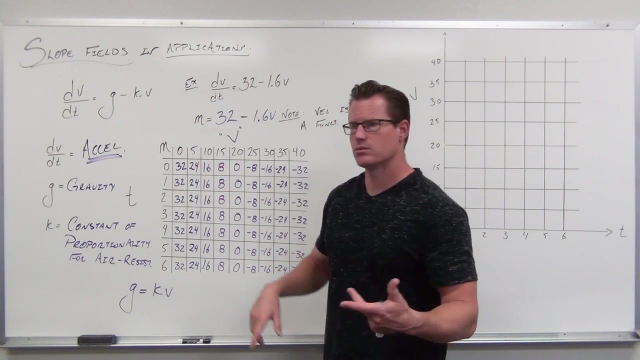 Well, initially we're going to be going this 32,. well, let me say this differently. We'll see this on our picture. We're going to be increasing our velocity at this 32 feet per second If we jump out at five. 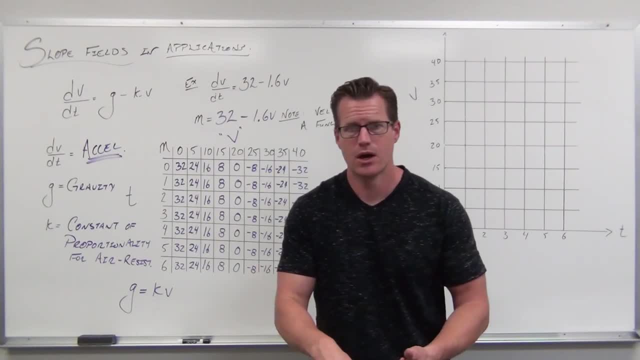 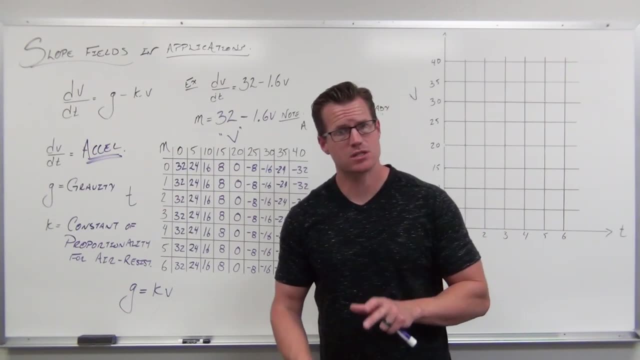 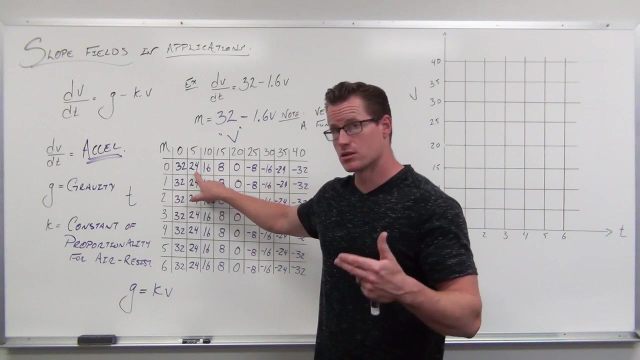 Does it make sense? If you jump out going downward, you're going to immediately encounter air resistance immediately. That means that your rate of change of velocity is going to be slower. You've already jumped out at five feet per second, So the rate at which you're changing is a little bit slower. Now let's say you jump out at 10.. You're jumping downward at 10 feet per second already. The rate of change is going to be slower. You've encountered that air resistance immediately Here. you didn't. That's why we're accelerating. 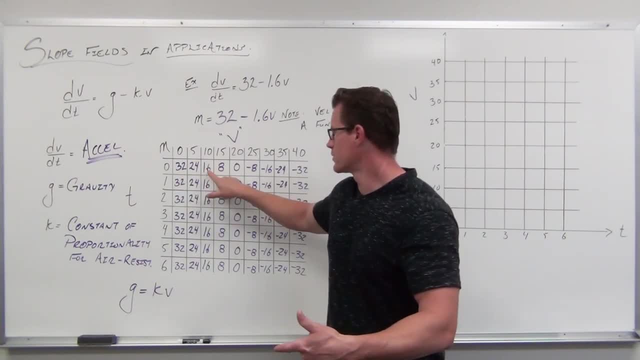 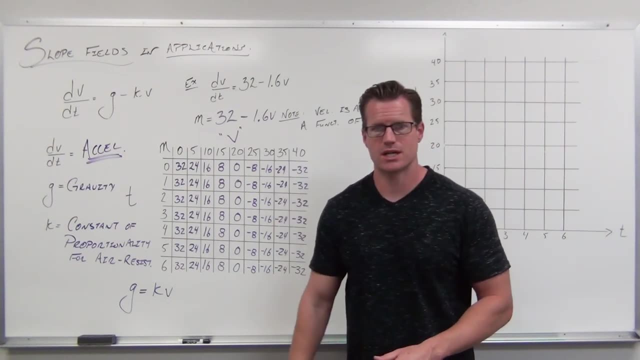 Oh, that's why our velocity is changing faster. That's why we're accelerating Here, no, Here, no, Here, a little bit, A little bit slower. Now, what about 20? At 20, if you jump downward at 20 feet per second right from the get-go out of this helicopter? 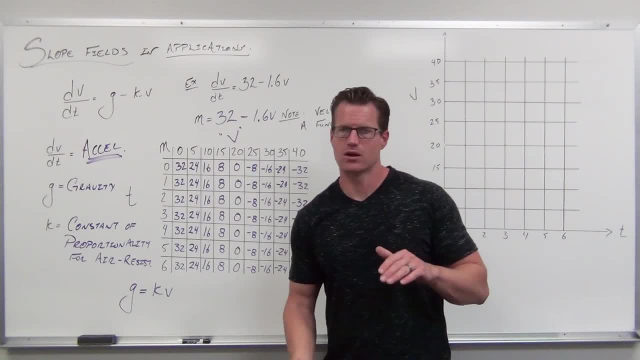 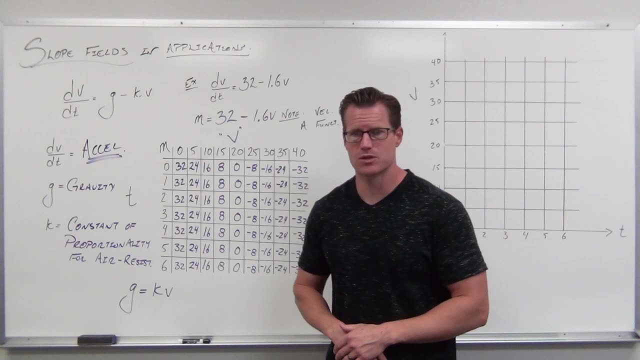 your rate of change isn't going to be anything at all. You've encountered just enough air resistance to meet up with your gravity. So this is weird and we're going to see it on the picture. but if you jumped out of this helicopter at 20 feet per second, you're not going to feel your velocity increase or decrease. 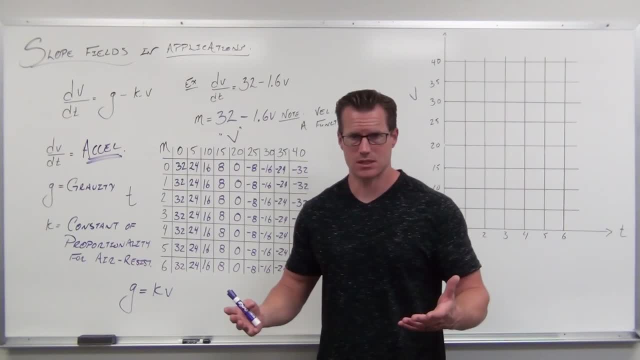 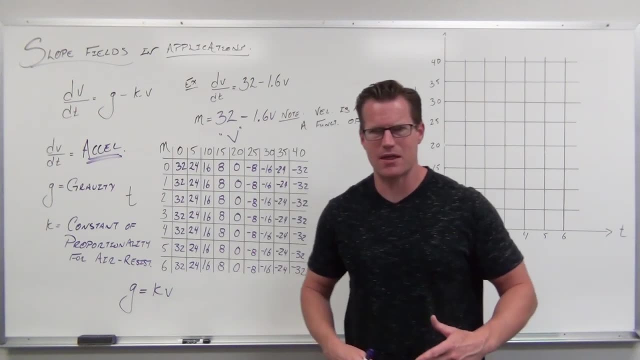 You will have immediately met your limiting velocity. Okay, That's wild. Now let's say that you jump out faster than that. Let's say that you jump down. Wow, I just really want to get out of that helicopter. And you're jumping down at 25 feet per second. 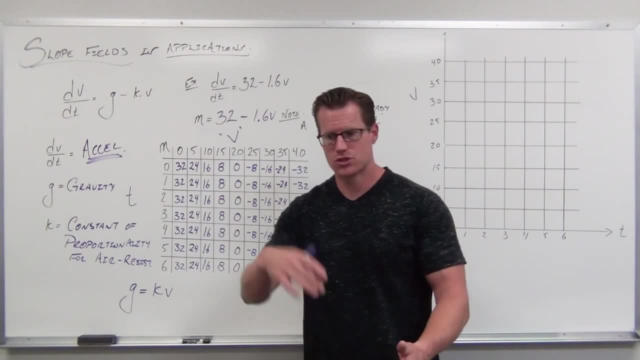 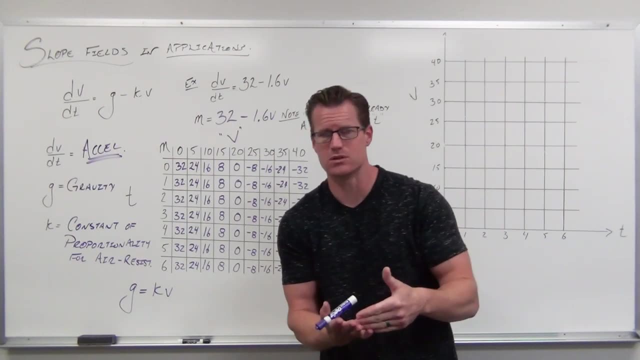 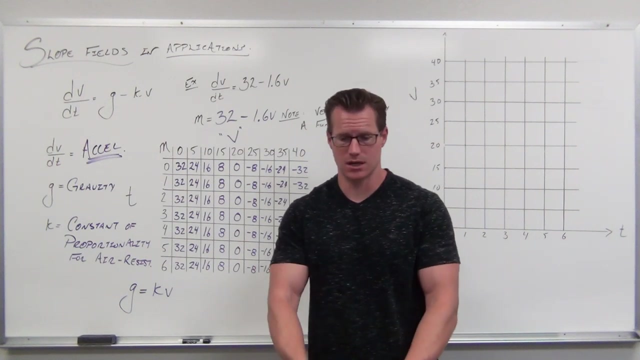 You're actually going to slow down. So if you're jumping faster than your limiting velocity, air resistance is pushing up more than gravity is pulling you down. You're going to slow down. That's the same principle like when you shoot: if you shot a gun downward, So at some point your gun's going so fast that it's meeting so much air resistance that gravity's not going to overcome that. Your air resistance is pushing up more than gravity's pulling that down. You have initial velocity there that's so fast that it's encountering so much air resistance. 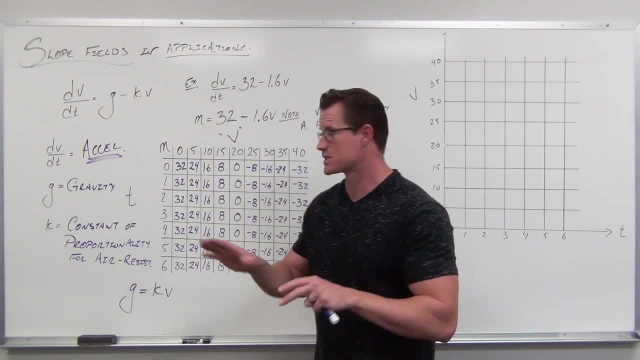 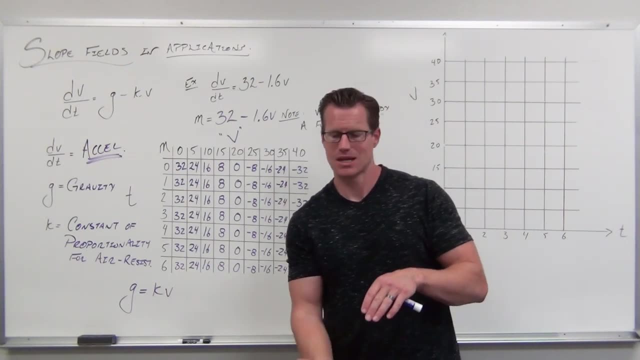 it's going to slow that bullet down even though you're shooting downward. That's what's happening here. So if you jumped out at 40 feet per second downwards and really pushing it, you're going to encounter so much air resistance that that's pushing you up more than the gravity is pulling. 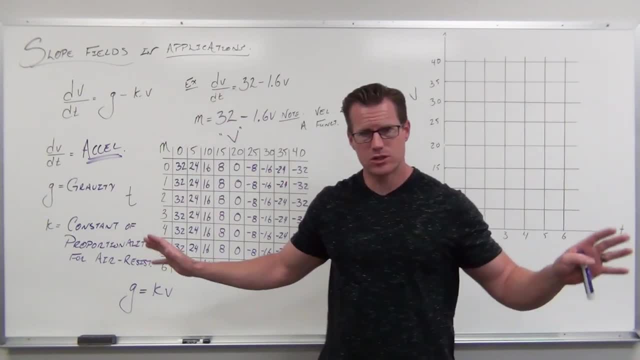 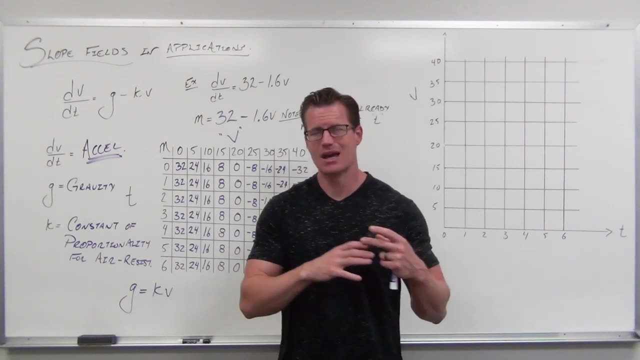 you down. That's weird, but that's what this is going to play out as So long story made real short. we have air resistance. It's proportional to your velocity and we can show the picture of it really kind of nicely. 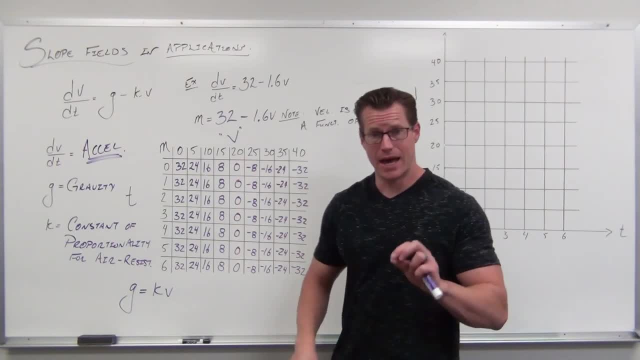 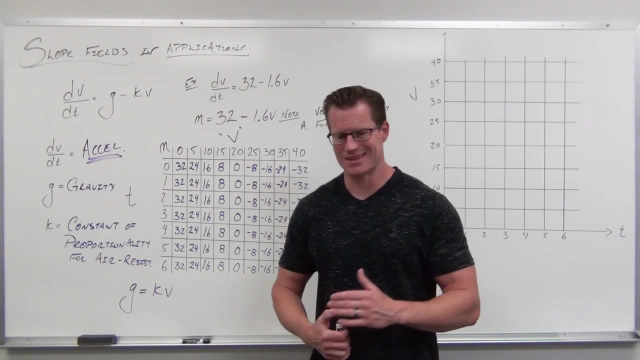 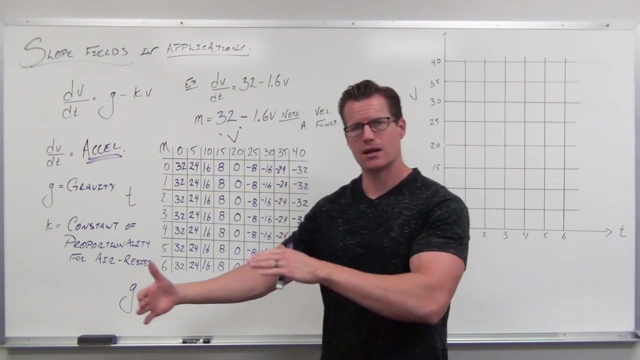 This point where we have a zero change, that is called your limiting velocity or terminal velocity, Or when we talk about population, we'll get like this population limiting factor, like a carrying capacity, something that limits how much we can grow. If you're below that, you're going to increase. 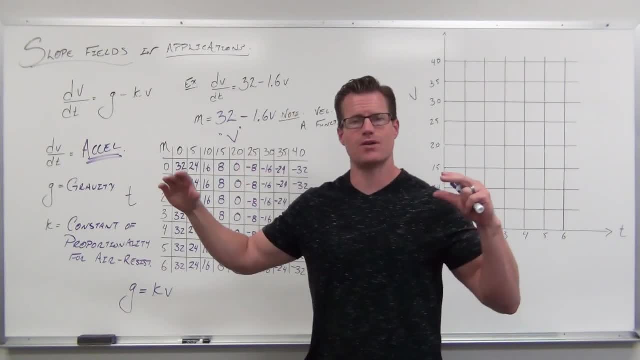 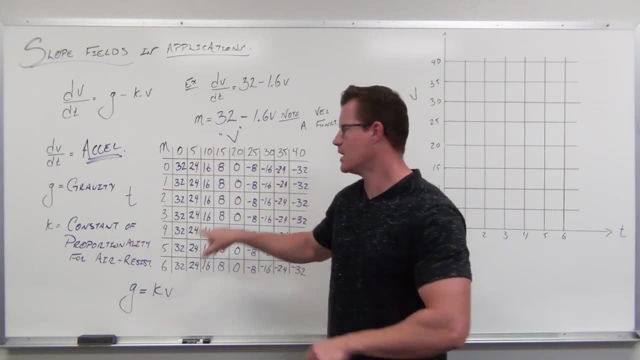 You're going to increase. If you're above that, you're going to decrease until you find this leveling spot, this limit. So let's put these slopes- Remember these are all slopes. How our velocity is changing is right here. Let's put them on our graph. 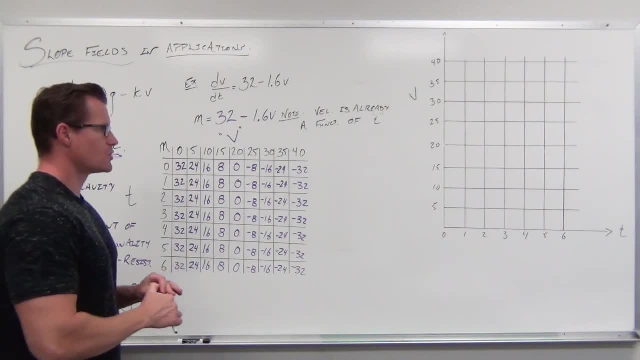 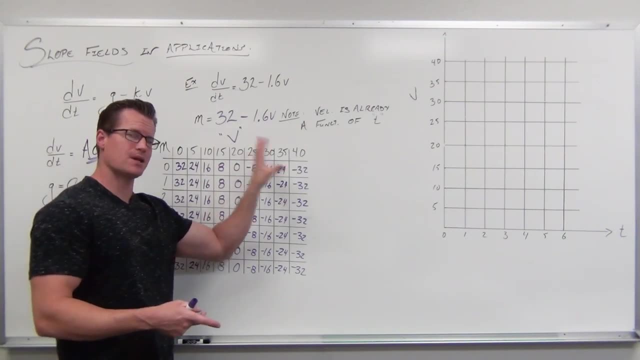 Let's see what happens Again. we made the grid. It's a lot easier to use. So, because our time isn't affecting- well, our time is affecting our velocity, but it's wrapped up in the velocity itself. So, for time zero, one, two, three, four, we're going to have these. 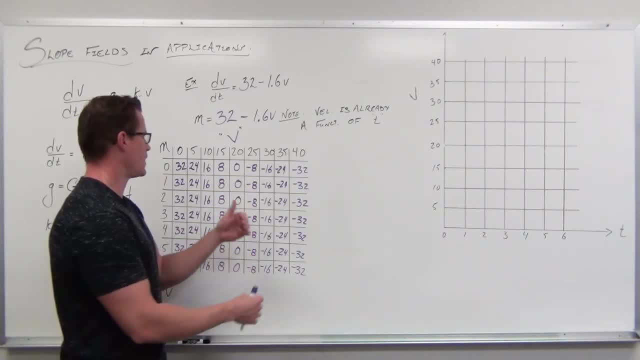 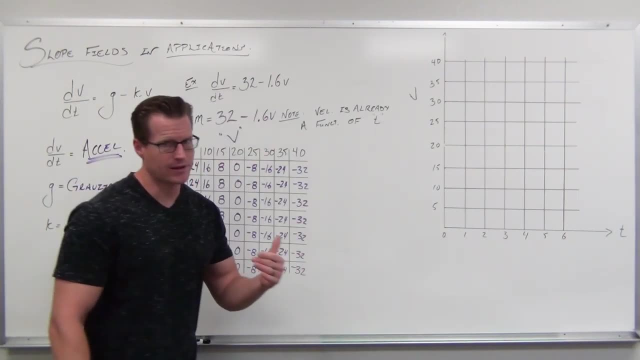 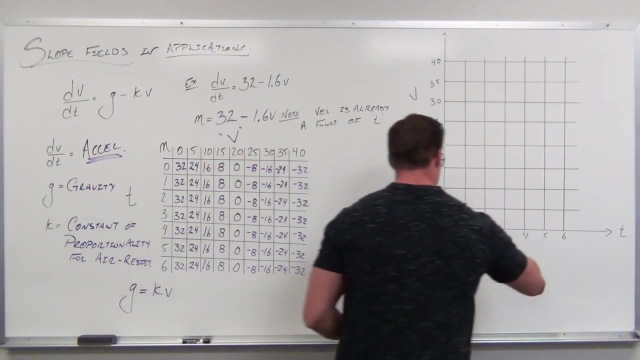 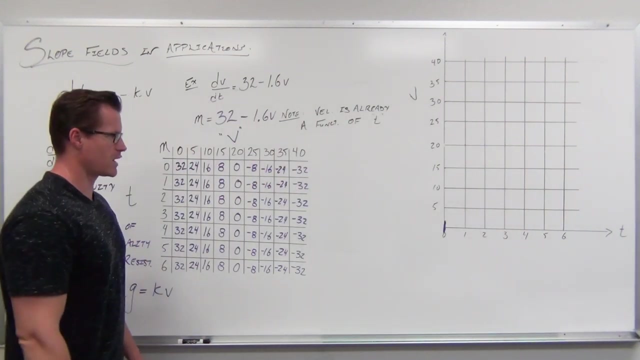 These intersections of time and velocity. So zero, zero. right down here we have a slope of 32.. That's really steep. I'm not going to really be able to draw that as not a vertical line. That's going to be darn near a vertical line. 32, rise or run. 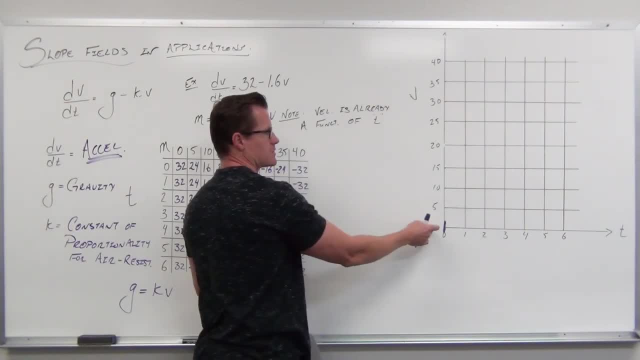 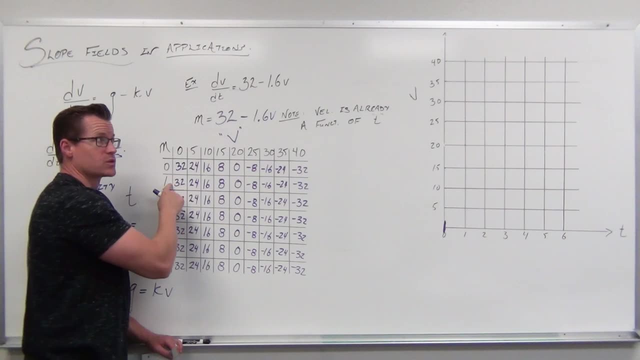 But also at. So here's our velocity. So zero, five, 10,, 15,, 20,. here's our times: one, three, six. So at zero zero, we got 32.. At, t equals one and velocity zero, we also have 32.. 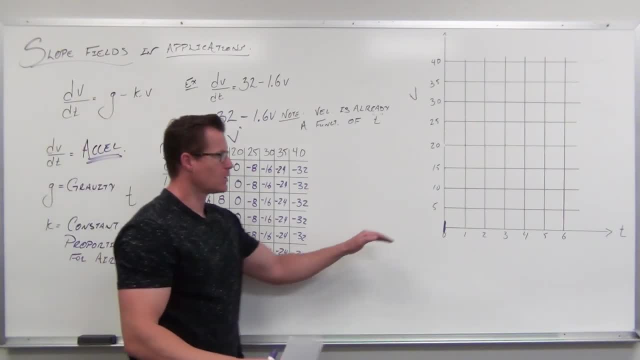 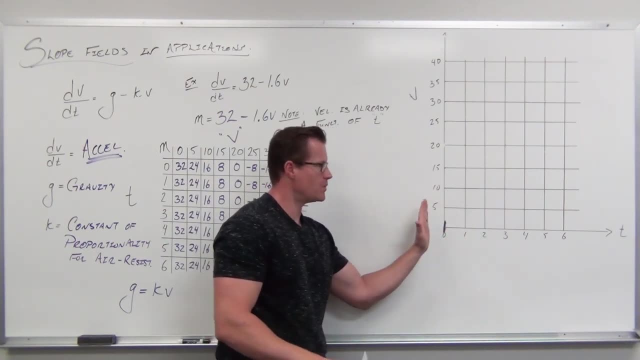 At. t equals two and velocity zero, we got 32.. So all along this velocity of zero, we have a slope of 32.. This is acts like a diagonal. I know it's not diagonal, but this does not change. All right. 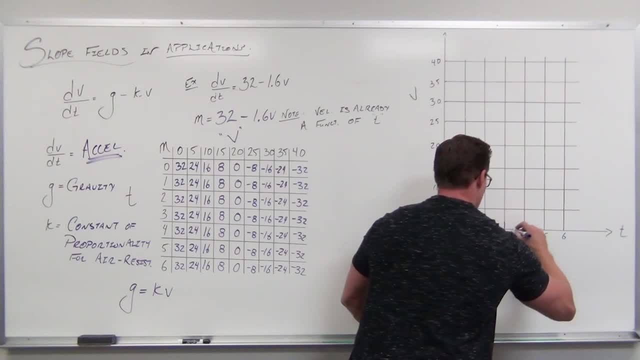 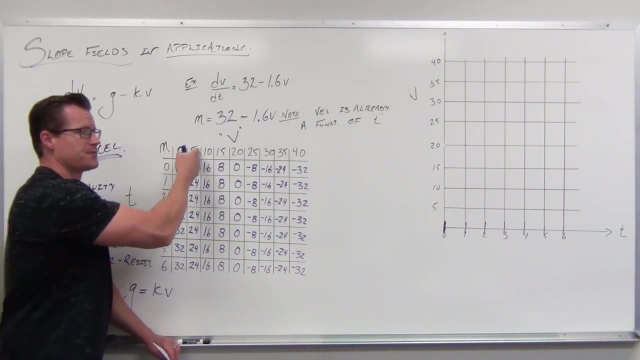 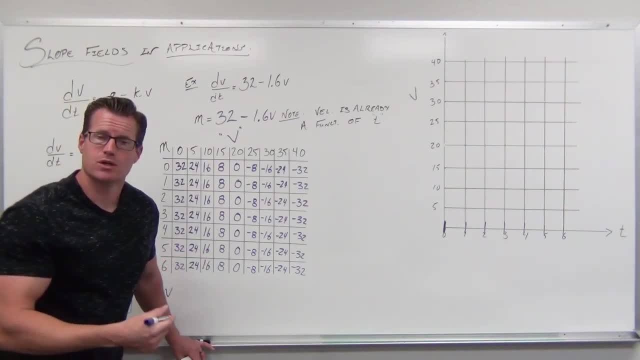 Then our slope starts to decrease from 32, and we talked about why that was So. if you jump out with an initial velocity, you immediately encounter air resistance, which means your velocity can't change as drastically as it did if you jumped out at. 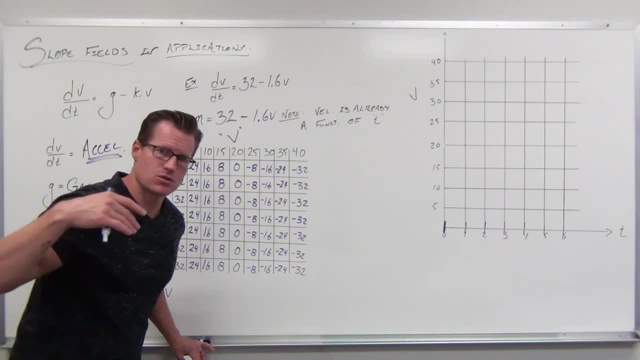 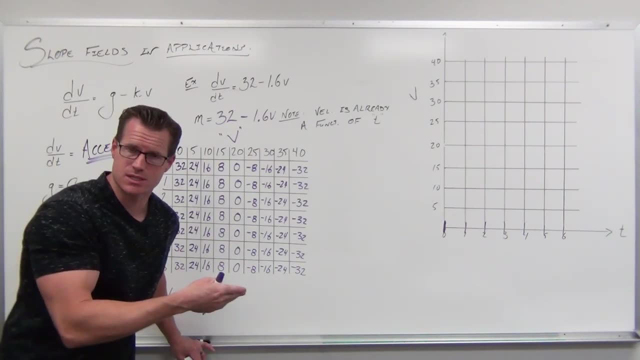 zero. At zero, you have no air resistance. for a little while. That means that you're going to increase velocity by 50% Right faster, because it's only gravity that's affecting you. As you increase speed, you start encountering air resistance. 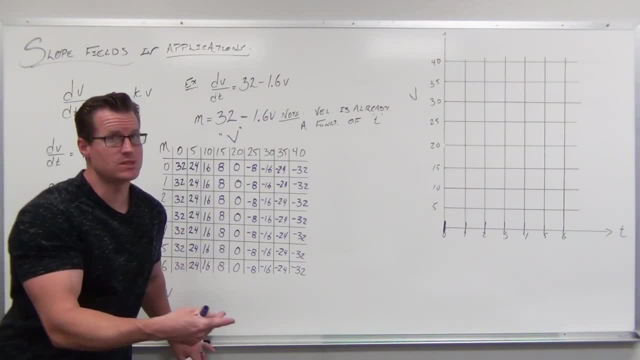 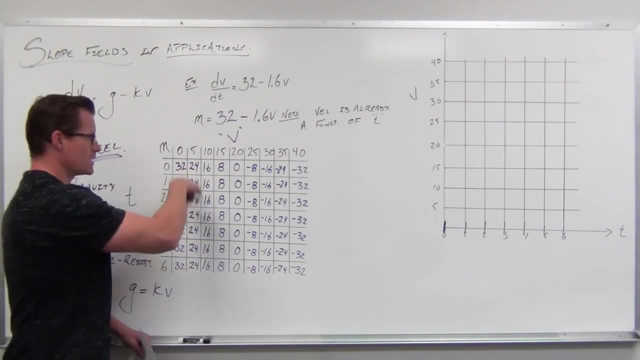 So the way your velocity is changing can't be as drastic as if you didn't have air resistance. So the more air resistance you have, the less that your acceleration of gravity can take over. Here we get 24.. So all along this level we have 24.. 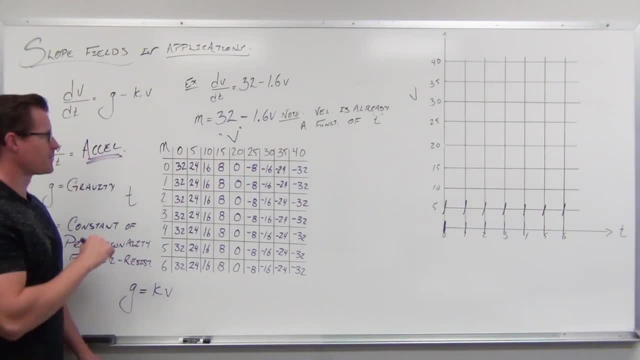 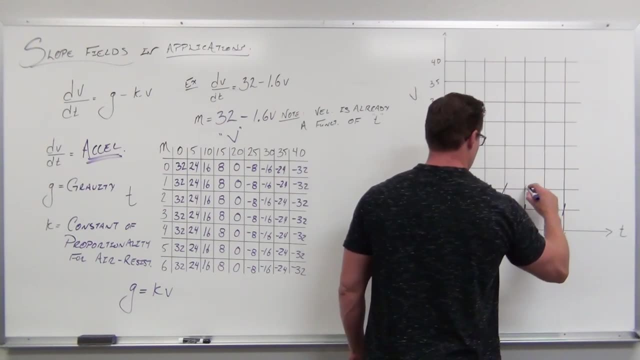 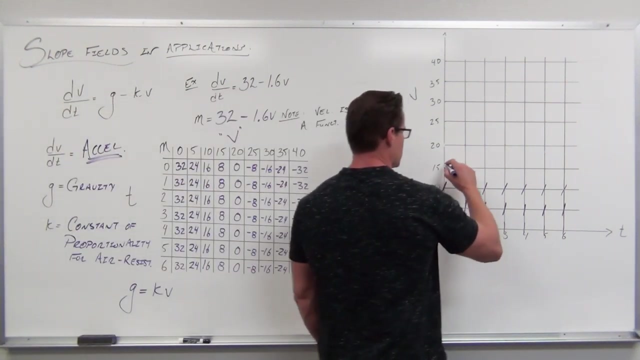 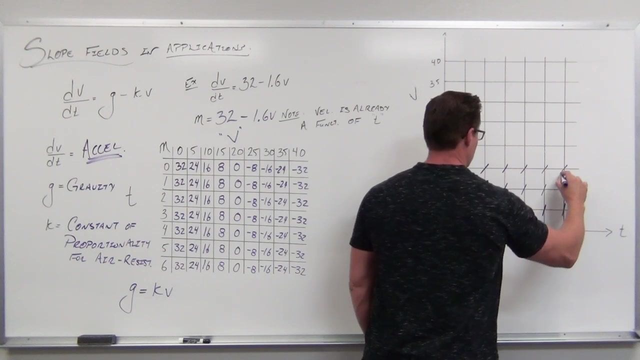 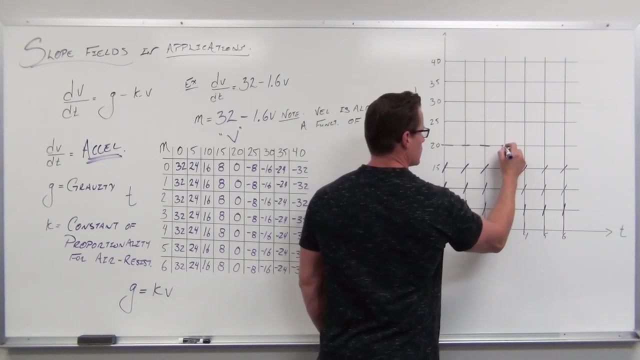 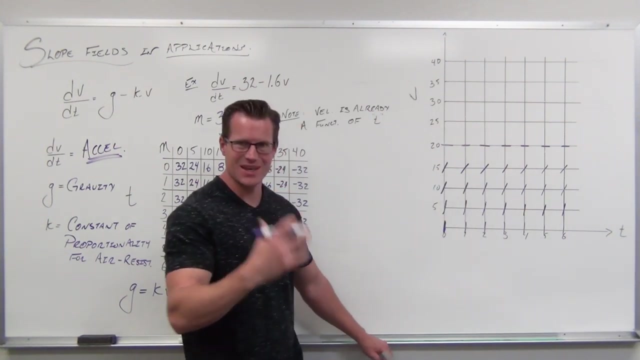 At 10, we have 16.. At 15,, we have 8.. At 20, we have 0.. 0.. 0. And that should be striking to be like. Oh Well, obviously, if our slopes are really no matter where we're at. 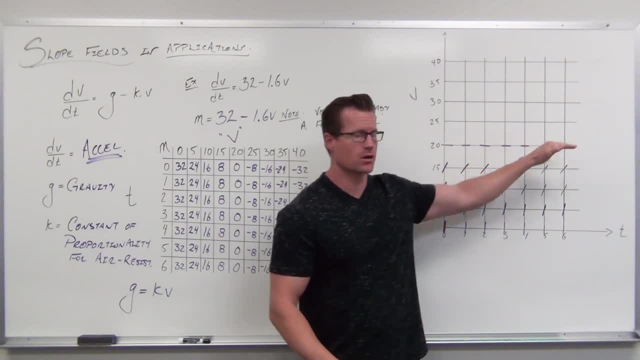 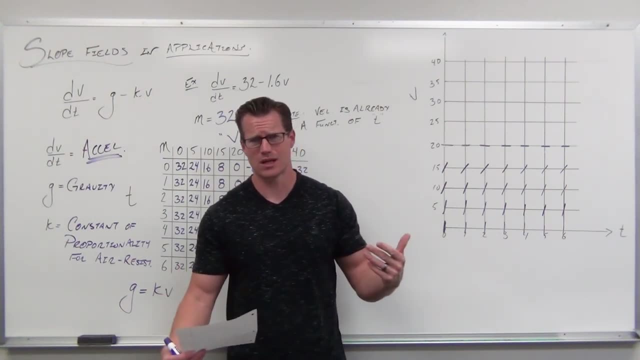 our slopes are going to increase, we're gonna go, uh, we're gonna level out right here. So if we- And this is what I'm saying to you as we're looking at our slope field, This is important because it models real life concepts really, really well. 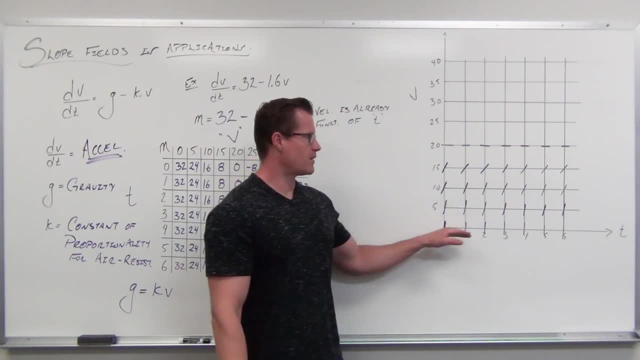 That's what slope fields do. That's how we want to use them. If you jump out at any velocity up to 20 feet per second going downward, you're going to increase your velocity. Gravity is going to overcome your air resistance until you reach that point. 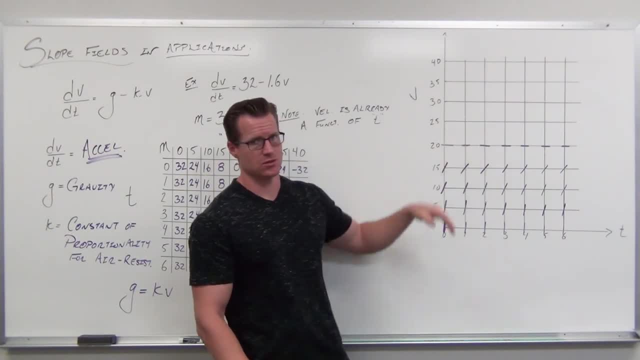 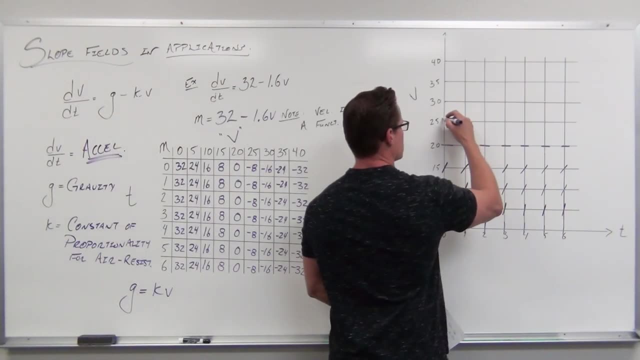 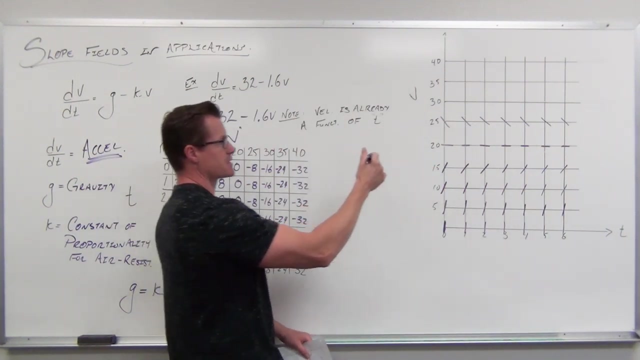 And then you're going to level out If you jump out faster than 20 feet per second down. so let's see 25, you get negative 8.. At 30, we have negative 16.. So it mirrors this. 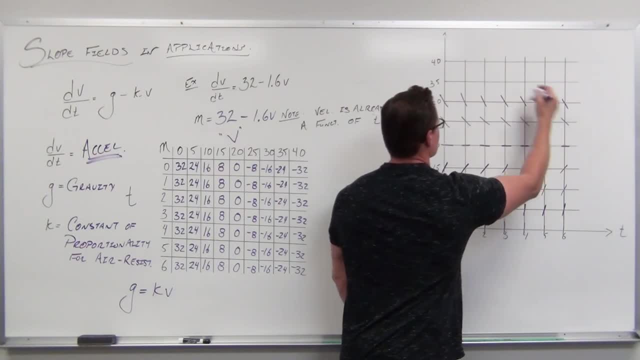 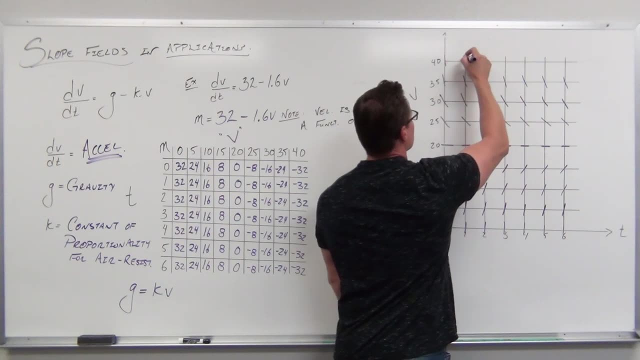 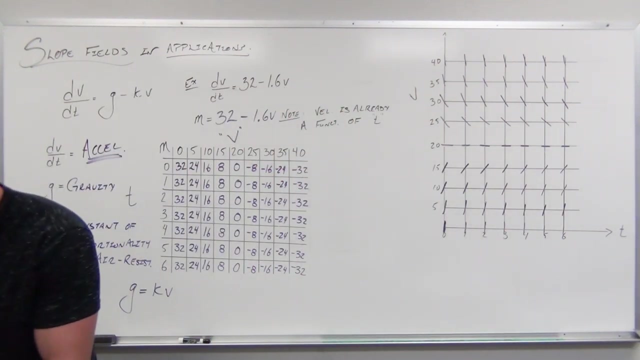 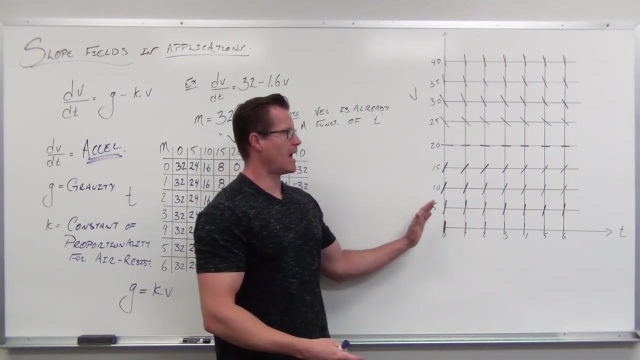 And putting this all together, our slope field gives us how our velocity is changing with respect to time. If we jump out Or fall out Or are putting an initial velocity that's slower than 20 feet per second, This is all saying that, yeah, you're going to increase until you reach that level. 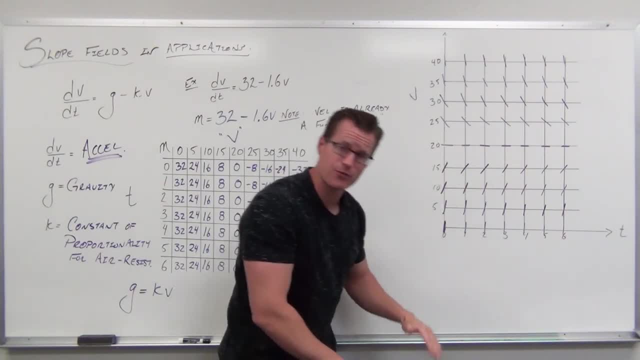 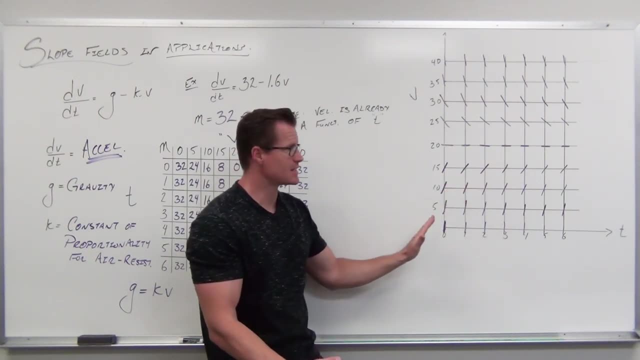 If you jump out at faster, so going downward, jumping downward at faster than 20 feet per second, you're actually going to slow down. Here gravity is overcoming your air resistance until you hit 20.. Here, air resistance is overcoming your gravity. 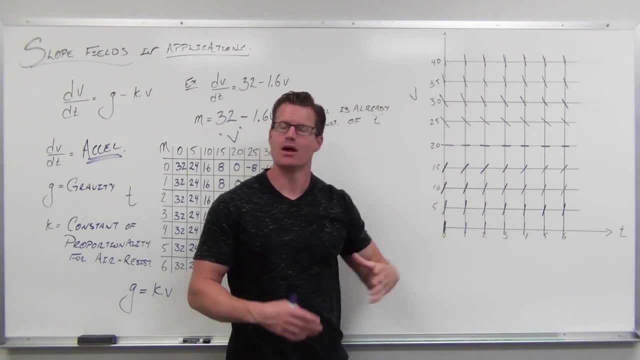 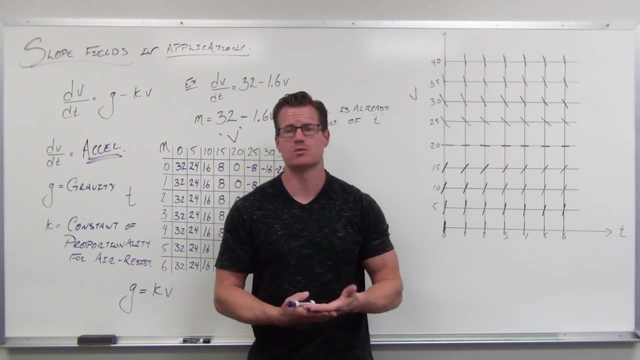 So this, This would be bigger than gravity. That's why you're slowing down. What's going to happen, though, is that these two things are going to level out in real life. Your air resistance and your gravity are going to come into some sort of equilibrium, an equilibrium solution. 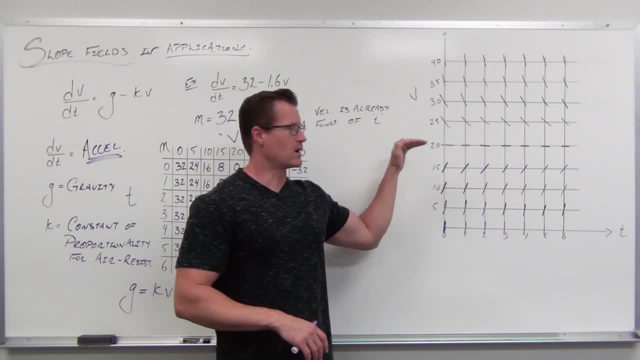 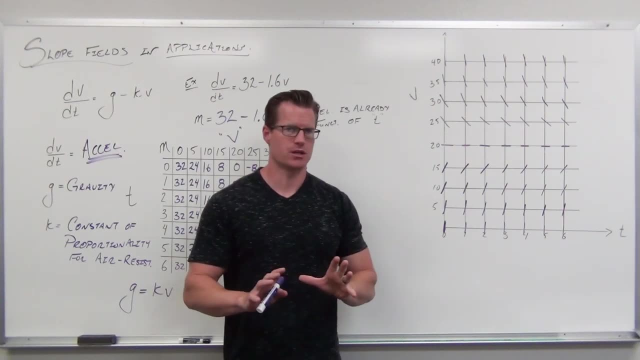 That's what. this is The solution where, if you started at 20, so 20 feet per second- you jump out, you're jumping downward at 20 feet per second. you are not going to feel a change, So it's not going to feel like you're increasing speed. 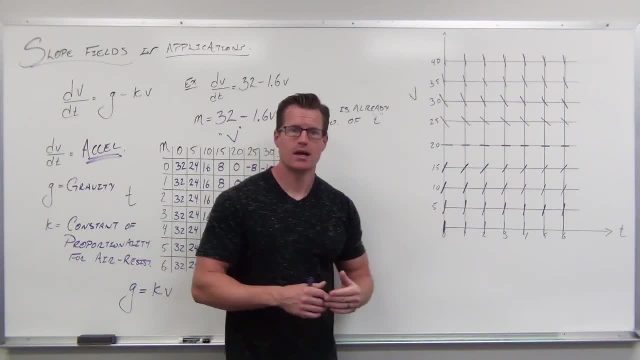 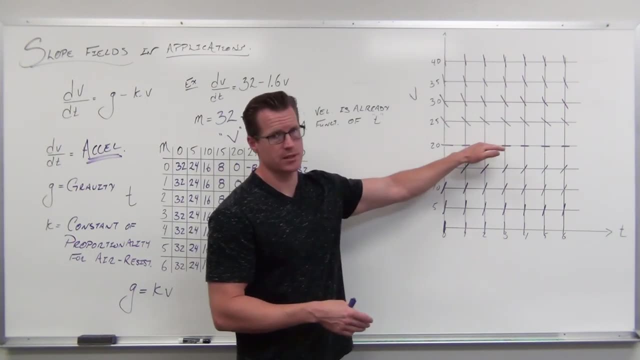 It's not going to feel like you're decreasing speed- Jump out slower than that. It's going to feel like you're speeding up because gravity is pulling you faster than your air resistance when you start to a point to that level of 20 feet per second where we even out here. 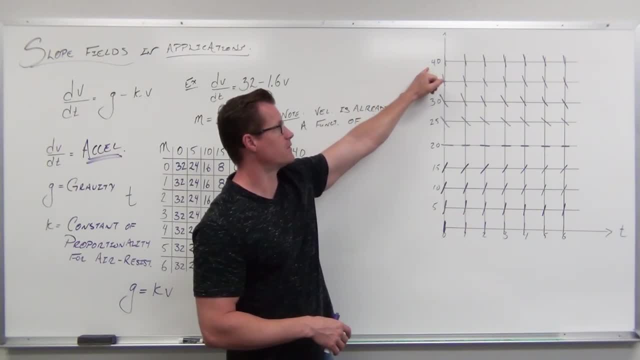 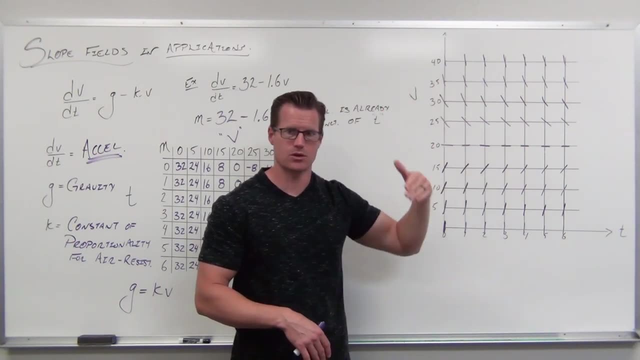 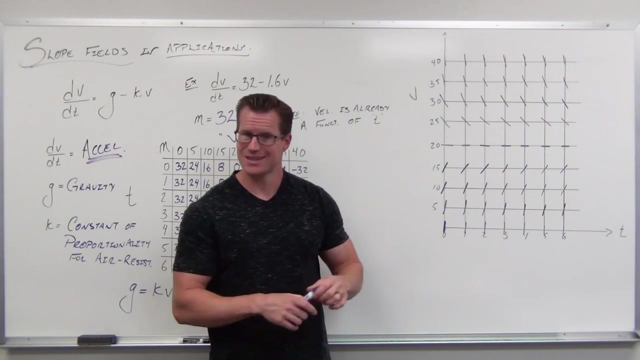 If you're jumping faster than that. so jumping downward faster than that, you're going to feel like you are slowing down. Your slope is negative. here You're going to be decreasing your velocity until you reach that equilibrium, until you reach that limiting velocity. 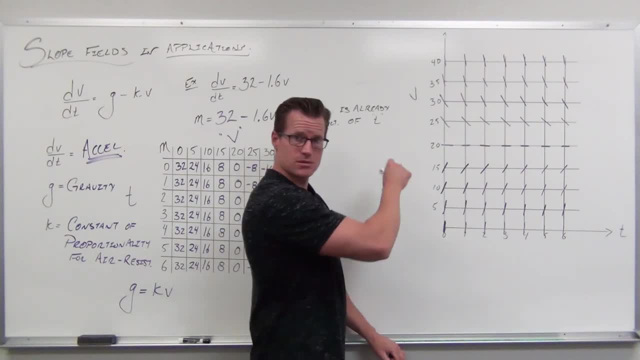 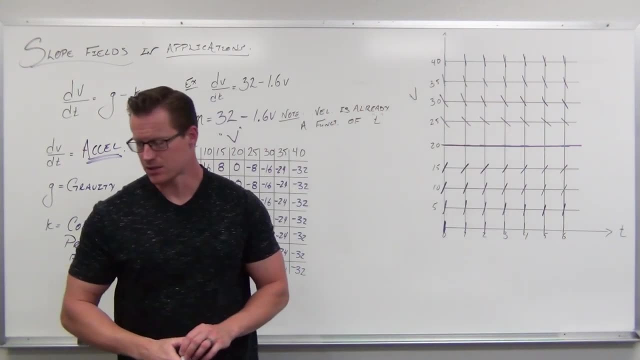 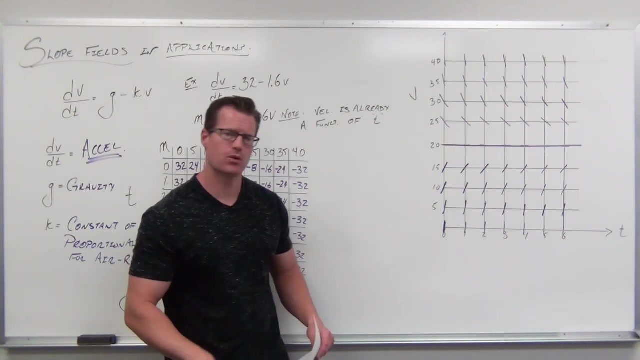 Isn't that weird, It's kind of cool. So right here, this 20, that, right there is our limiting velocity. No matter what happens, whether you jump out, whether you're pushed out, jump downward, whatever- you're going to reach that velocity, given enough time. 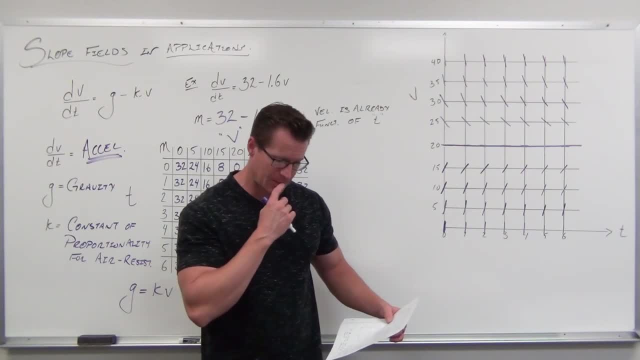 So that's kind of interesting. We'll figure out how much time you really need. Again, you're not going to jump up, So we don't have a negative velocity. You're not going to jump upward. This is the helicopter idea. 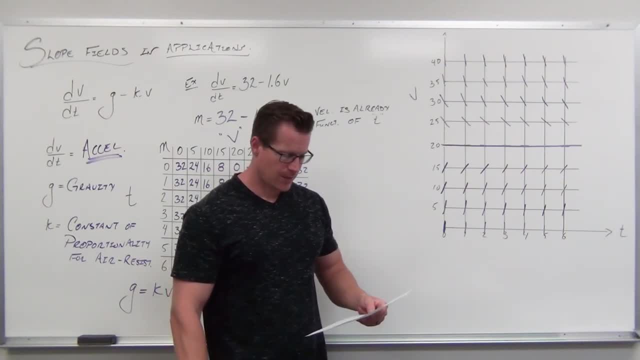 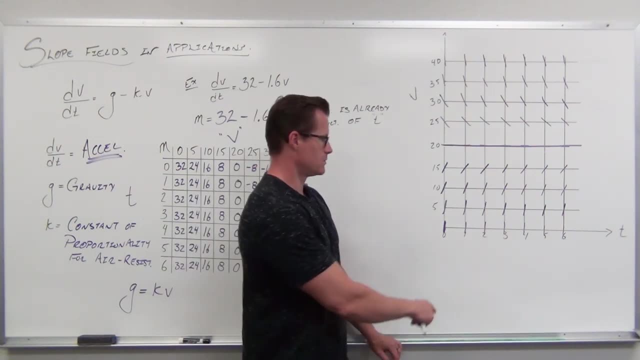 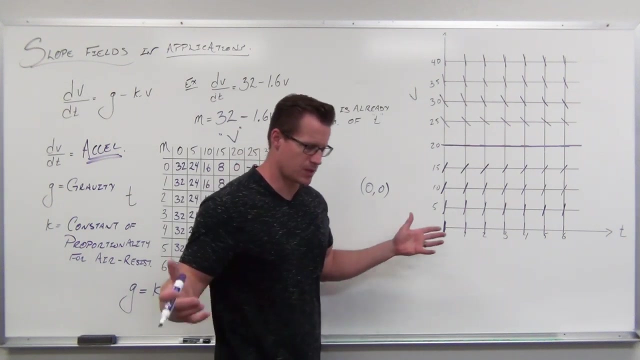 So our limit is this: 20 feet per second. So let's say that we jump down at zero, So we start here. So remember, from our slope fields, if we had an initial condition and a starting spot of zero, zero, So at time, zero, we're not traveling any, but we're just jumping out. 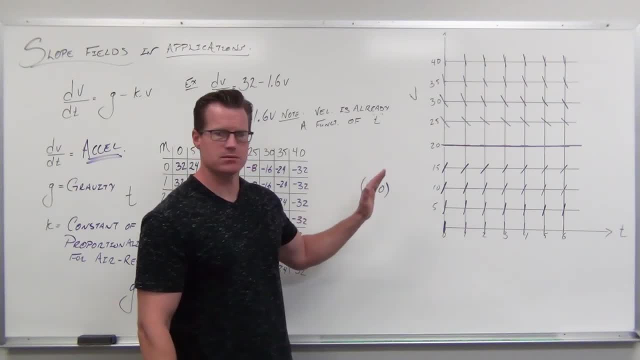 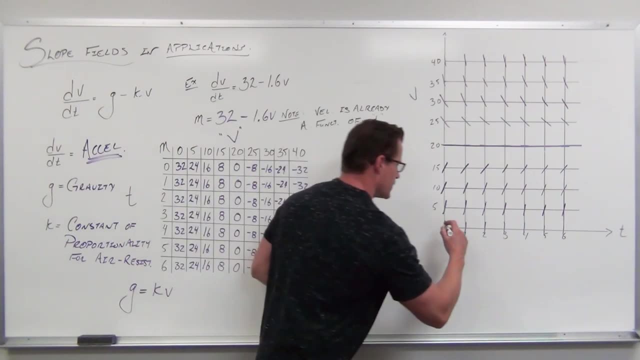 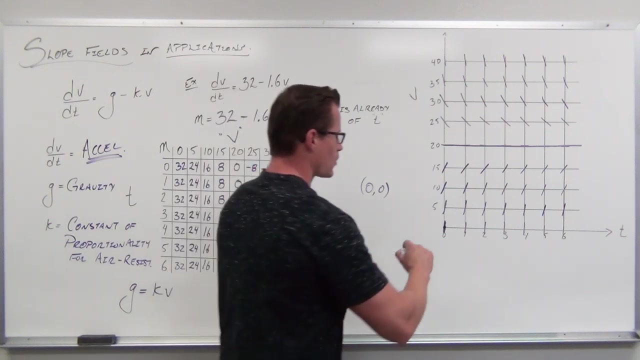 We're not jumping downward. Let's see how fast we actually are. We're actually coming up to that 20 feet per second. So, starting here, remember that slope fields. they've got to find this curve that matches these slopes. So we're starting really steep. 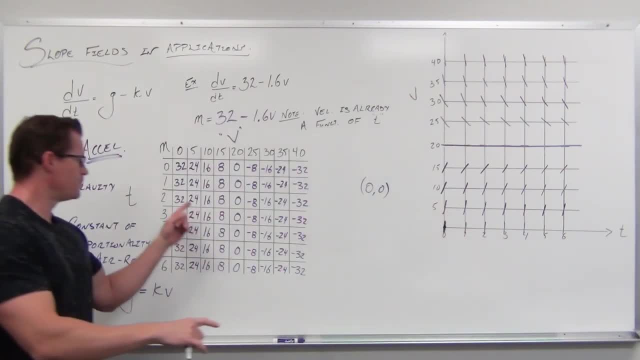 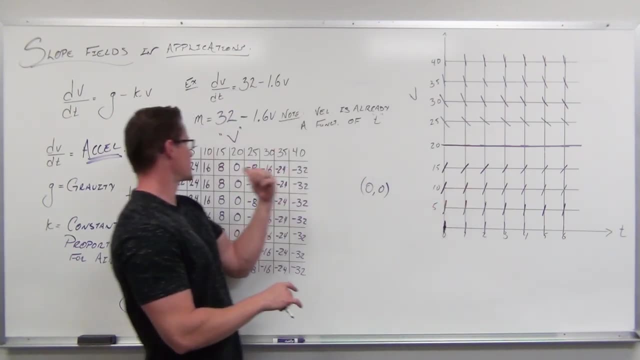 When we get to this level, we better have a slope of positive 24.. So when we hit five, we got to have a slope of 24.. When we hit 10, we got to have a slope of 16.. Then eight. 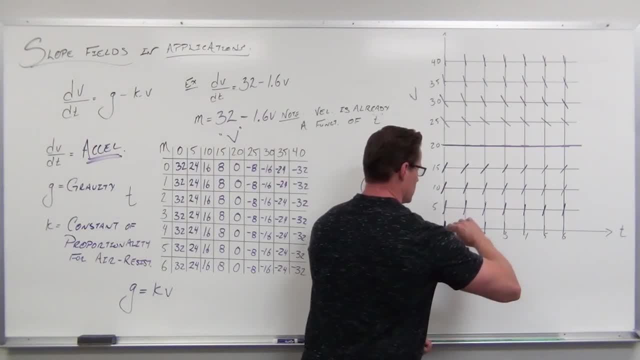 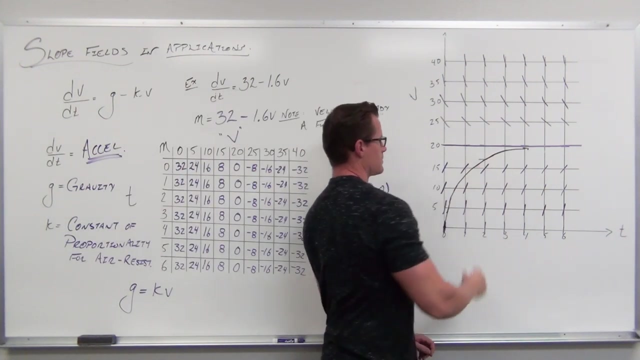 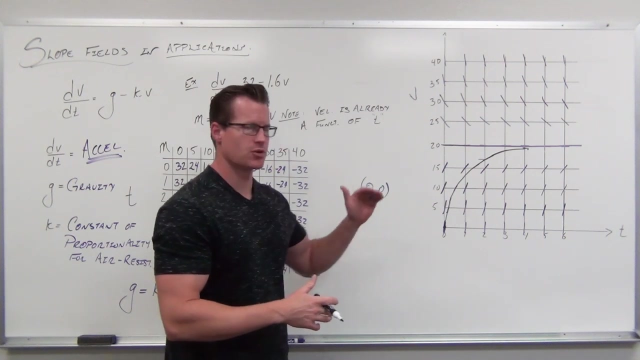 Then zero. this right here looks like it's about 17 and a half or something. so we reach 17 and a half feet per second after only two seconds. so we go from zero to 17 and a half feet per second in one two. that's like well, what. 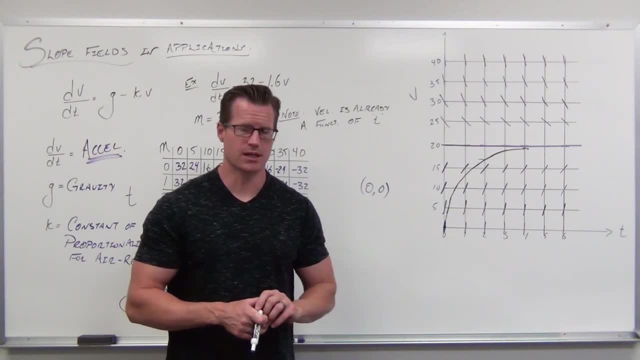 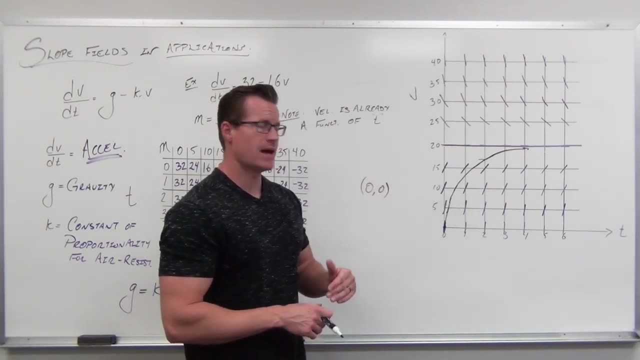 is that that's a good percentage of 20 feet per second when we, if you divide that, so do set about 17 and a half divided by 20, that's a percentage of time of that limiting velocity that you reach after two seconds, so you can find. 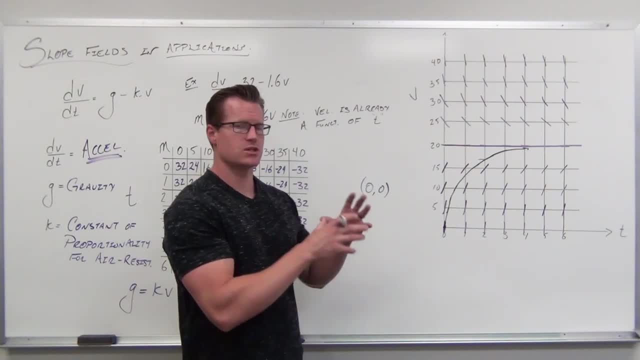 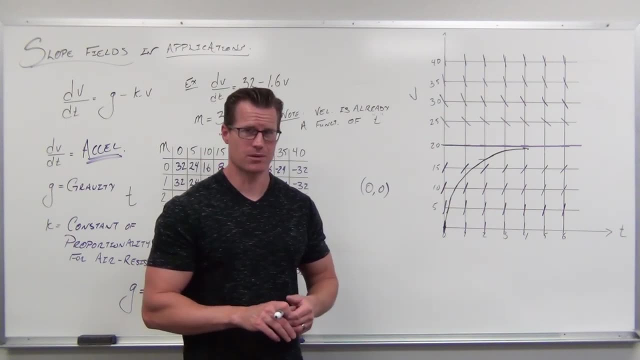 out how long it's going to take you, you to reach a certain percentage of 20? now, theoretically, do you ever reach 20? it's an asymptote. so technically no, or theoretically no, but that's the limit. so you're going to get to that point. get closer and closer and closer, but but. 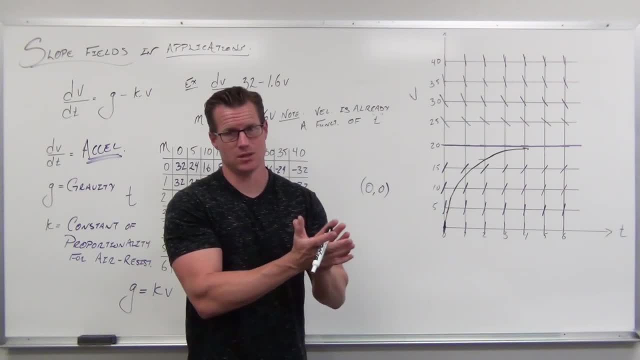 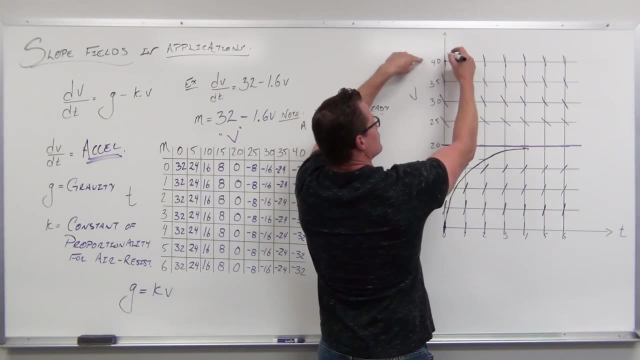 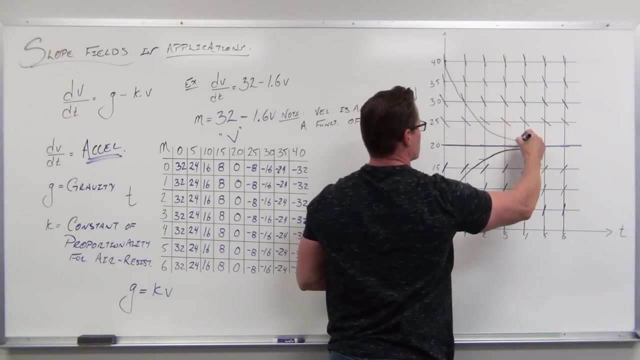 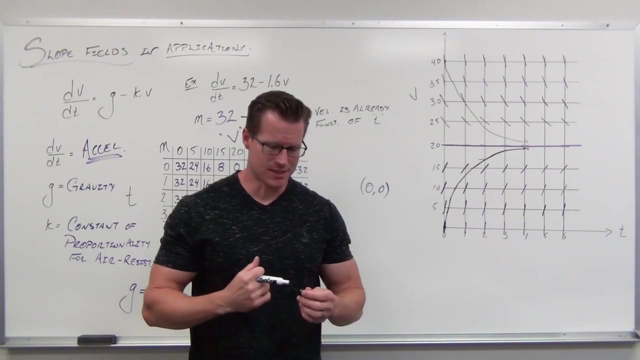 you're never going to exceed that. that velocity you can only limit to it wild. now let's let's say you jumped out it at 40. same thing happens in reverse: you're going to slow down until you reach your limiting velocity. I hope this is making sense to you. it's very interesting the way that works in real. 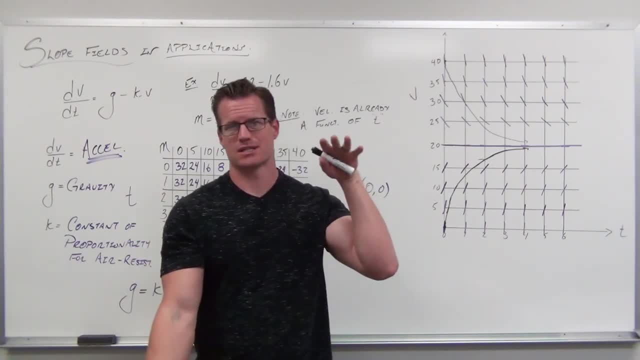 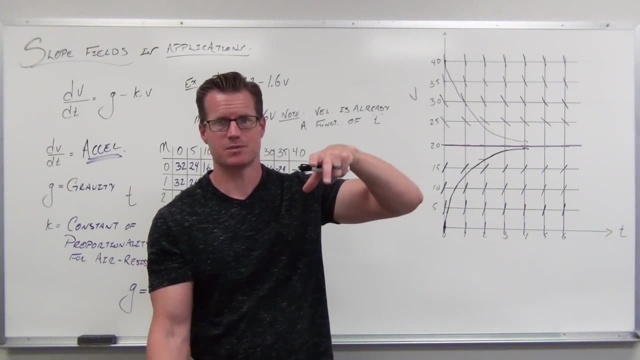 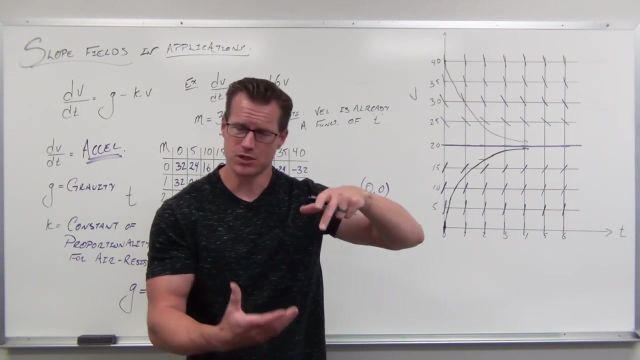 life, because at some point, when you really do think about it, gravity and air resistance- if you're jumping out faster than gravity, you can slow down. you're jumping out slower than gravity, you're gonna speed up, but that air resistance is forcing you backwards. so when you're, when you're, when you're, so when you're, 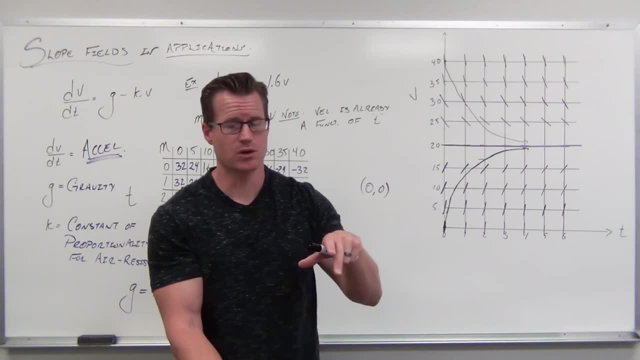 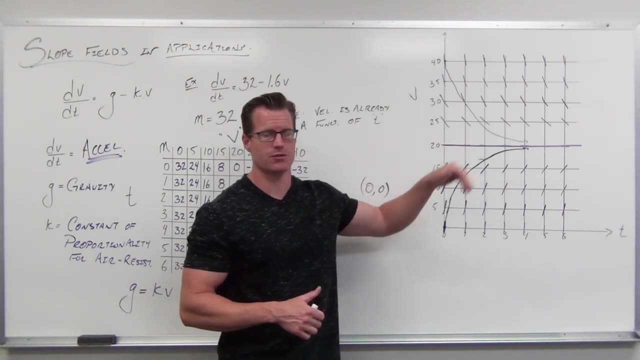 jumping out so fast, air resistance is overcoming gravity. when you're jumping out so slow, gravity is overcoming air resistance. at some point they meet. that's what we're talking about with an equilibrium solution. if you jumped out of 20, that could be able to change faster or slower than that you're gonna reach. 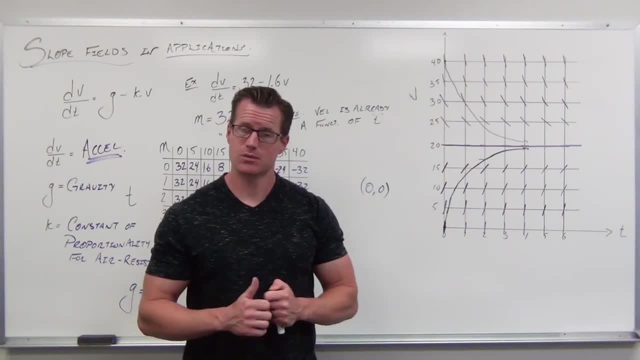 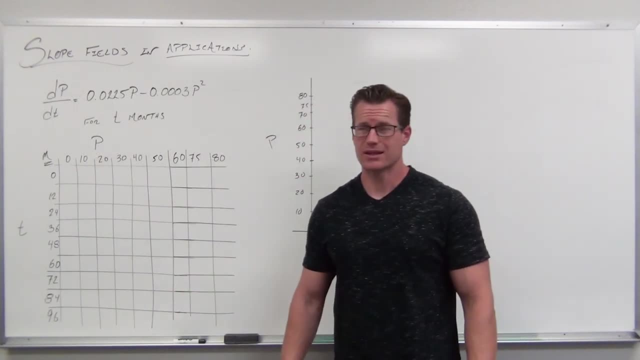 that limiting velocity. we're gonna do one more example about population. we'll talk about limiting population or carrying capacity, so hang on for that one. I'd like to walk you through one more example about population. we're gonna do this very quickly. the idea is exactly the same, I just want. 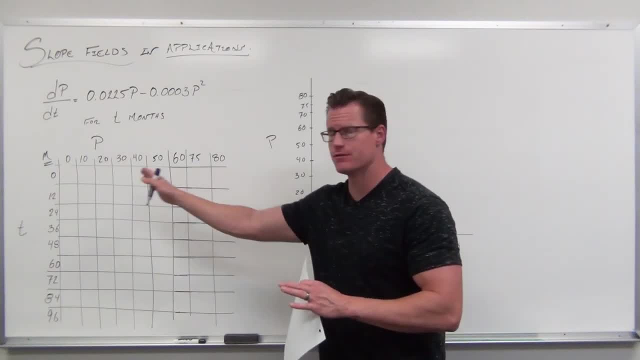 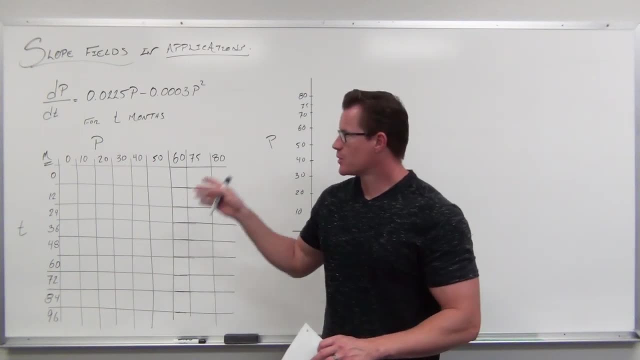 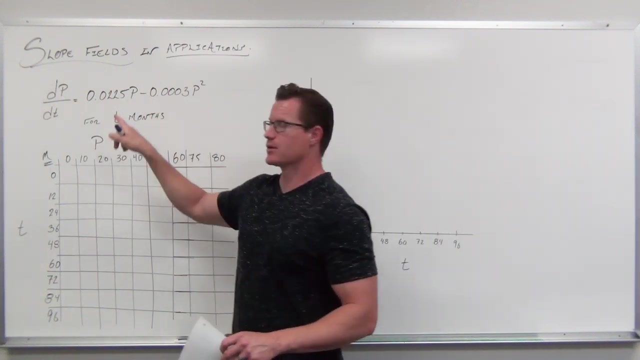 to show you how slope can do some funny things in the middle of this, this problem, to show you that on the slope field, and to talk about something called carrying capacity. so so when we look at this, we have the way that that a population is changing with respect to time. now again, we don't have a T up here. 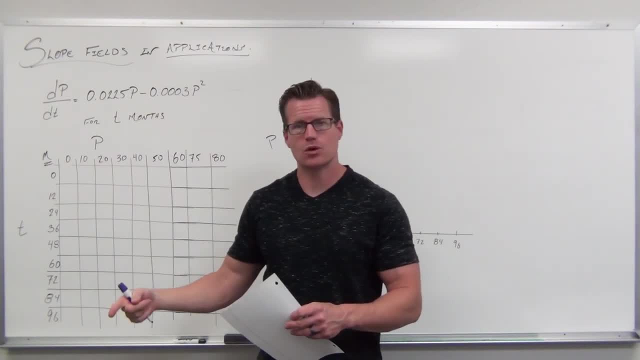 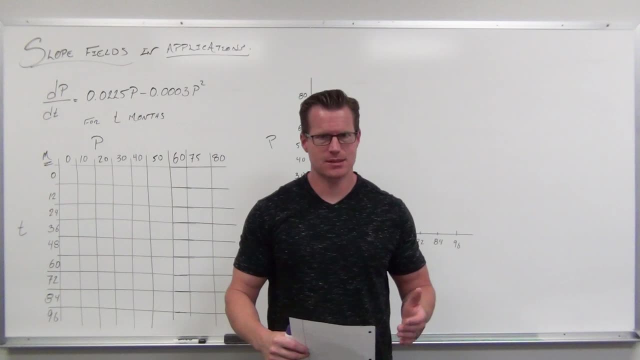 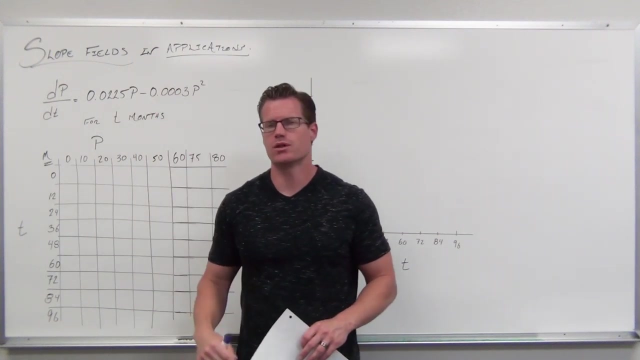 but the population itself is a function of time, and so the way that population is changing, or you think of it, the, the acceleration of population, that's kind of weird. but how fast is the population growing or decreasing? well, that's given by this for a certain population, with T being. 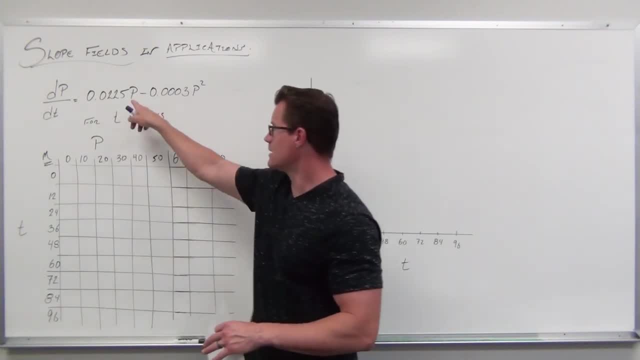 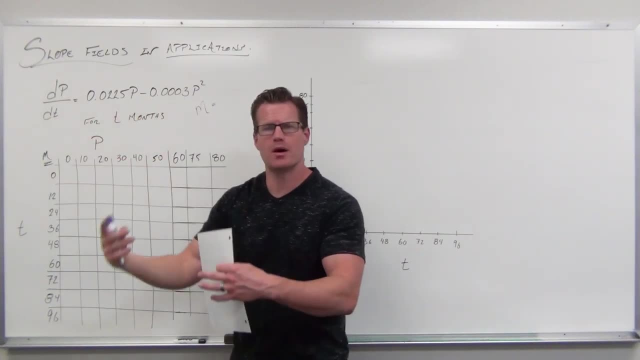 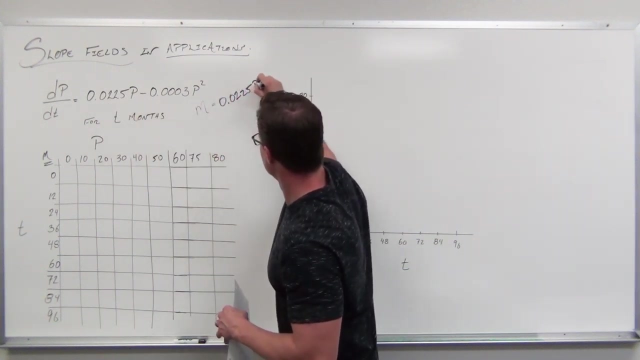 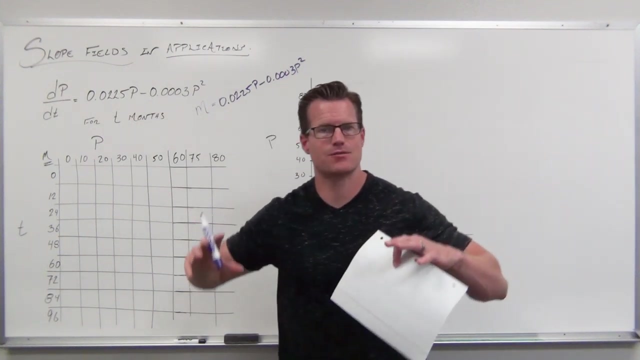 months now, because we don't have a T in here. our slope is still equal. this here is the slope of the population. the way the populations change with respect to time is still equal to this, but there's no T involved. the P is a function of time already, so it's involved in that population. well, if we 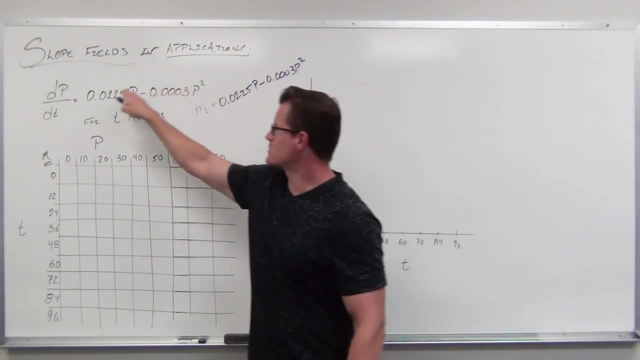 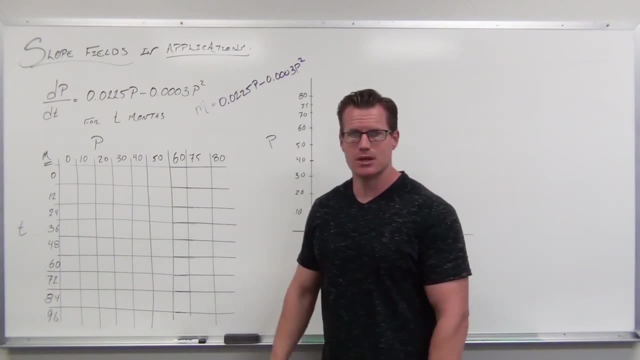 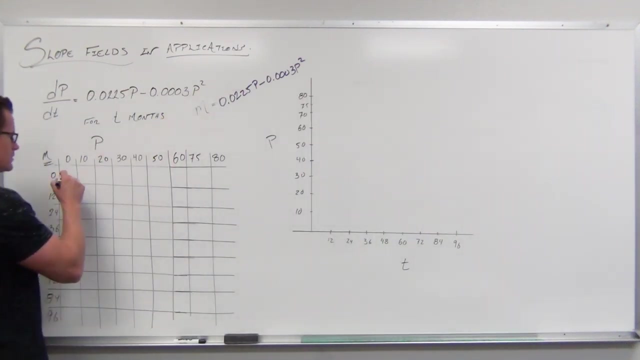 want to go ahead and do a slope field. our slope is given by this function of P, function of T, with our dependent variable P in there. let's just start plugging in initial populations. so what if we started at zero? well okay, zero minus zero, these are all going to be zero. do you see that it's not going to? 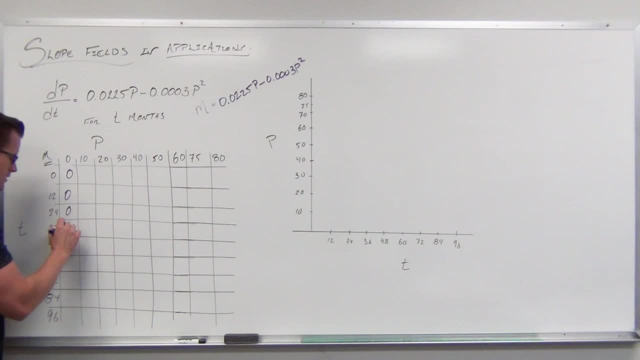 change as far as what time we have. we're gonna have zero this whole way down. same thing happens for all this. I'm just gonna give you one number. if we start with 10, our slope would be 0.2 all the way down. if we start with 20, 0.33 would. 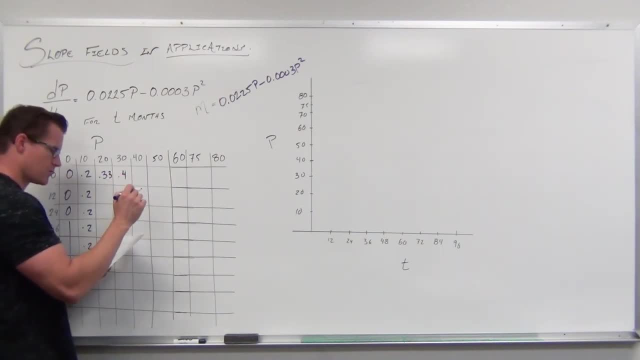 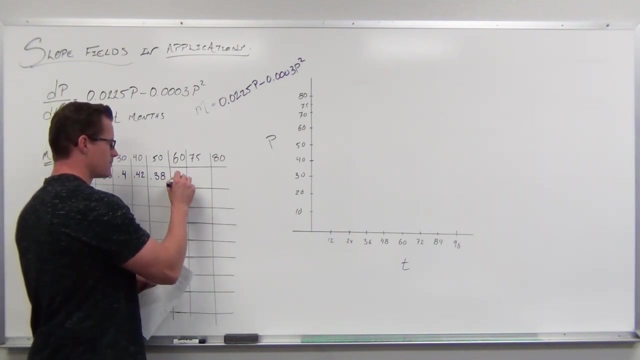 be our slope. start with 30.4 would be our slope, start with 40.42 would be our slope, start with 50.38 and you notice something funny kind of happening. so our slope is increasing and then it starts decreasing again. that's a very interesting than 60 would be 0.27, 75 would be 0 you're looking for. 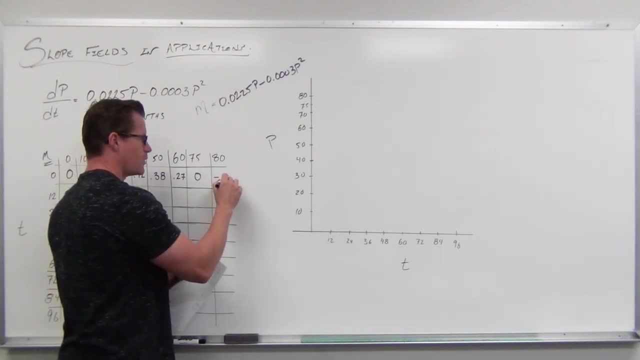 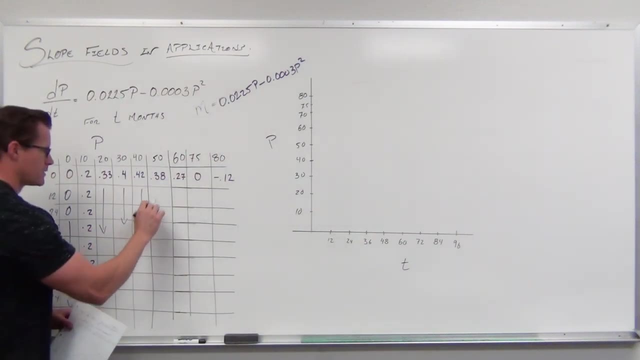 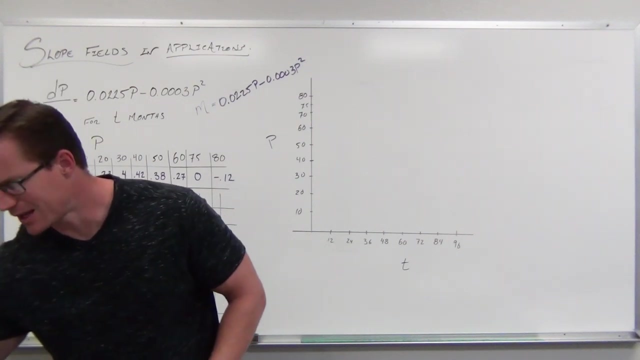 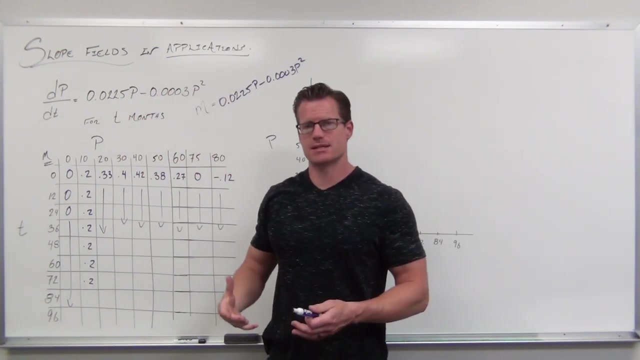 that, and then 80 would be negative 0.12. here's what this is saying. this would be all the way down for all of these. remember my goal in teaching you this, not just how to do it: understanding what's going on. if this is the way that population is changing, what this says is: 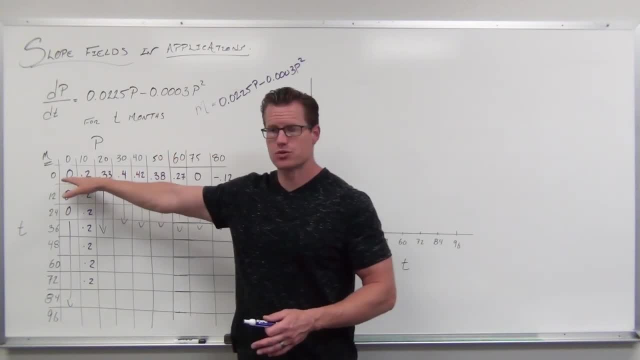 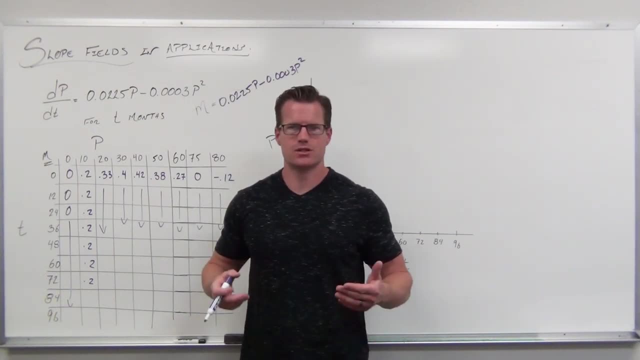 that if you start with these populations. here's what is going to happen. if you start with a population of 0, are you gonna see any growth? obviously not. there's nothing to grow. if you start with a population of 10, whatever this population size is, you're. 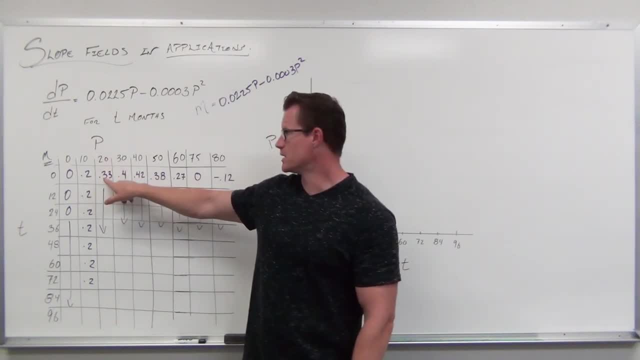 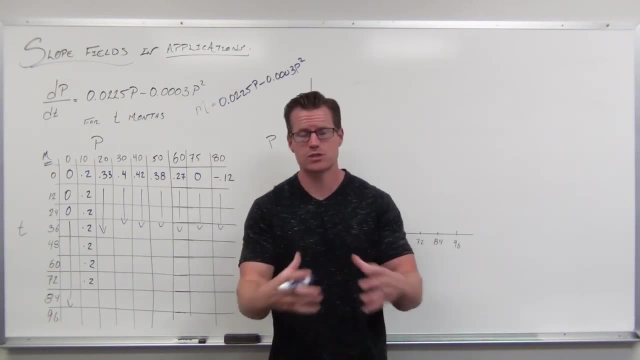 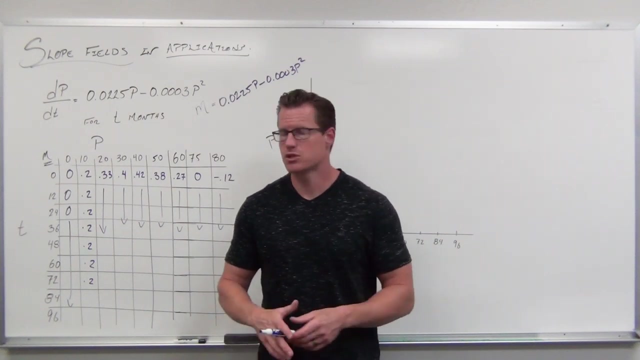 going to immediately start seeing a population increase: 20 increase, 30 increase faster, 40 increase faster. that should make sense, right? because if you have more things to reproduce, the population should be growing faster. to a point because our natural resources aren't limitless, which means that as we 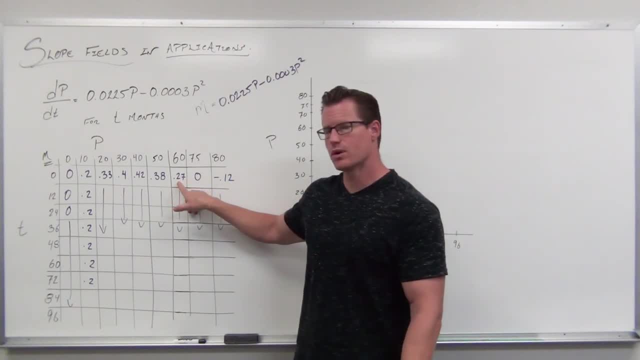 get higher and higher and higher. our population is growing, but not as fast, because we're reaching some sort of a limiting factor here. at some point we hit what's called a carrying capacity. so if you start with 75 units of population, whatever that is, it's not going to grow. it's not going to. fall. it's limited. if you start with more than that, you're gonna actually have a die-off. if you put, say, you had a really small pond and you just you dumped zero fish in, no fish are going to grow, get that, they don't just spontaneously come. 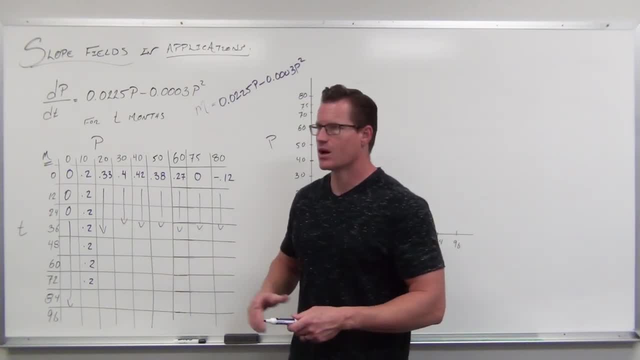 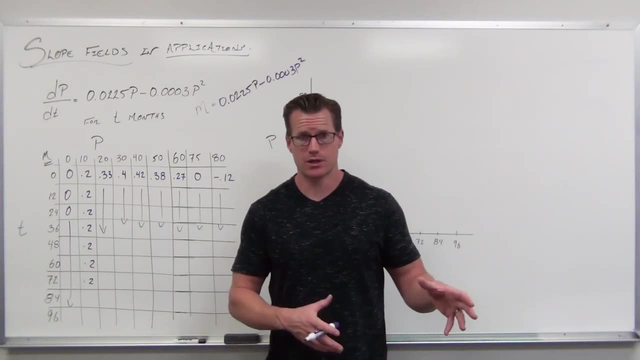 about. that doesn't make sense. if you dump in way too many fish, like a billion fish in a really small pond- there's not enough resources. a lot of them are gonna die. so as we start having our population go higher and higher and higher, it makes sense that at some point we're not 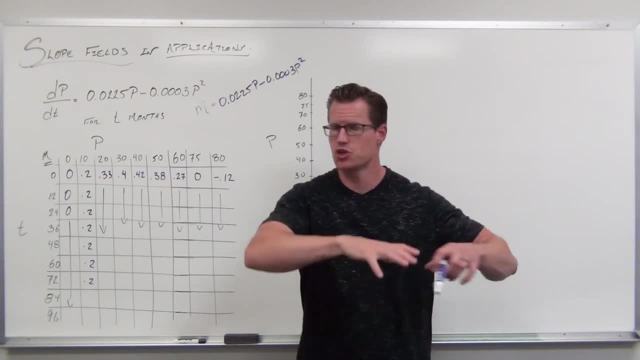 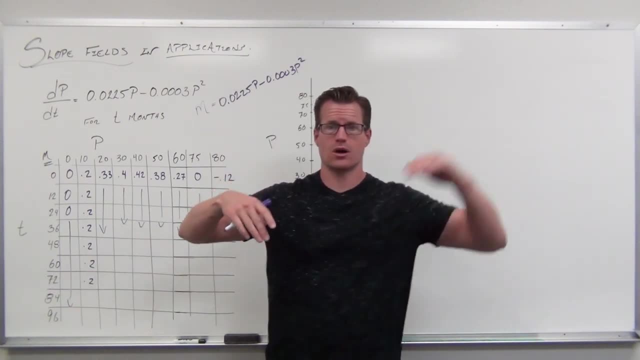 gonna be able to grow anymore. in fact, we're gonna start dying off because there's just too much of this population in one spot. there's a middle ground then, because if you start low and it's gonna grow and you start high, it's gonna die. there's both Ryan, that's kind of fun. then at some point there's this: 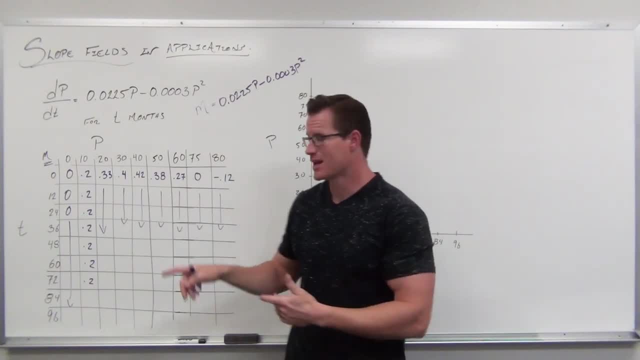 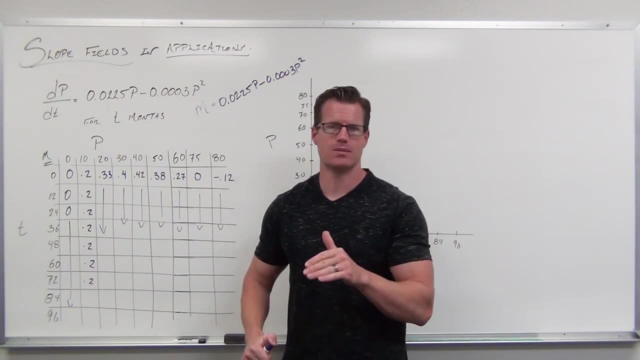 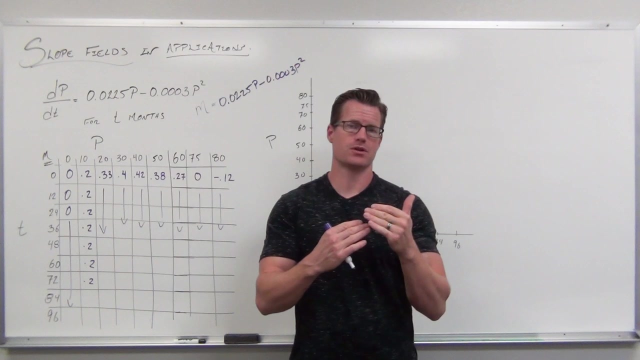 equilibrium solution and that's what that 75 does. that zero right there. look, positive slopes, negative slopes- there's got to be a zero. that right there. that's your carrying capacity. that means that no matter whether you start lower or it's not zero or higher, you are going to level off. you're gonna limit yourself to. 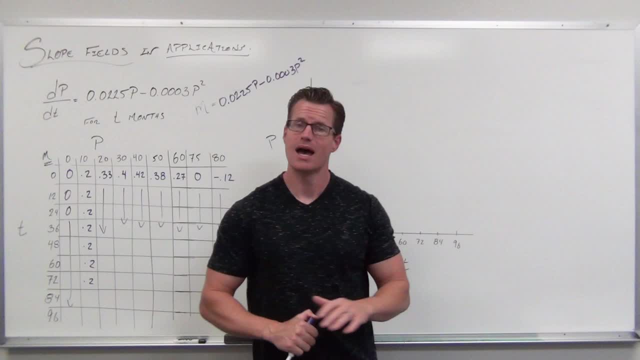 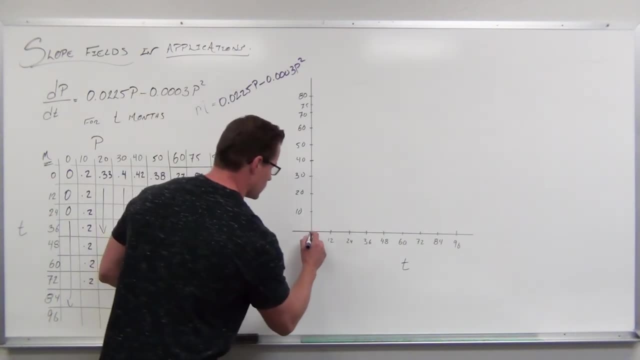 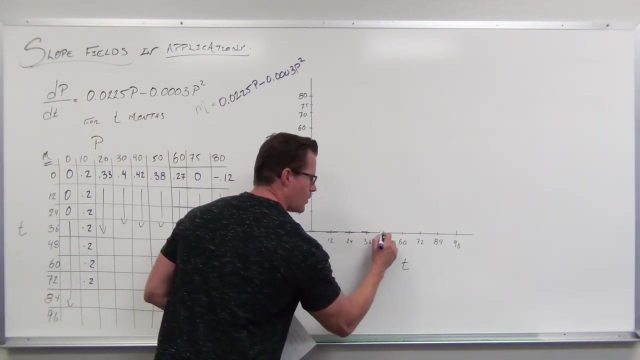 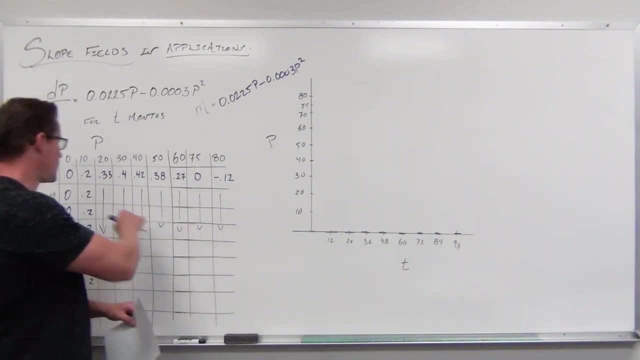 that 75 units of population, whatever that is, and the pictures gonna bear that out. so I'm gonna do this really quickly. but at zero, zero, we have of course zero, and if we have population started zero, we're gonna have zero all the way, no matter if we start off with ten. so we're gonna have this part of this. 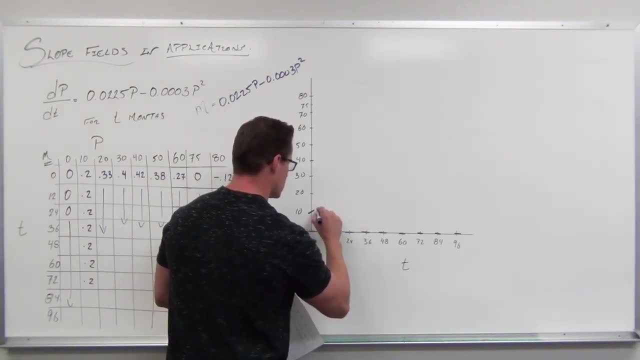 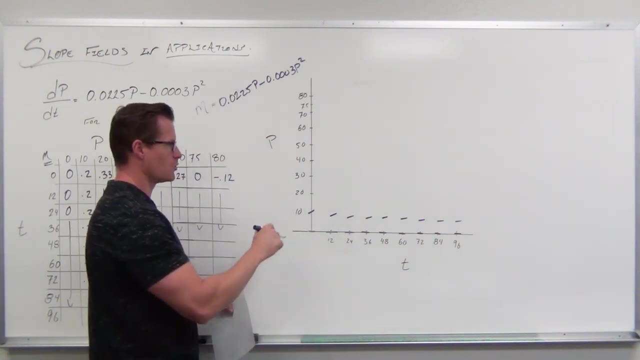 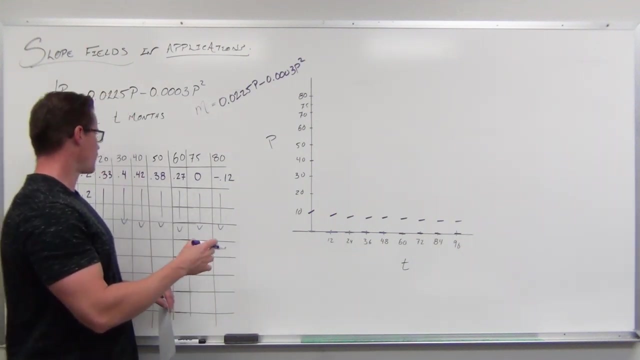 slope of 0.2. so all the way along you get a little point two slope and we're going to increase until we get to 40 populations dropped. we're gonna increase until we get to 40 populations started. next wave let's go 40 population start an initial population of 40 units. 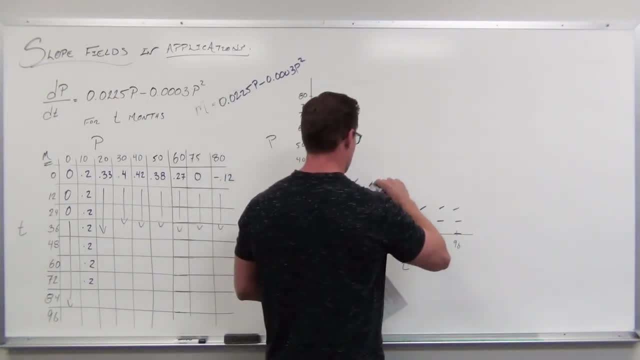 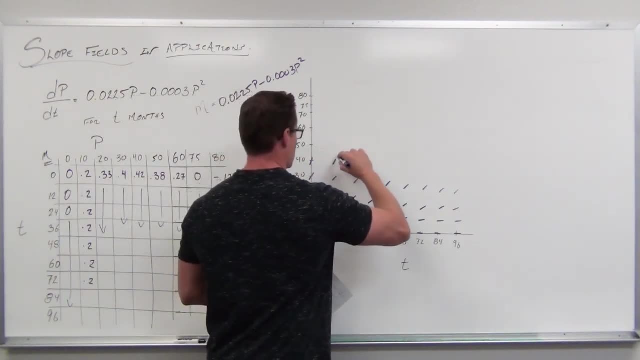 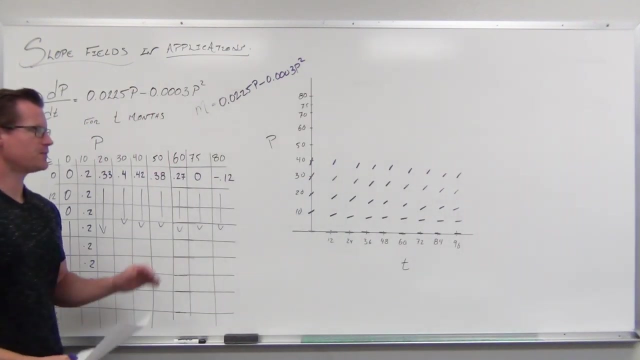 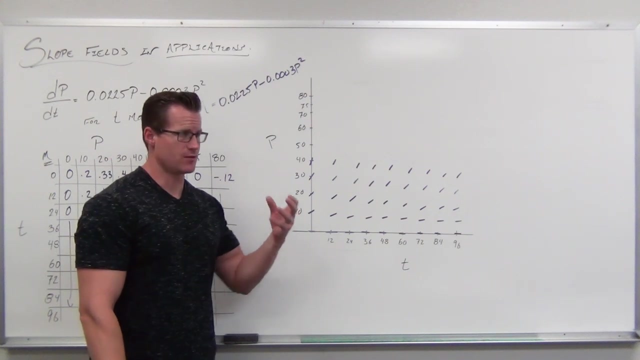 I'm kind of exaggerating my slope right now So you see what's going on. But then once we get to 50 we start to slow down. So the most rapid growth that we have is right around start with 40. you start with that much, you have a lot of. 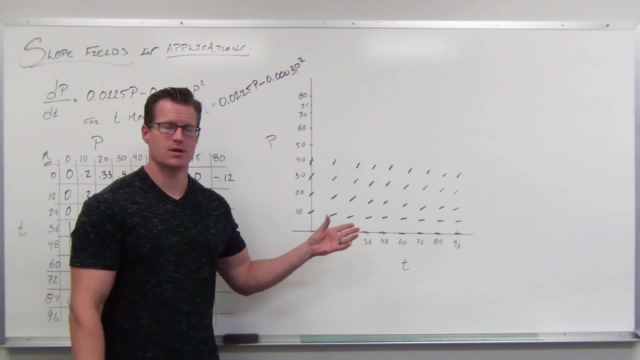 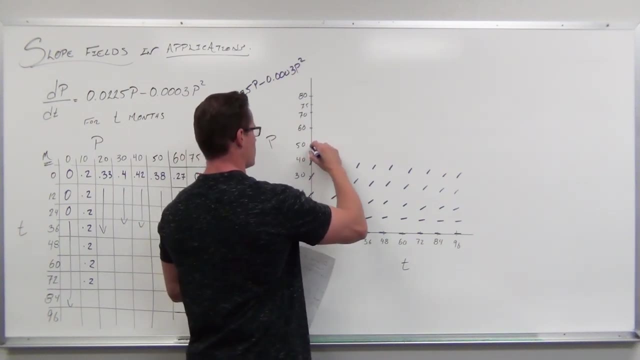 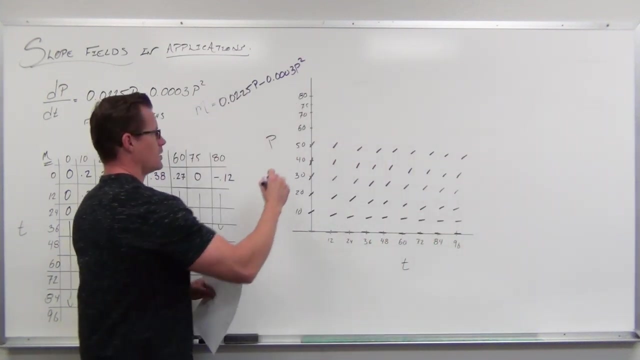 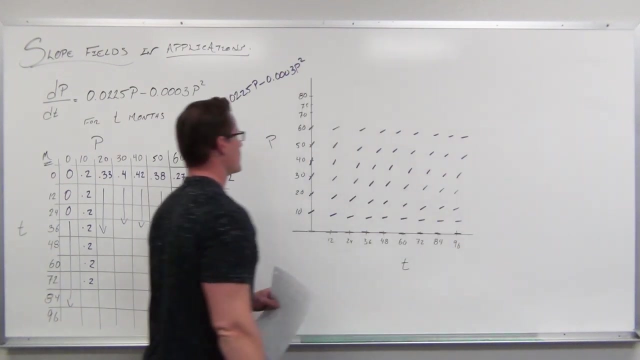 Things, whatever these beans are to reproduce and yet, but you have enough resources to make it sustainable. when we get over that, We start slowing back down And Even slower And probably even so. I don't have this listed here, I'm missing my 70, I didn't want to put that up there- but even slower. 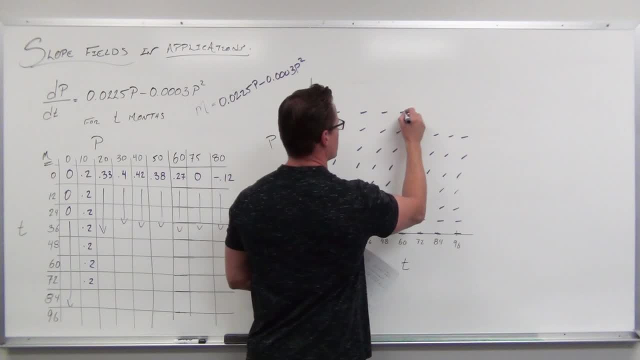 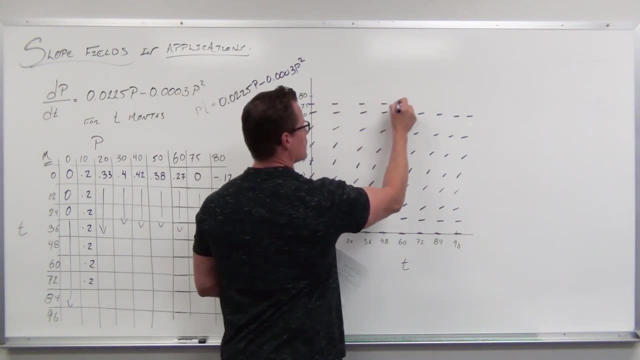 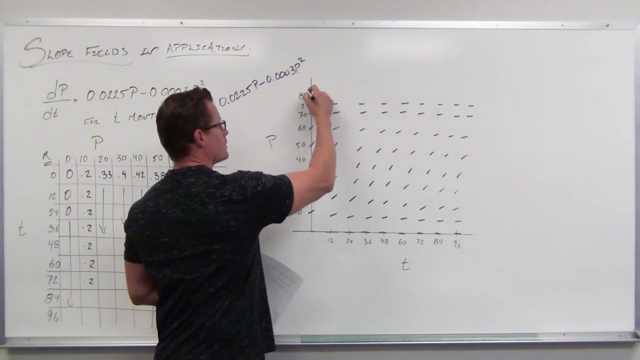 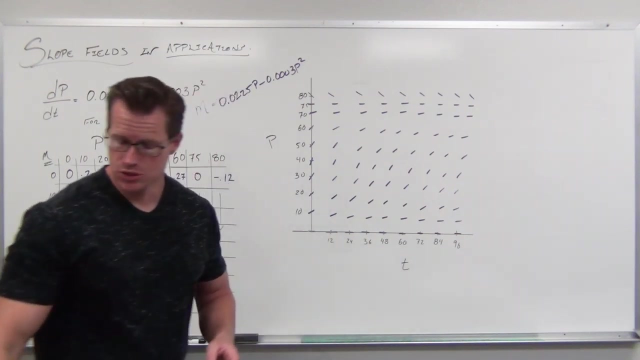 70s, point one, if you want to know What's going on, To the point where we have zero And above that we have a negative slope. So if you are looking at your slope field, It looks like this. This should be really telling what's going on. 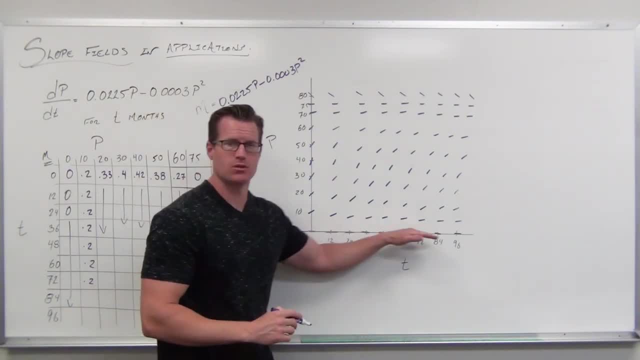 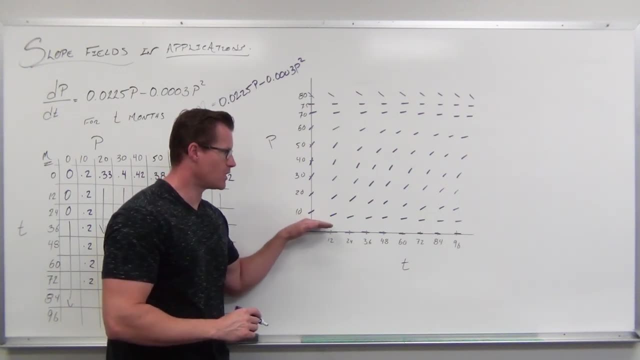 If you start with a population of zero, you are not going to see any growth. Obviously, if you start with just slightly more than that, it's going to grow slowly at first, But then, as our time moves on, look how our curve has to flow through this slope field. 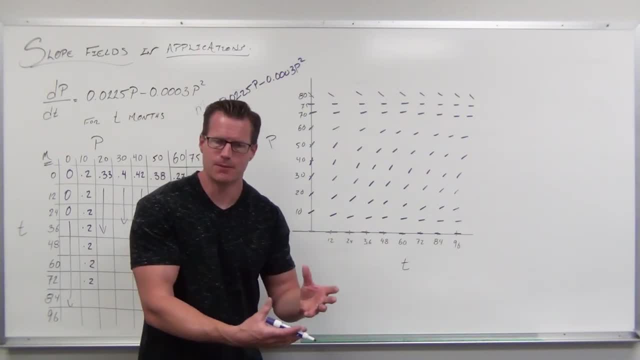 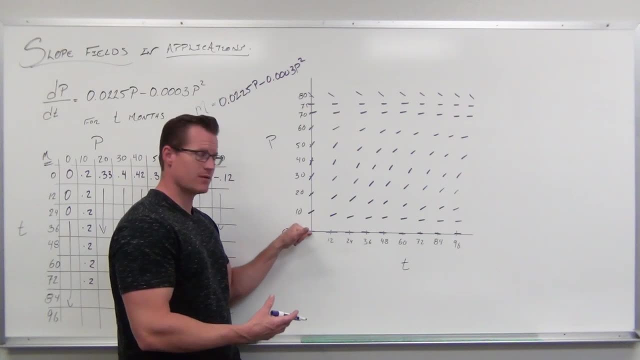 So it seems like, well, time doesn't matter, It does matter, But it's just like you're starting at a different level here, population wise. So if we start at zero and we have no population, no matter what our time is, we have zero. that that is an equilibrium solution. 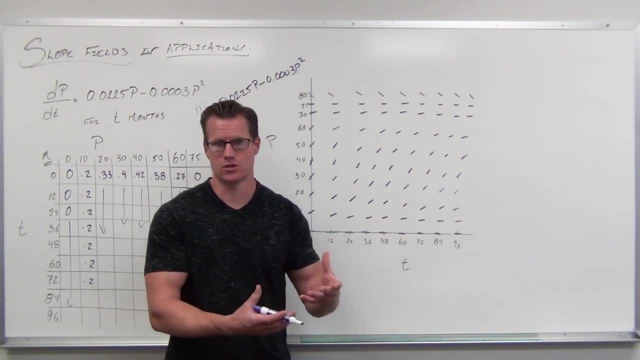 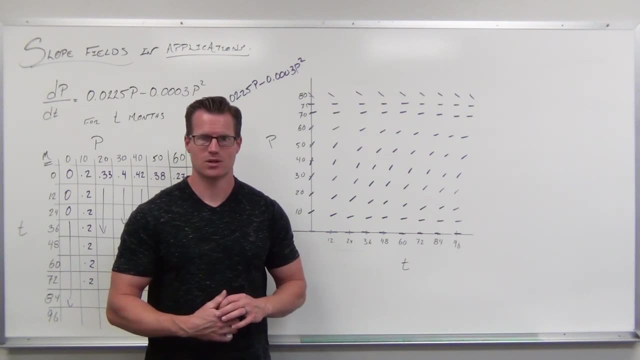 But it's not a good one. I mean, it's like it's like the trivial solution. You know, yeah, it's nothing. It's like saying you're gonna launch a basket or you launch a rocket from the ground at time zero. It's on the ground. When's the rocket on the ground? at time zero. 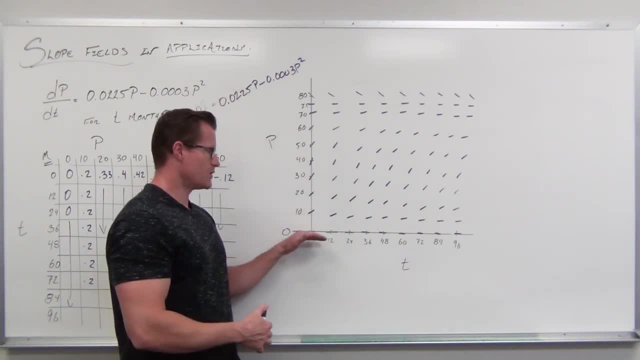 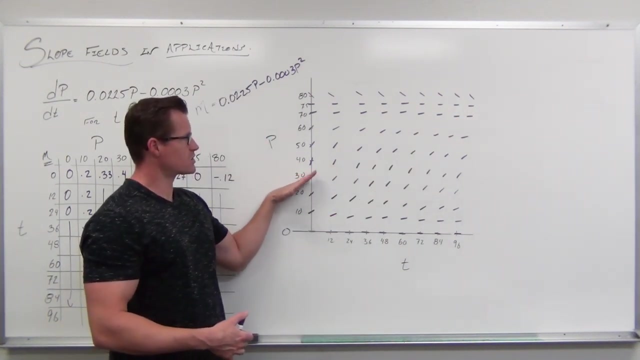 Thanks. I meant like after it's all done, once it hit the ground. So if you start with no population, obviously you're not gonna have one about what time. But if you start with just higher than that, you're gonna flow along this curve. You're gonna match your slopes up, but eventually you're gonna level off. if you start higher, you just 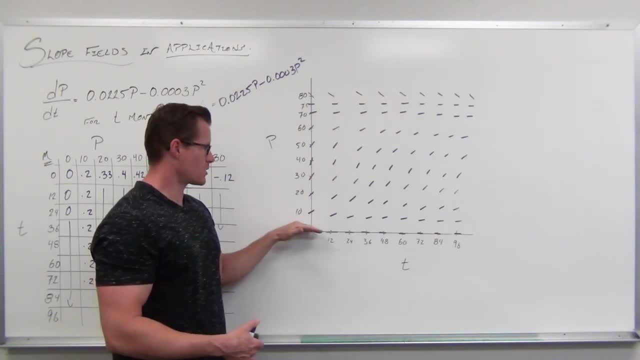 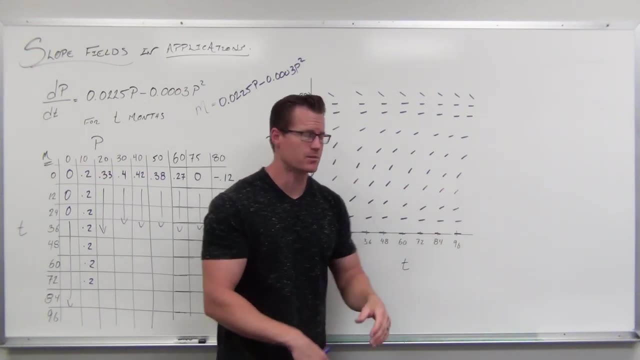 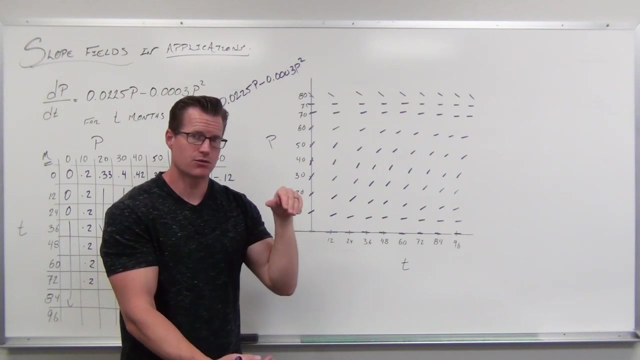 Gain quicker, but you're gonna level off. if you start lower, Yeah, It might take you a long time to finally reach that because you don't have as many many Reproducing items. if you start way higher, Well, you're actually gonna drop. This is like what the last example- your gravity is overcoming your air resistance, or your air resistance overcoming your gravity. 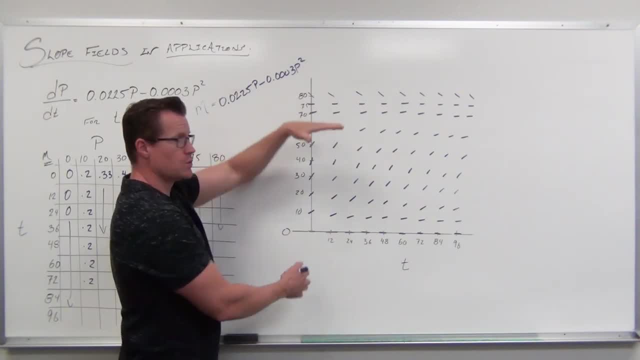 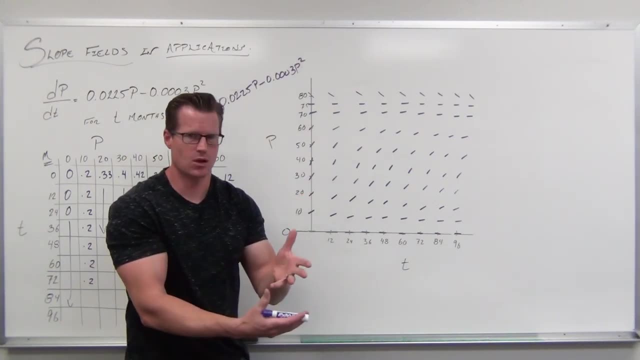 This is the same thing: your level of food is overcoming your population, Which means you can grow, or your populations Come in your level of food list called food, which means your population is going to decrease. You don't have enough. So that's the way that these slope fields work. 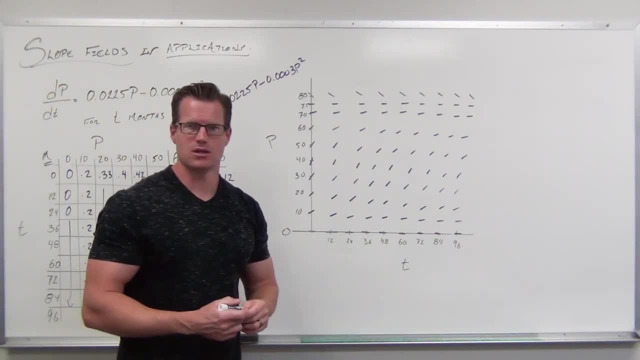 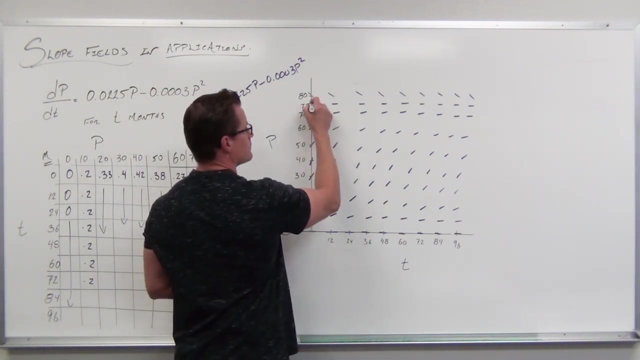 They're looking for the zero. that zero is typically your carrying capacity or your limiting velocity for speed problems or your equilibrium solution if you start with that. So if we started with 75 units of population, you wouldn't change If You started with, let's say, 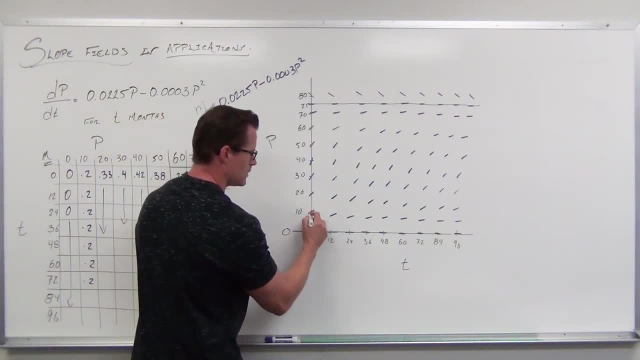 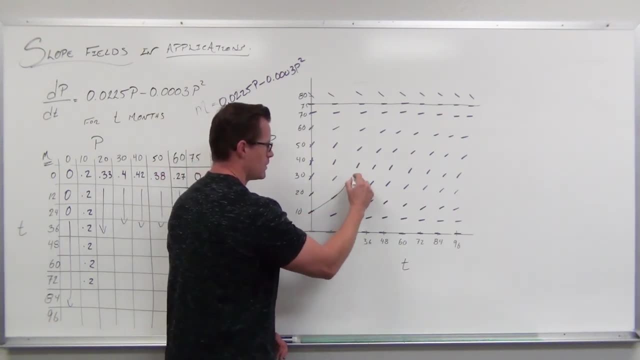 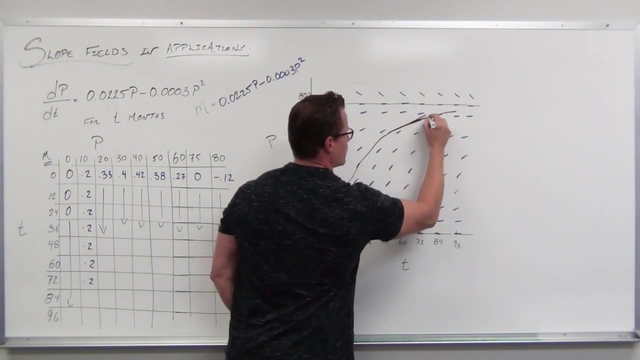 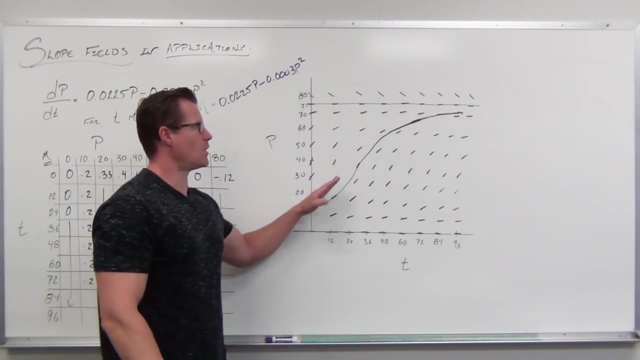 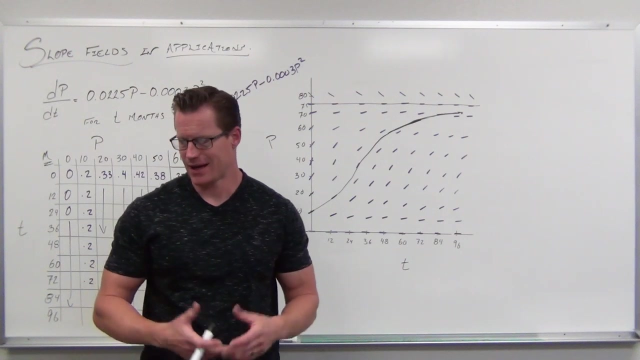 10 at time zero. Make sure you're hitting these slopes as you're moving forward. We travel along, but eventually we are going to level out. So how you can figure out things like how fast would it take you to hit 90 percent of your Or 75 percent of your, your limiting capacity, or two-thirds or whatever. 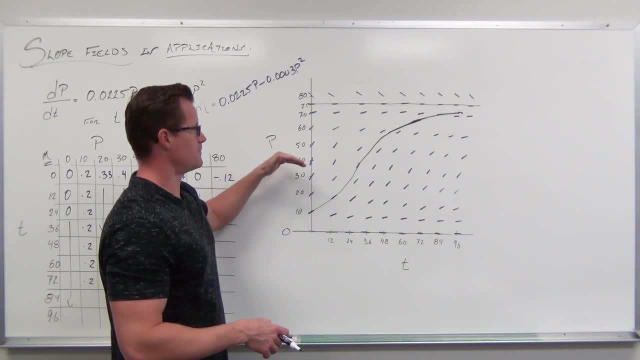 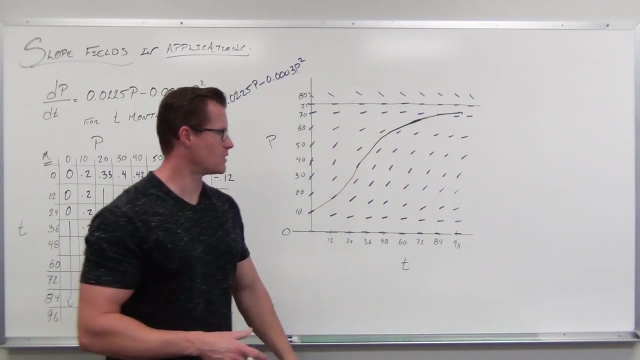 And just look for where you reach, Let's say, 60, a level of 60. that happens. when do I hit a level of 60?? Well, it's going. if I started 10 by sort of 10 units population, Well, that would mean that I get right around 60 months or so. 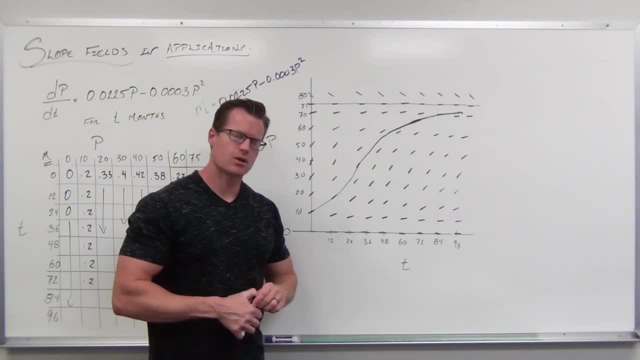 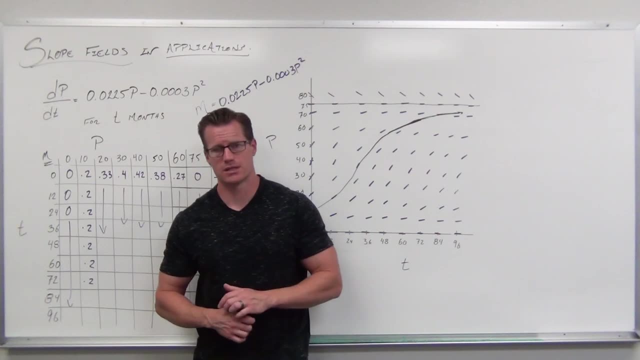 It's like 48, between somewhere between 48 and 60 months. So the whole idea of slope fields one last time is the last we're going to really talk about it. Slope fields model- hopefully some realistic examples that you can't or maybe aren't able to solve with difference equations right now, or maybe even ever. 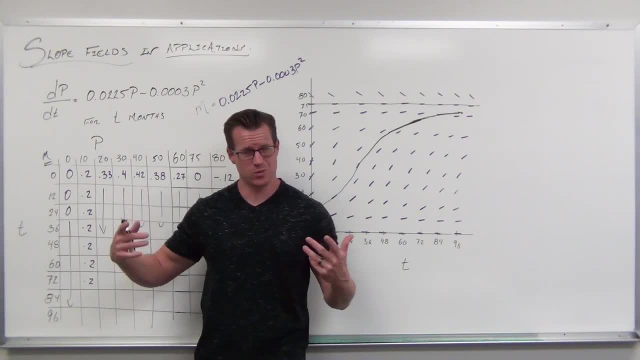 What they do is they consider a first derivative to be a slope, which we have. They say: that's the formula for your slope. No problem, I can just plug in some points. I got it. Then it's going to give you a slope at every point. 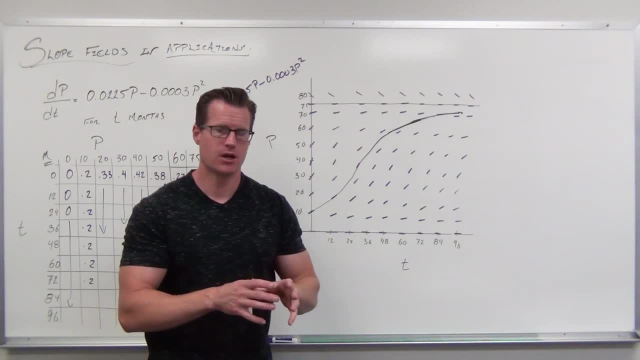 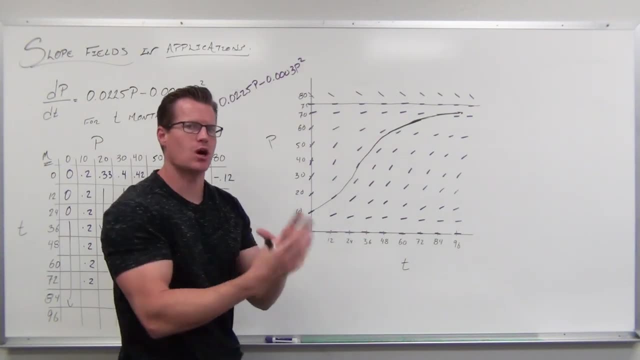 The whole picture is your general solution. So every possible curve would have to fit these slopes. So this is your general solution. It tells us a lot about situations, though If you just look at the slopes, it goes. that's your limiting factor right there. 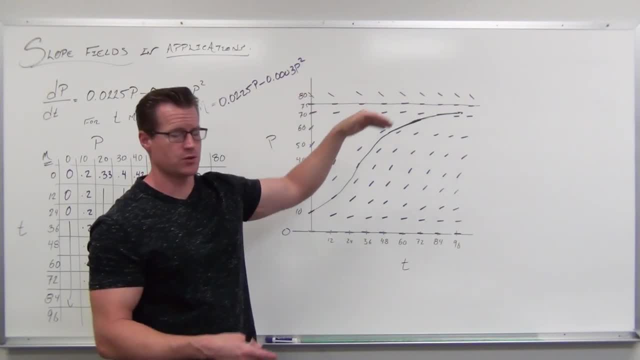 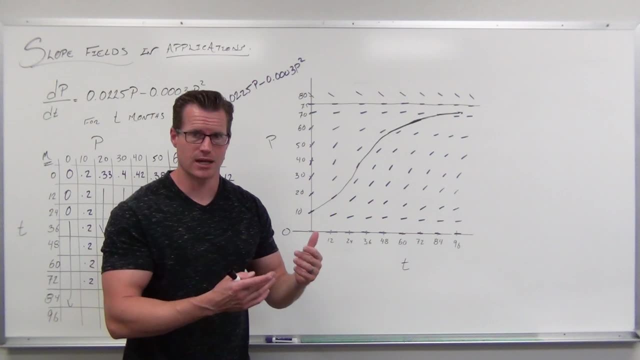 So if you start with a population of 75, you ain't going to grow. If you jump out of the helicopter at 20 feet per second, you're not going to fall any faster. So they tell us a lot. They tell us a lot about a situation just by looking at it. 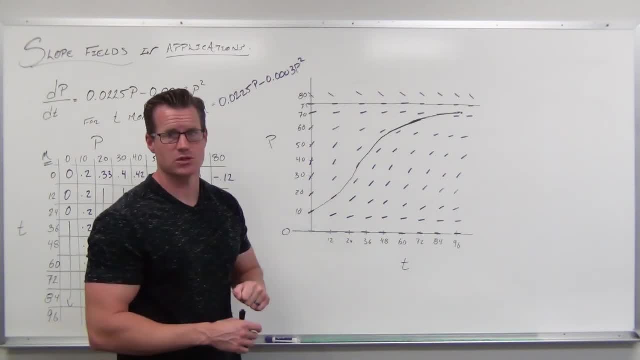 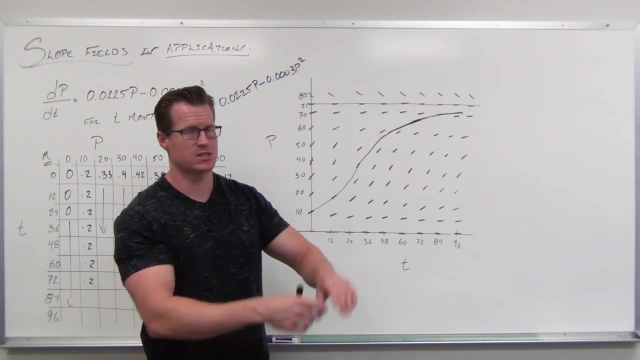 To get a specific curve, you need a starting point. So you need to say: I'm going through this point and then you can find a particular solution. That's how all initial conditions work. anyway. Initial condition gives us a particular solution. 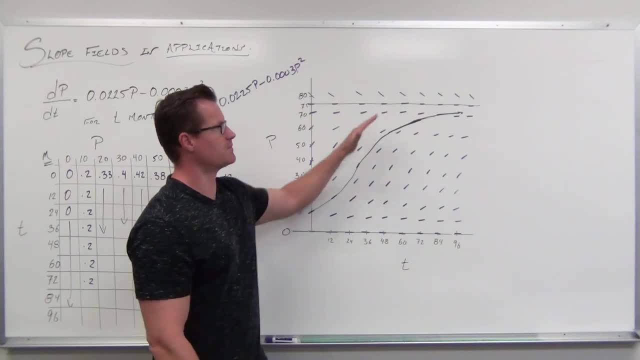 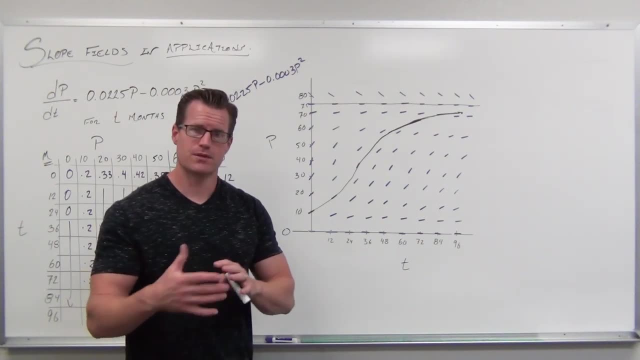 A lot of times we can see what are our trends in gaining or losing and how that would really affect our real life situation. So I'm hopeful that this is making sense to you. I'm hoping that you see the niceness of it. I'm hoping that you see the niceness of it. 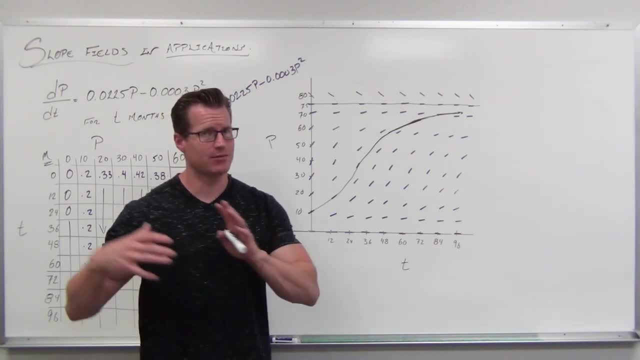 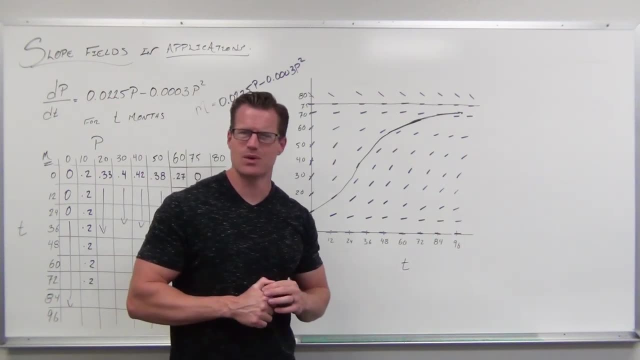 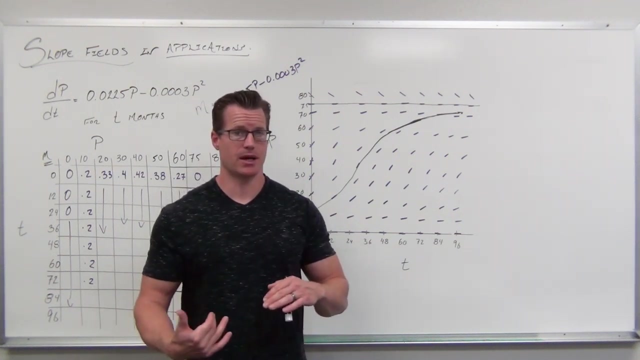 I'm hoping that you see the niceness of it. I'm hoping that you see the niceness about this: that you can approximate solutions without actually having to do anything with the problem. That's pretty cool. Computers do this really well, And what's nice about it is remember that whole talk about how we have this tradeoff between perfectly modeling the situation and doing the math behind it. 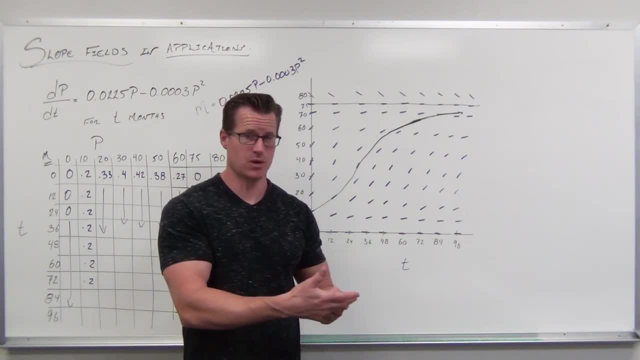 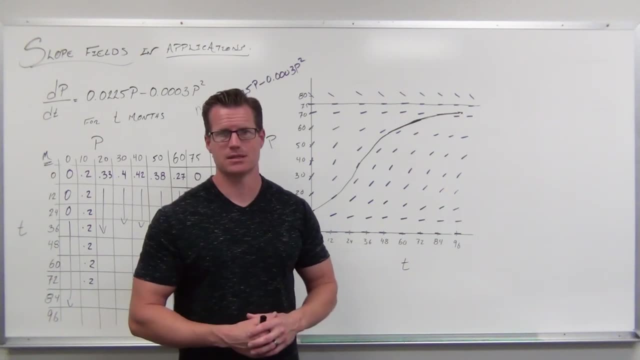 Well, if you've got computers, you can kind of do both. You can perfectly model a situation and then do a slope field And it will show you a lot of trends in it. It will show you limiting capacities Or limiting, It will show you limiting factors or carrying capacities or limiting velocities and include more variables, even though you're not able to solve it. 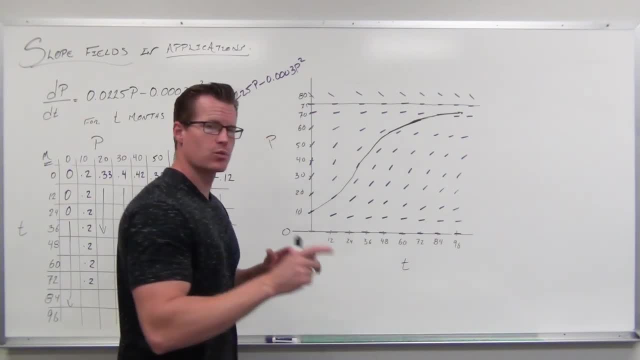 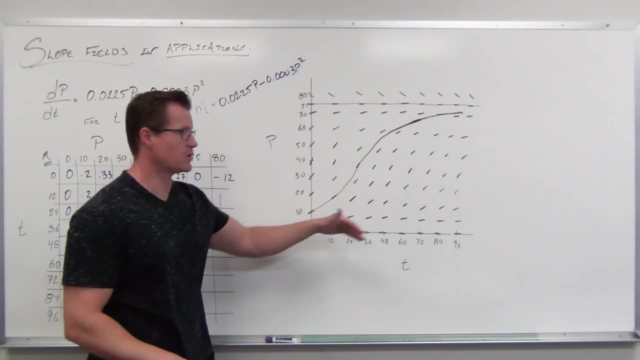 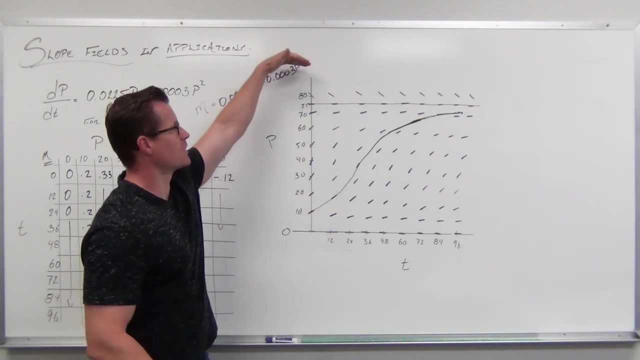 And that's pretty neat. So I hope this makes sense. I hope that right now you're able to take a slope from a differential equation. make up a table, get yourself a slope field and interpret what's going on. Look at how slowly we go if we start low or how quickly we decline if we start high. And think about how that would make sense. It makes sense in real life that with low populations we grow slowly, But as we get more and more population we start limiting ourselves because of resources to a point where we're going to level off Just enough resources to support us but not grow anymore. 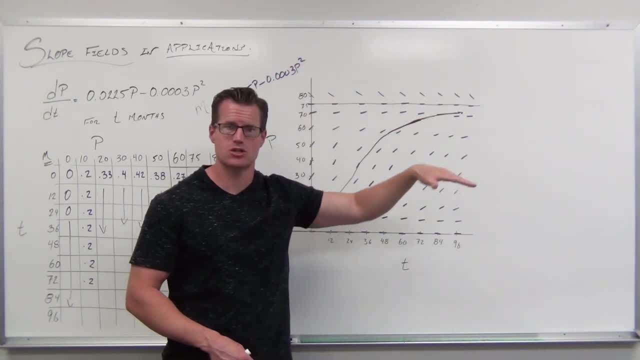 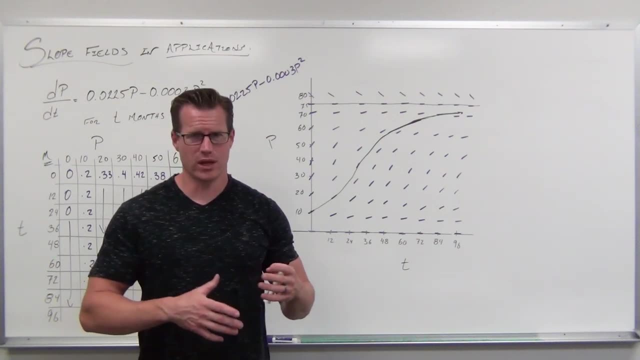 If we start too high, there's not enough resources to support and we would decline population. That's what slope field is about: is interpreting real life situations. So next time, what we're going to talk about is how to determine when we're going to have solutions or not. 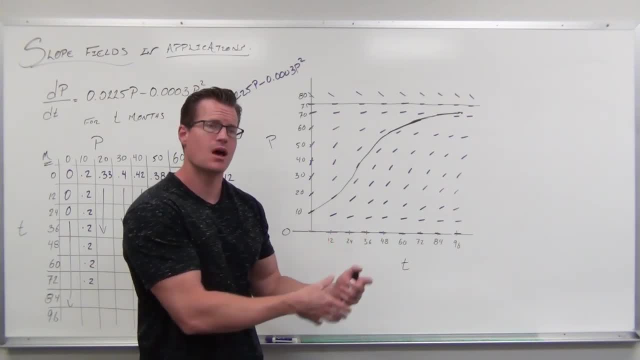 So slope field is one way to do it. So slope field is one way to do it. So slope field is one way to do it. So slope field is one way to deal with it when we don't have a solution. But now we're going to start determining when we do have solutions and when we can expect a unique one. 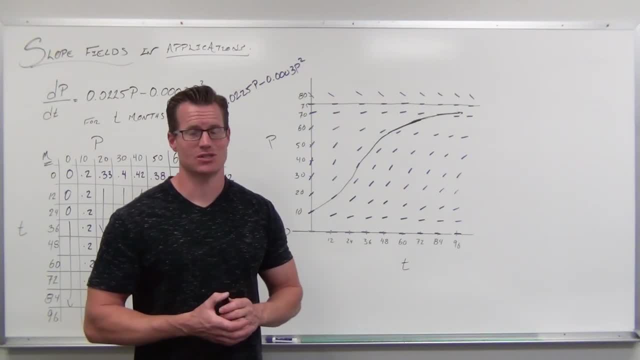 So we'll talk about that, and then, after that, we start dealing with solving techniques, which is going to be fun.